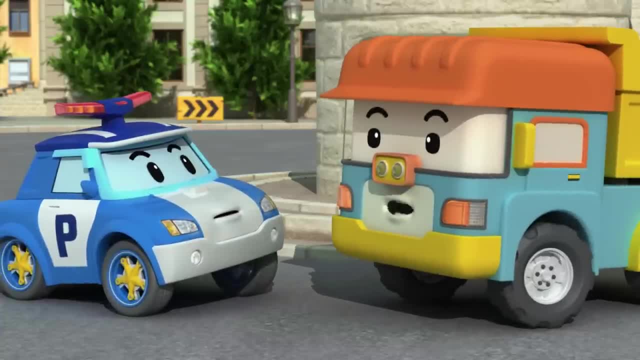 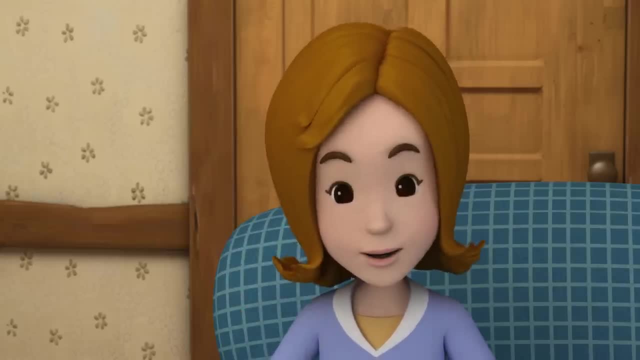 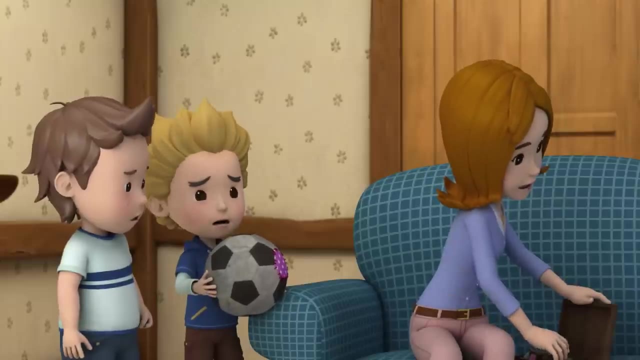 Hmm, I think I have an idea. Great, What is it? I don't see it There. Good as new. Oh, This looks awful. Sorry, next time you should be more careful. Learn from your mistake. Don't play with it near the road. 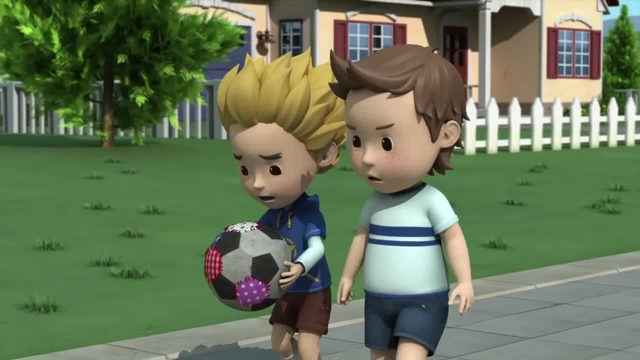 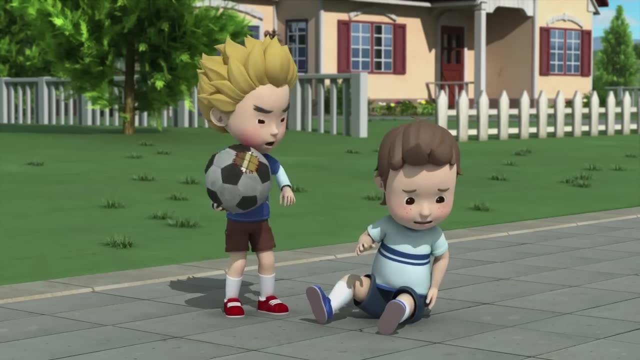 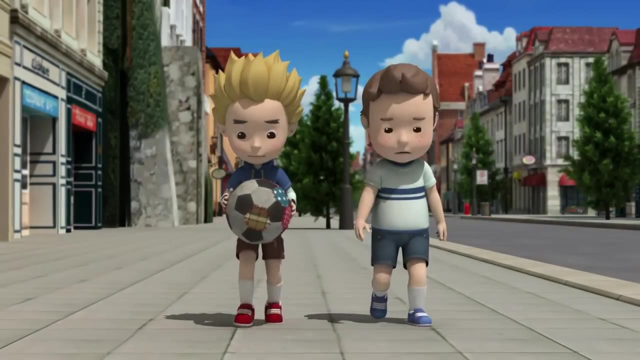 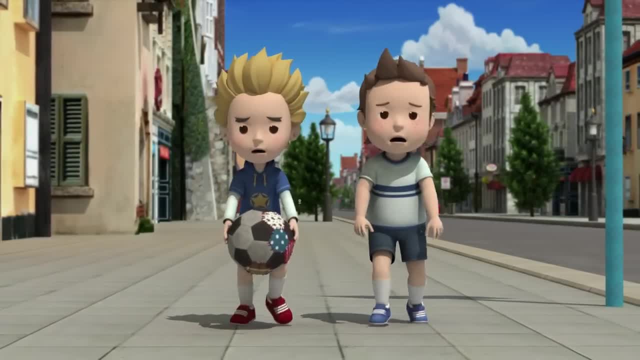 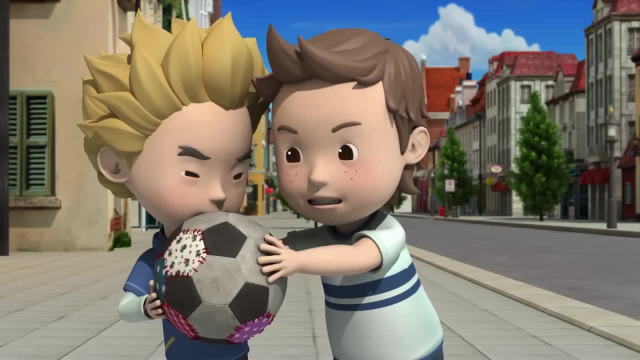 Here, Here, Here, Here, Here, Here, Here. Ugh, It's so boring just holding the ball. Give it to me, I'll carry it. No, it's mine, I'll do it. Let me, I will. 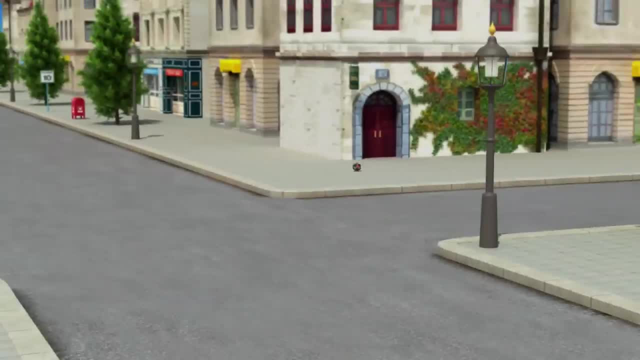 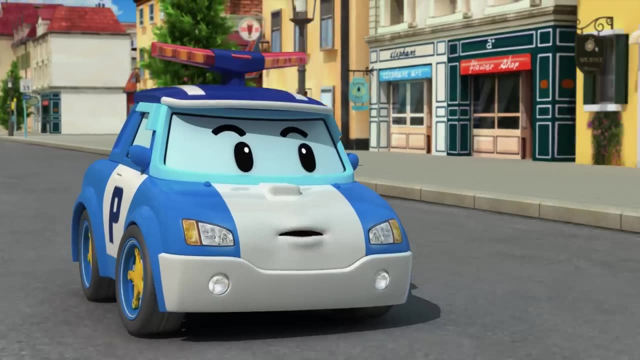 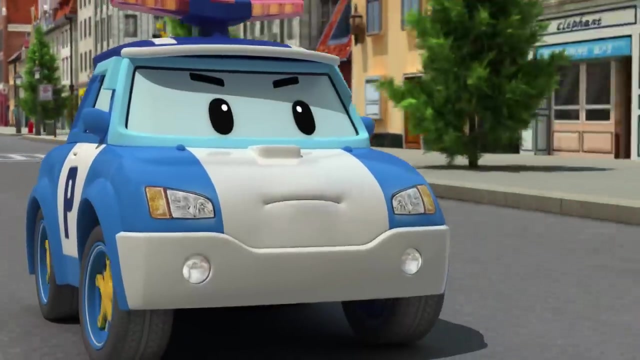 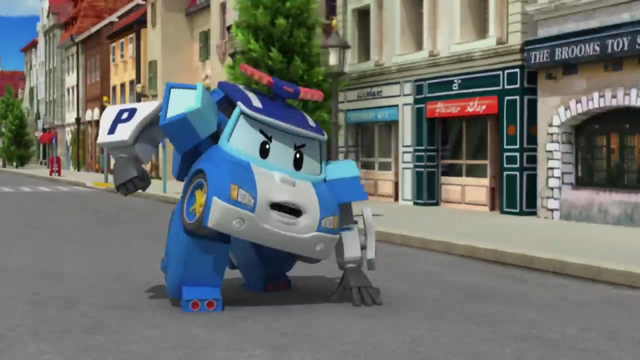 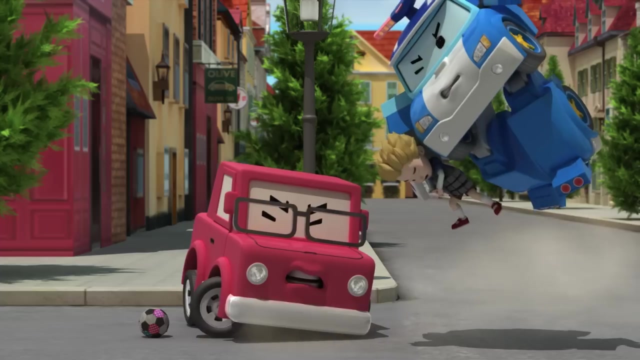 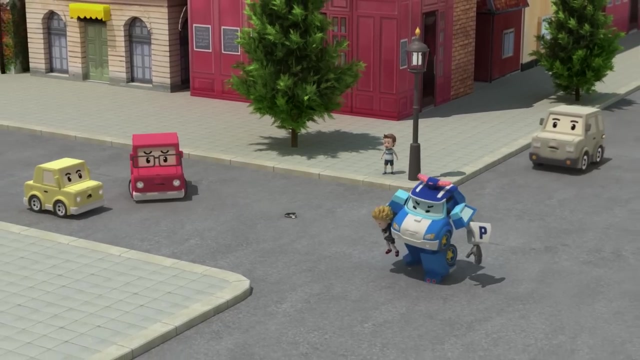 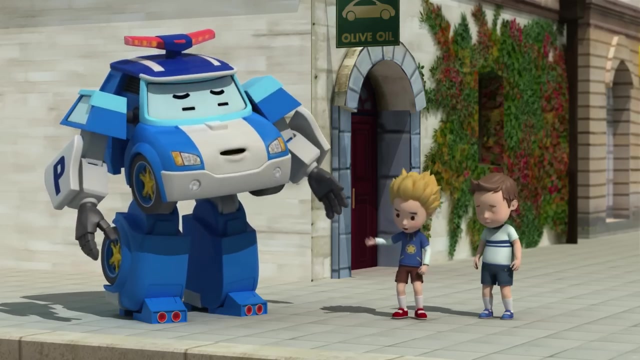 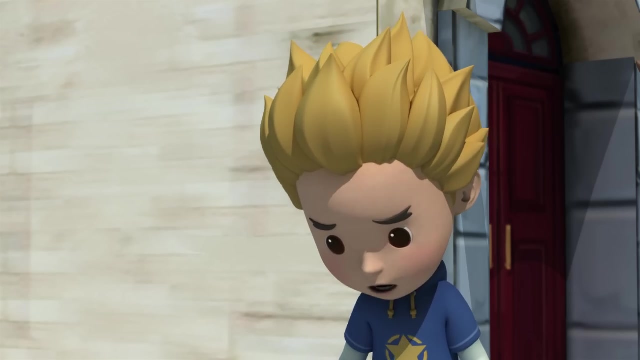 Get it. Come on, I'll No, Kevin and Doug must have gone home. Oh, Kevin, stay there. Oh, Kevin, are you okay? Yeah, Thanks a lot, holy Kevin. Doug, This is your second near accident so far today, I know, but I really tried to hold on to the ball this time, Polly Kevin. 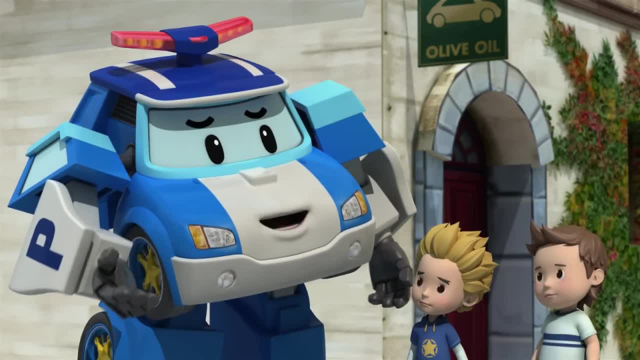 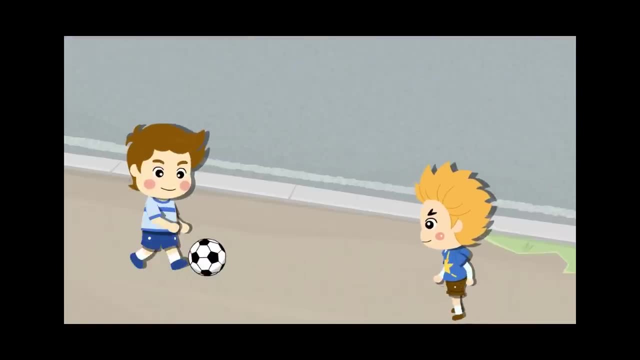 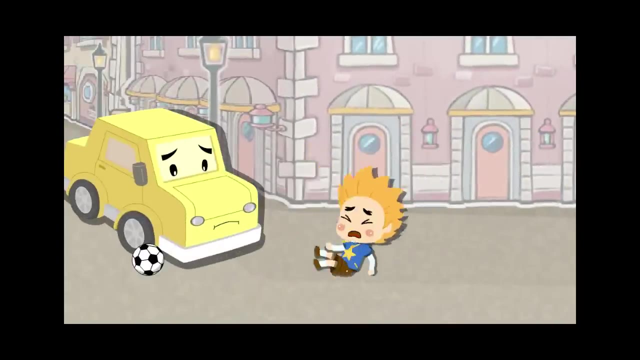 You can always get another ball, but you can't get another life. Yeah, can you remember a few simple rules for when you play ball? sure, Don't play ball where there are cars nearby. play in the park. When you're focused on the ball, you might not realize when a car's coming, and that's dangerous if the ball goes out into the road. 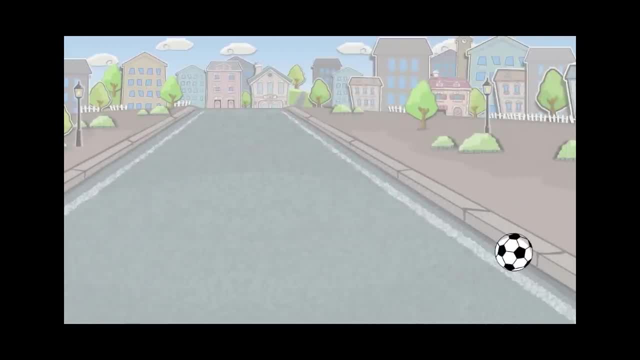 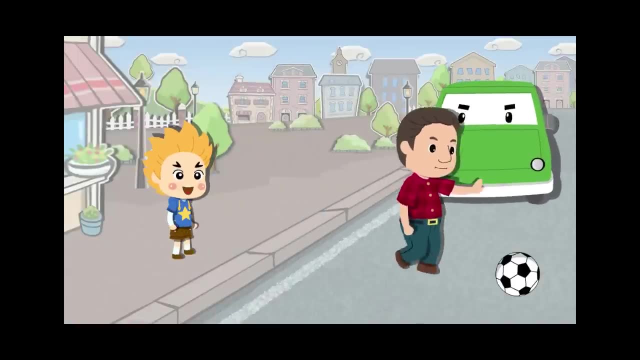 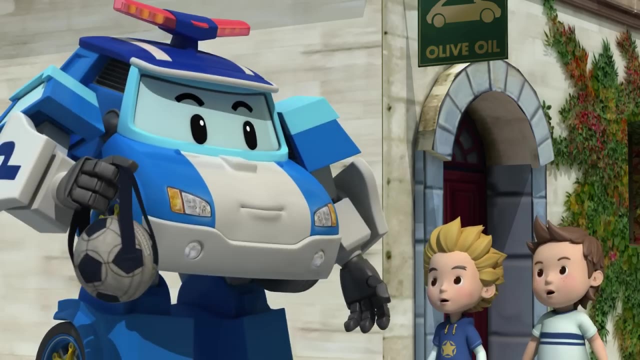 never run out after. Just wait until the ball comes to a stop, cross safely and then pick it up, Or ask an adult to get the ball for you. okay, Polly, and now tada. What's that? Polly, It's a ball bag. you carry your soccer ball in this and you don't have to worry about it rolling away. 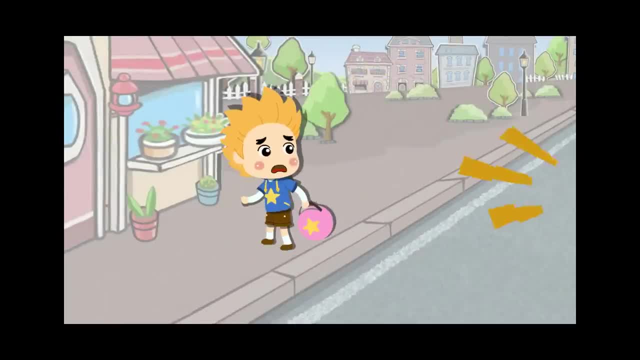 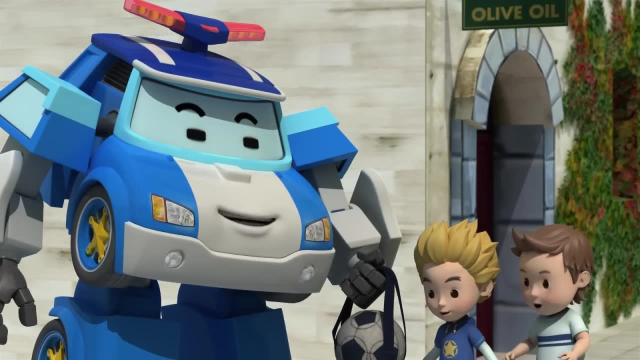 When you carry a ball in your arms, There's always a chance that can get you into danger. when you don't have a ball bag, use a plastic bag instead. Here, Kevin, This is for you. Thanks, Hey, Doug. Whoa, a new ball too. 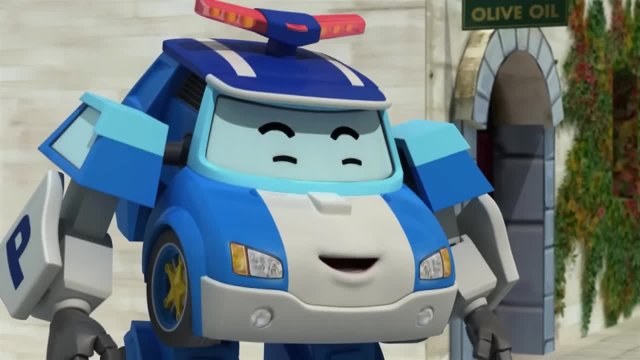 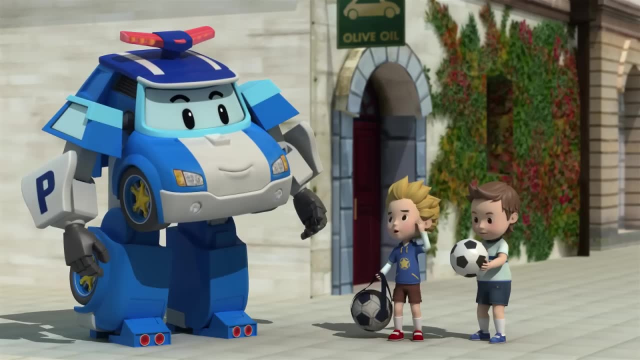 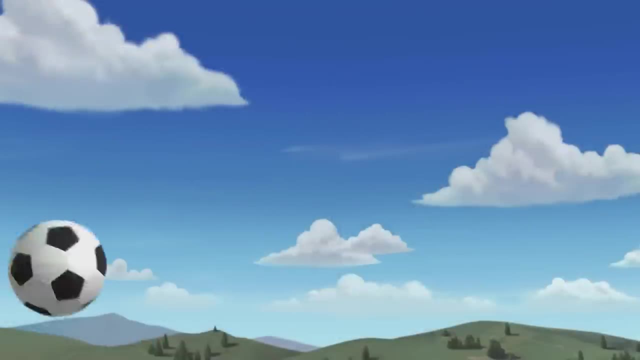 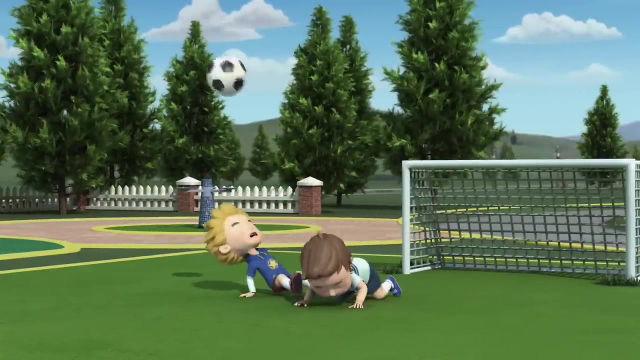 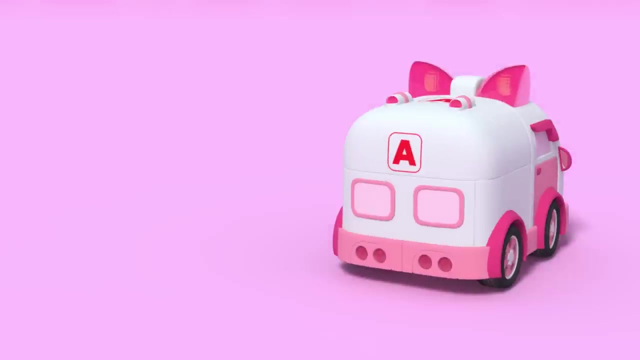 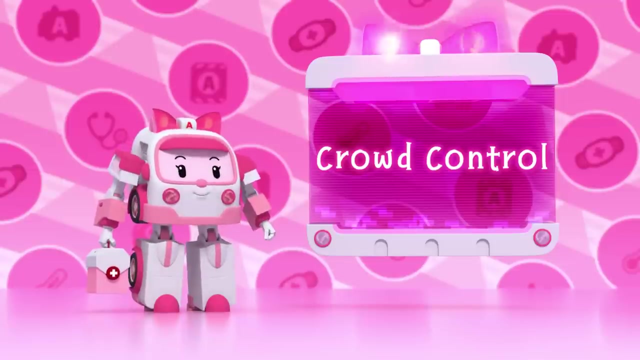 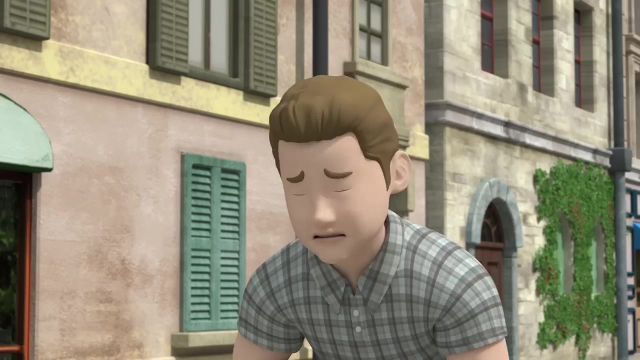 Wow, Thank you Polly. Well, actually the balls from dump the truck, He said to say that he was sorry about running over your ball. Wow, that's nice. Yeah, Here we go. You better catch it. Whoa, Hey, Crowd control. Lucy, hold my hand for safety. 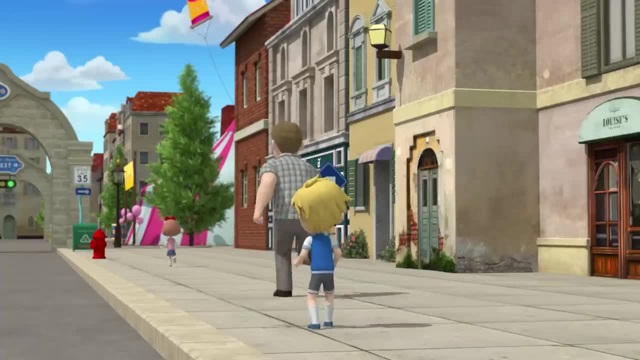 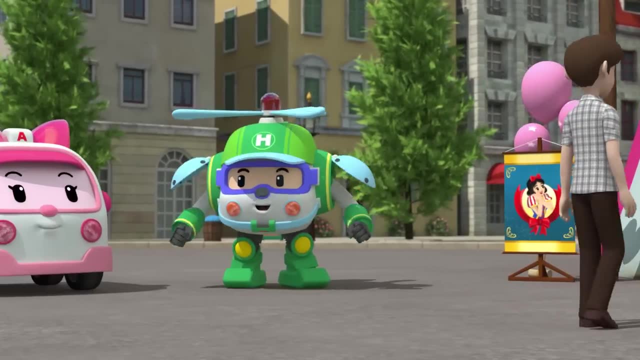 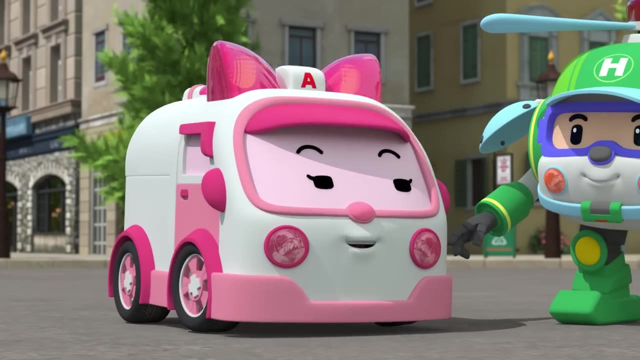 But we're gonna be late for the show. Wait, Lucy, Come on, can we slow down? Wow, There's a lot of people coming to see the Snow White play right now. Holly, let's be sure to keep a lookout. There's a lot of people in one place, So I don't want anyone to get lost. 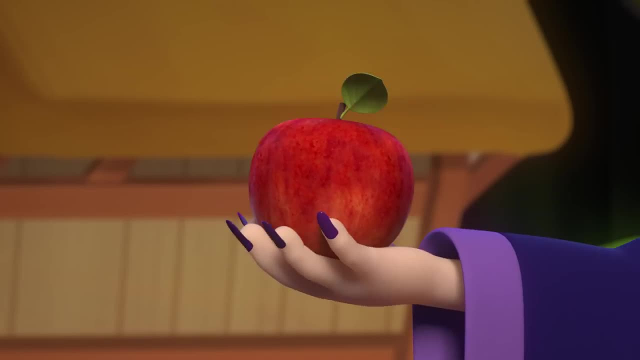 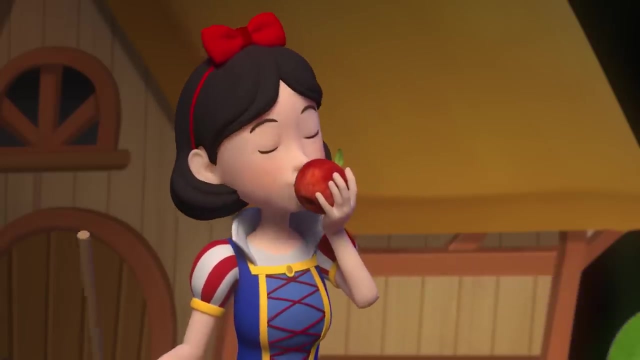 It sounds good to me. Hello, fair princess, I brought you this fresh apple. Would you please take a bite? Oh my, How very kind. Oh, no, Don't eat the apple, Daddy. don't let her eat it, No, Lucy. 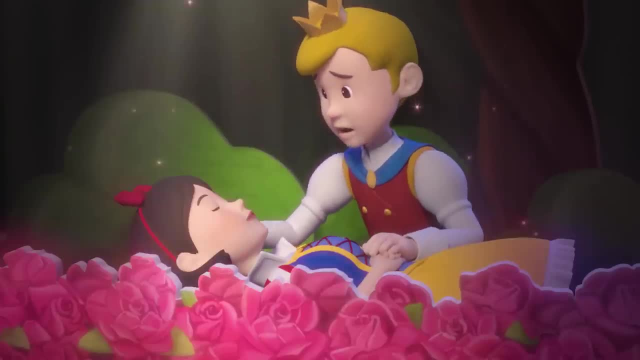 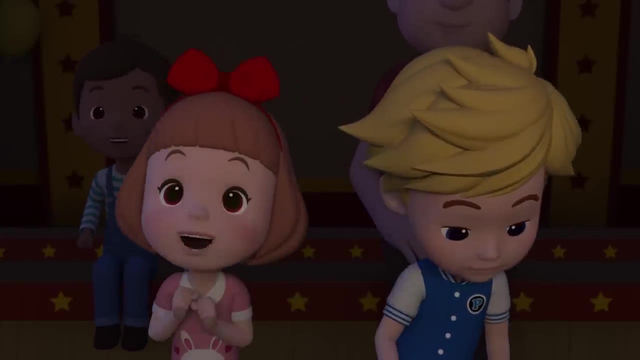 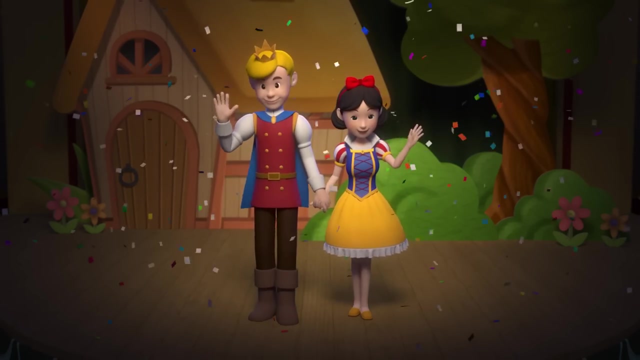 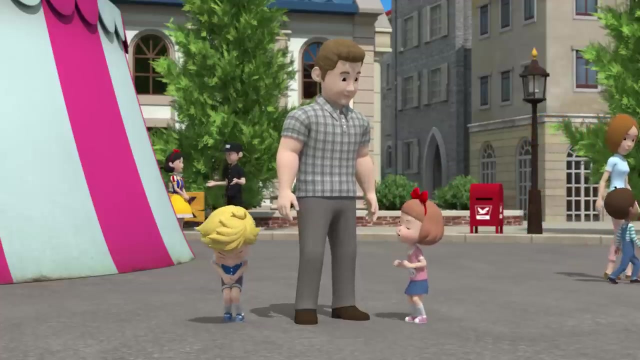 Lucy, It's a play, My love. open your eyes, Look, Look, You're happily over after. Is it over yet? Thank you, It was fun addling the bunch, Yay, Ah, wonderful job, Dad. that was super extra fun. We should bring your mom next time, OK. 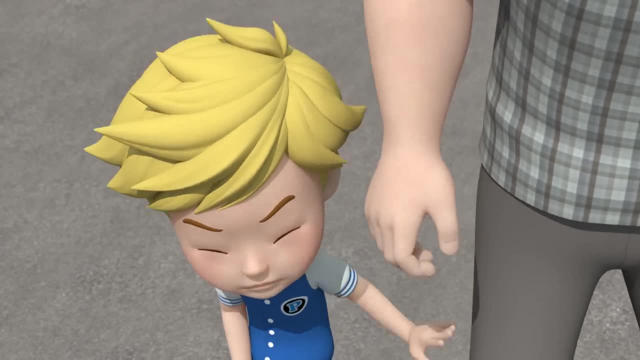 Yeah, Uh, oh, Dad, C'mon, C'mon. No, don't forget your завar. Ought to bring your mom next time. Ok, I gotta go. Really really bad Right now. Uh, over there, Let's all go. 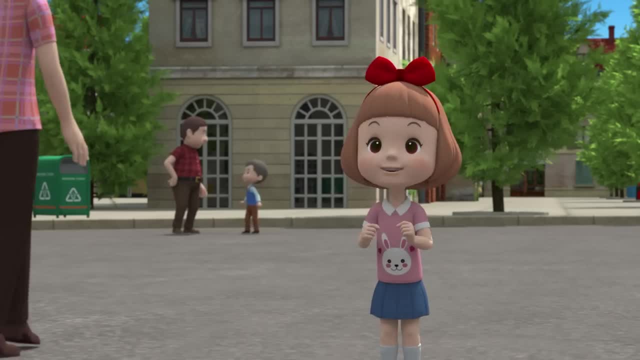 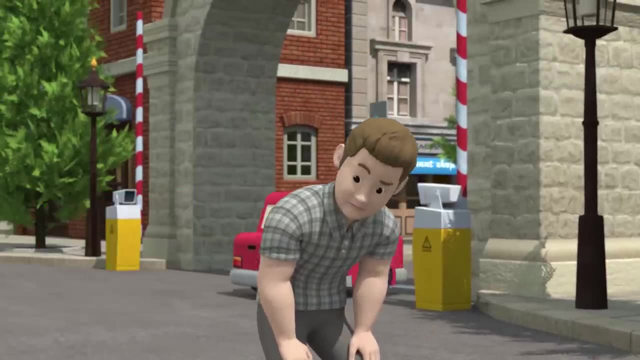 I mean, if you are, It's the princess of real life, Snow White. Oh no, Lucy, don't tell me you have to go too. Huh, Lucy, Lucy, Tomorrow's just the matinee, Thank goodness. 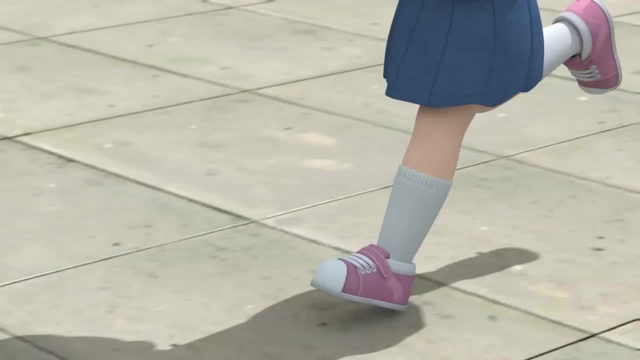 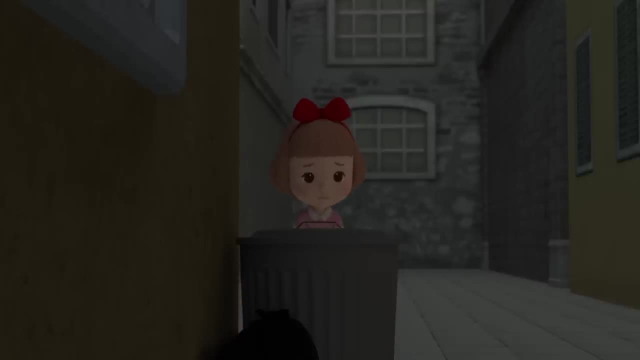 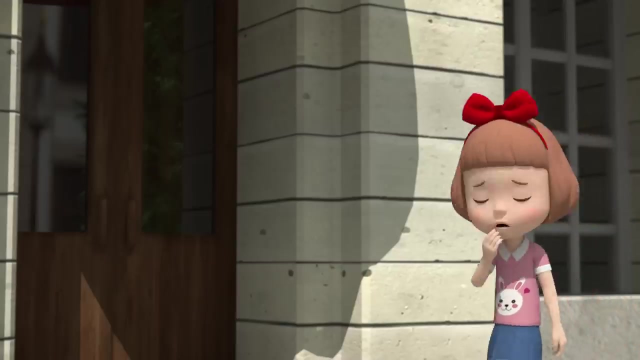 Princess, Snow White, Snow White, Oh Snow White. Oh Well, where could the princess have gone? And where did my dad go? Did I go too far? Oh, That's where the play is. I'll go that way. 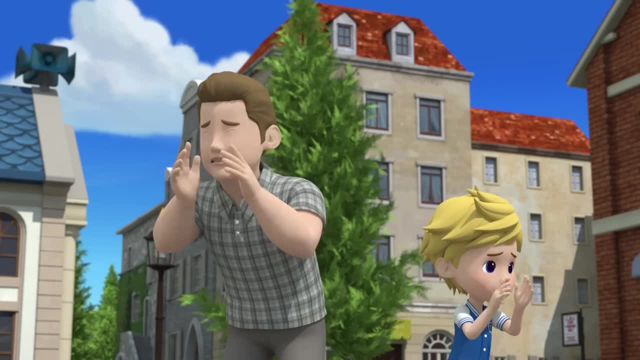 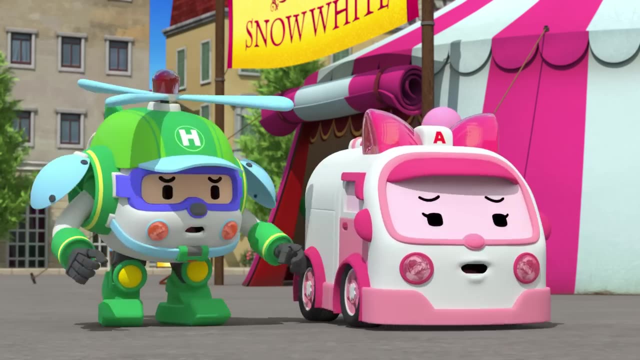 I'm so smart, Lucy. Lucy Is something wrong Afraid. so My daughter Lucy's gone. What Lucy's lost, It's my fault. this is happening. Just stay calm, I know. I know We'll be able to find her. 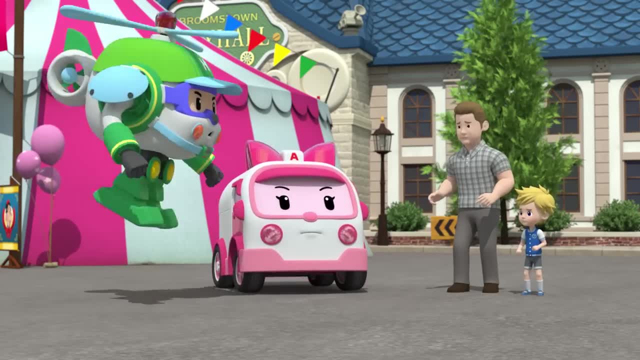 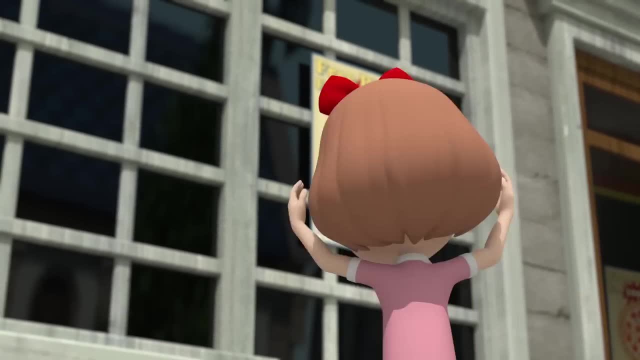 We should check places nearby. Got it, I'm Snow White. Here I go Socks so clean as white as snow. Oh, I'm hungry. Oh, All right, That was good. Huh, Hi, little cat, Do you want a treat? 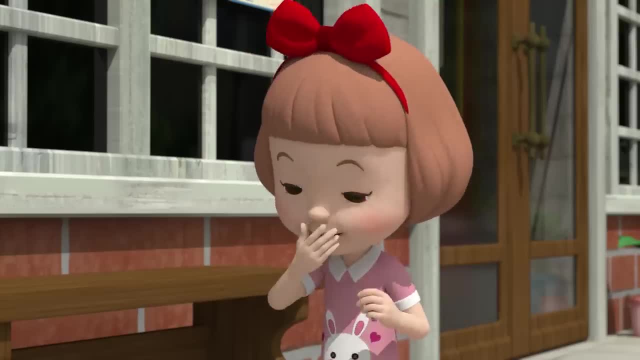 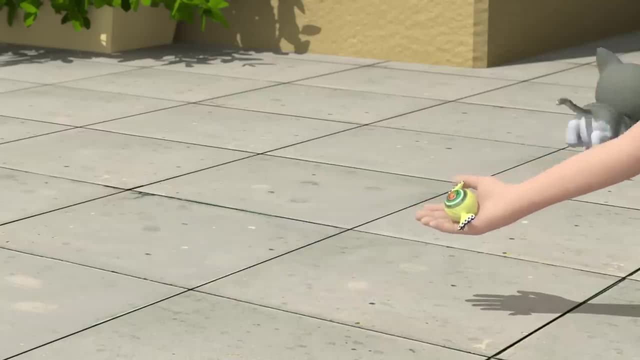 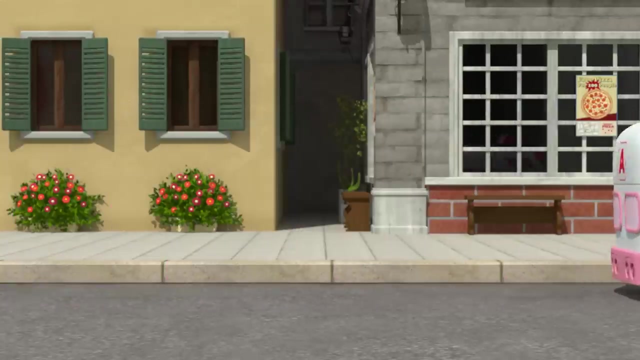 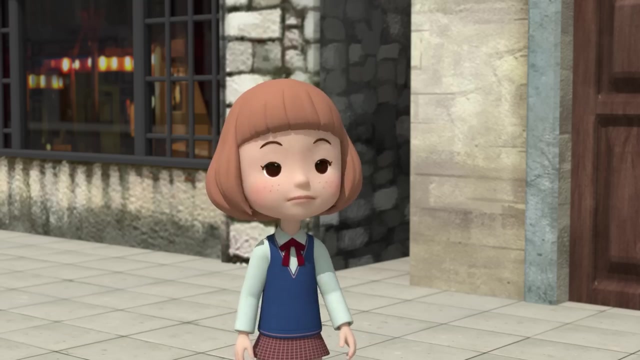 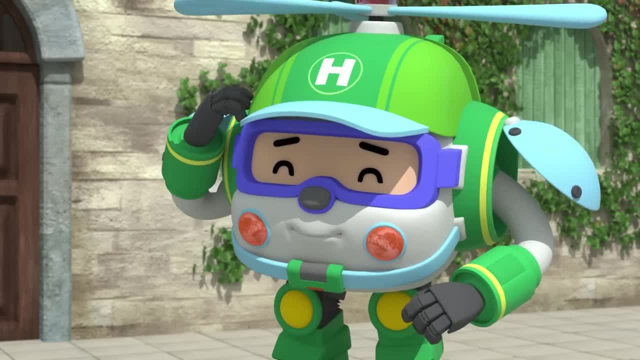 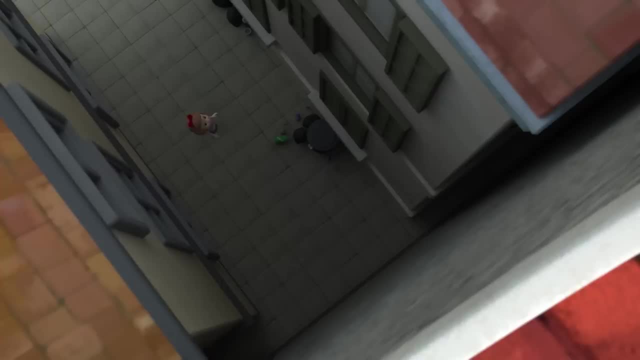 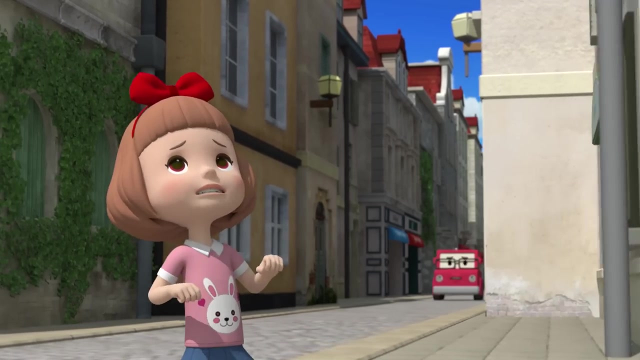 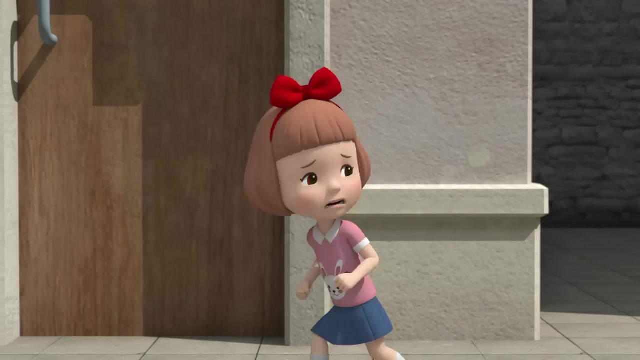 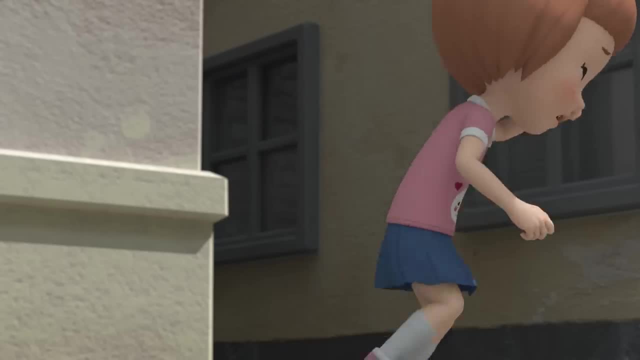 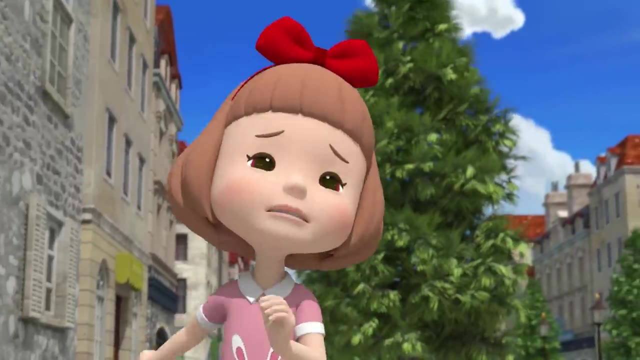 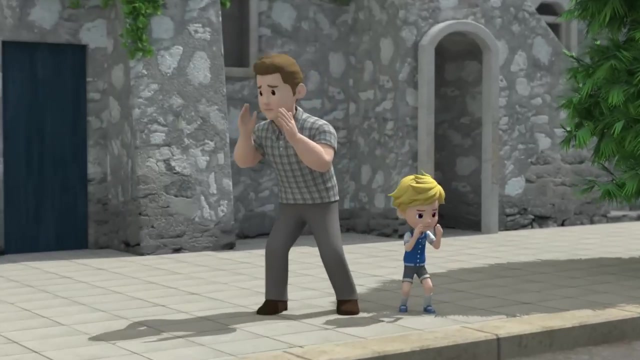 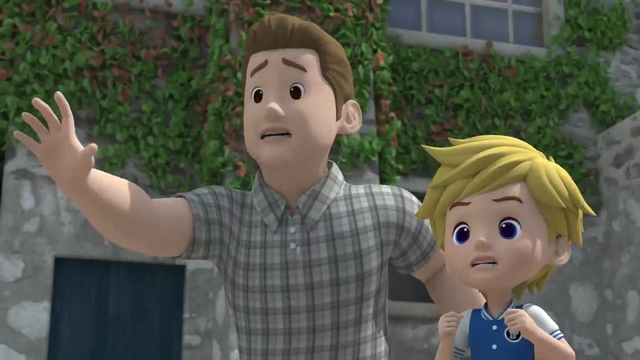 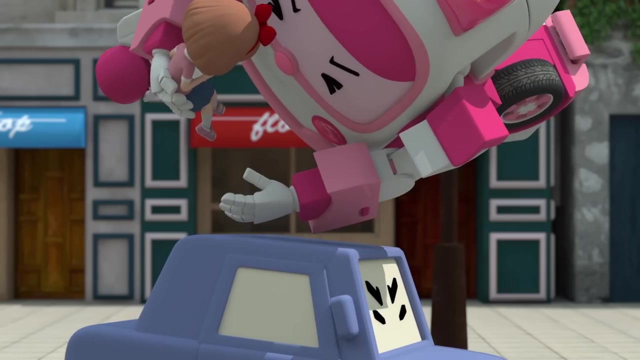 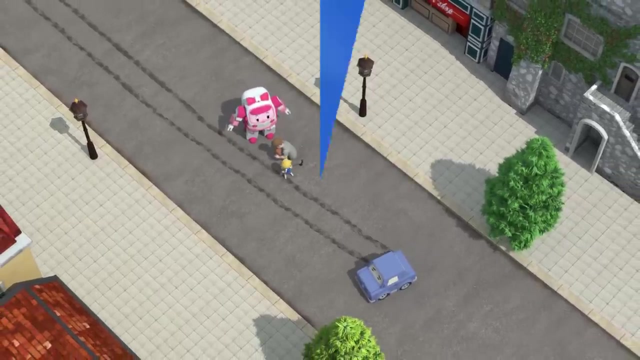 You could get hurt. Sorry about your box, Daddy. Where are you? Daddy, Lucy, Lucy, Lucy, It's Dad. I'm over here. Oh, what's wrong, Lucy, Hang on, Daddy, Lucy. Daddy, That was a close one, Lucy. 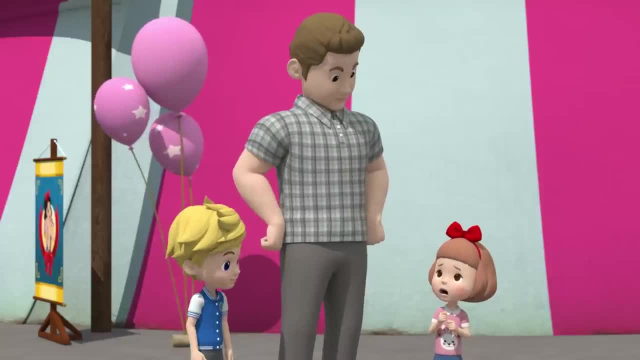 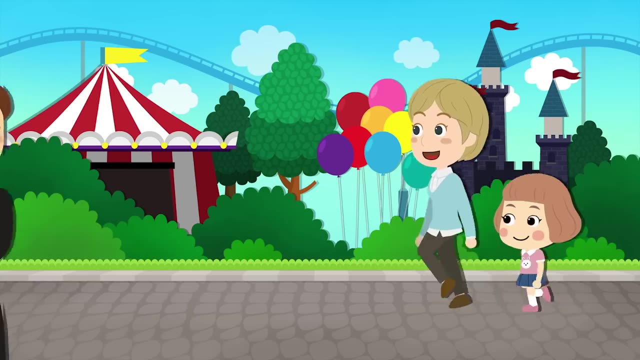 Your dad was worried about you. I'm sorry, Dad. We're just glad that you're safe. If you ever do get lost again, here are some things that might help. In large crowds of people, it's easy to accidentally get separated. 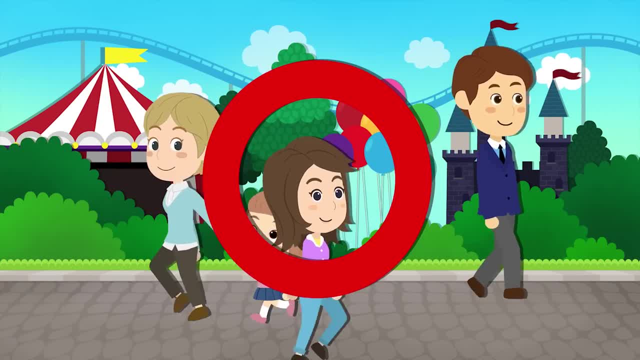 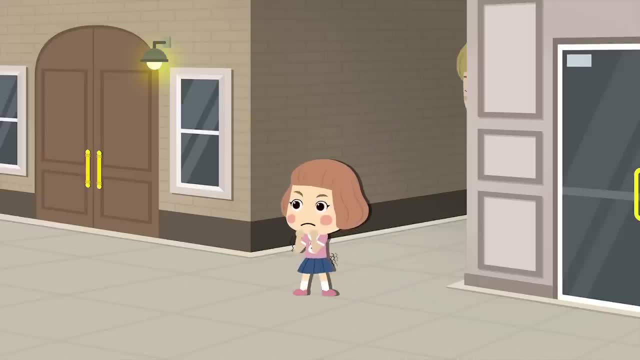 from your parents. Always hold onto your parents' hand. If you do get lost, don't run away quickly. It's better to stop in one place and wait for them to find you. If you see a police station or a fire station. 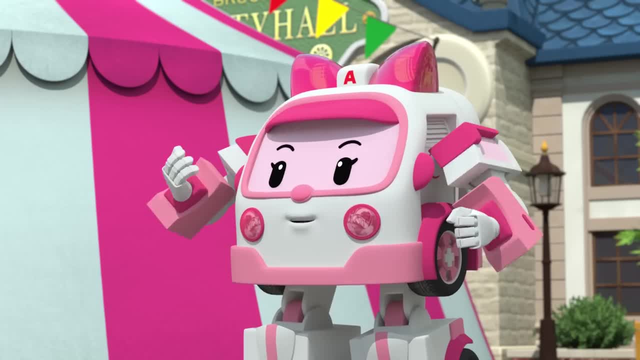 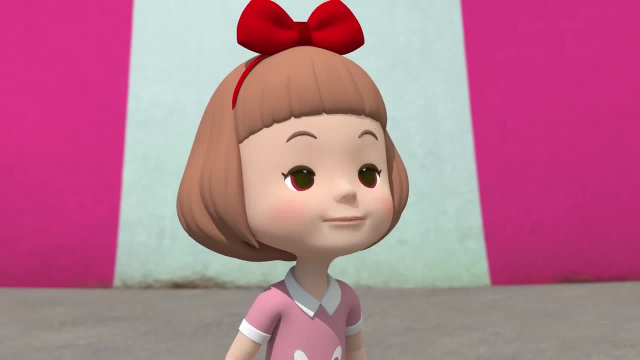 you can ask them to help you. Tell them your name, your parents' names and information, and their phone numbers as well. Got that, Lucy. I know what to do now. It's Snow White- Snow White's here, So cool. 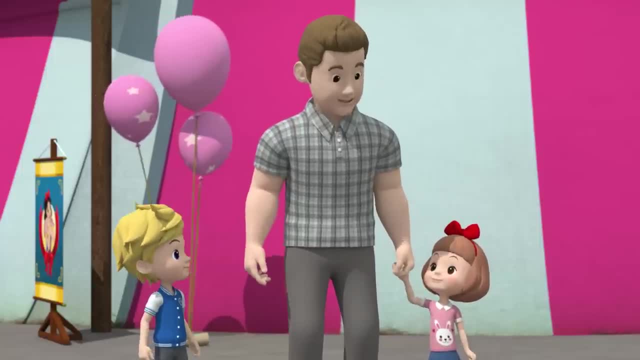 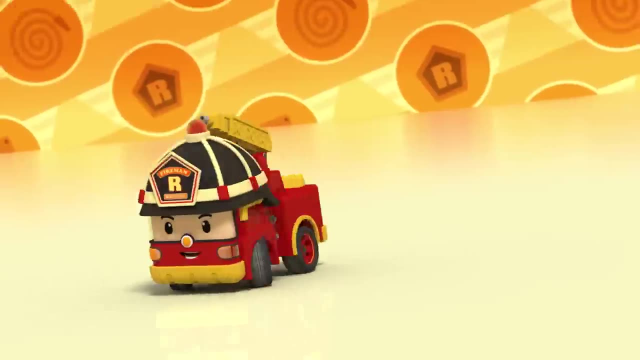 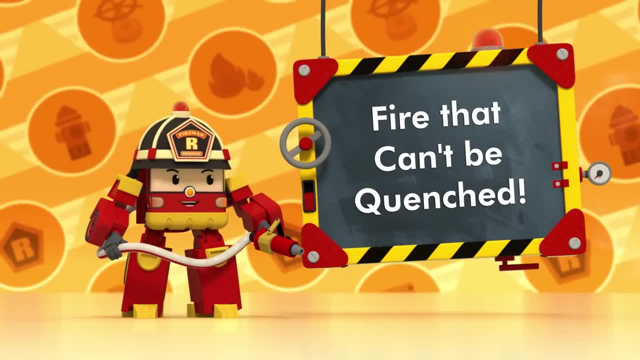 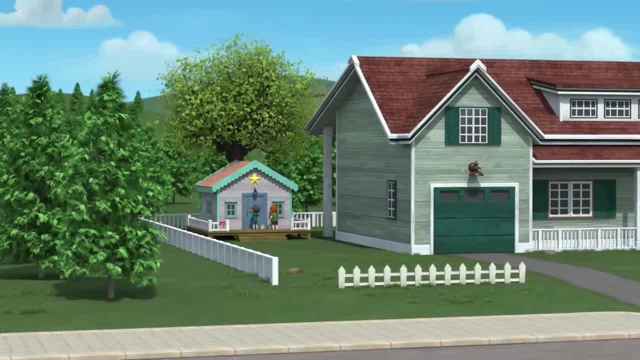 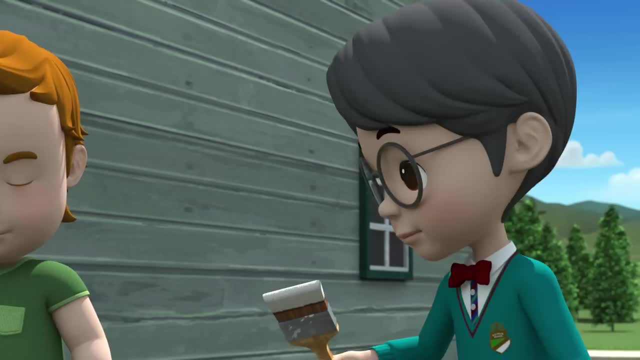 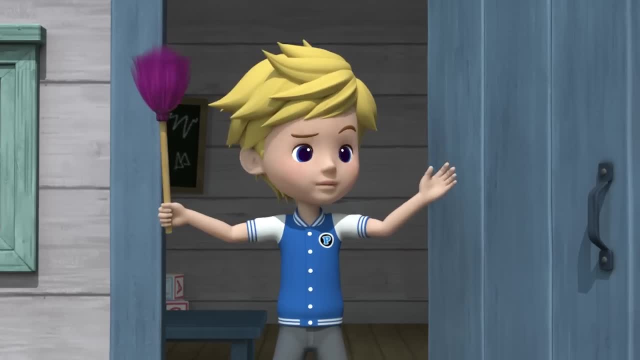 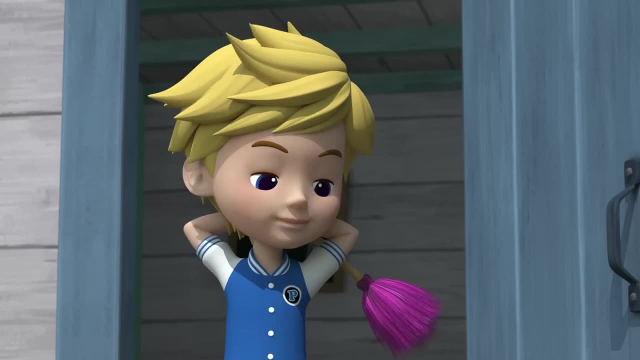 Ha ha, Ha ha ha. It's all clean. Ha ha ha. Oh, What did you do? This is your fault. Yeah, My bad. Anyway, I'm all done cleaning. Come in Yahoo. Ha ha, Hang on. 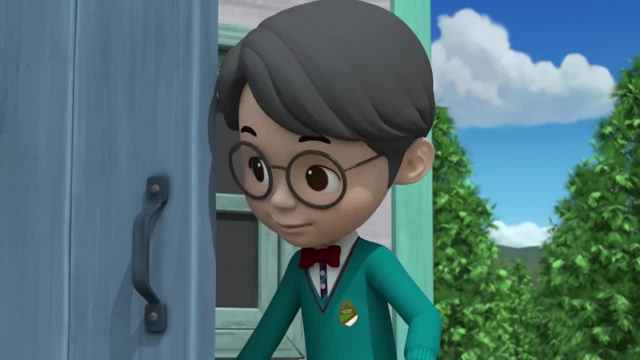 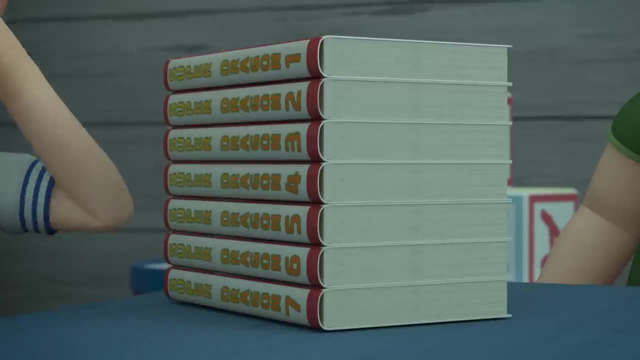 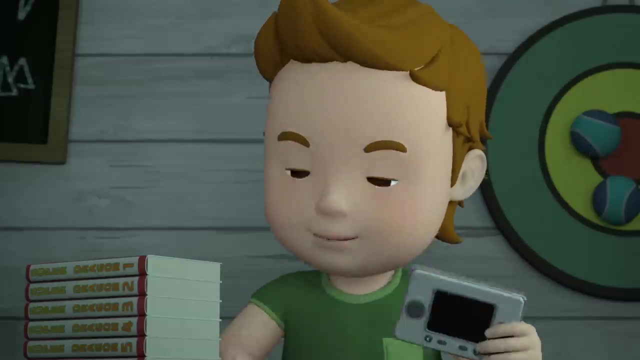 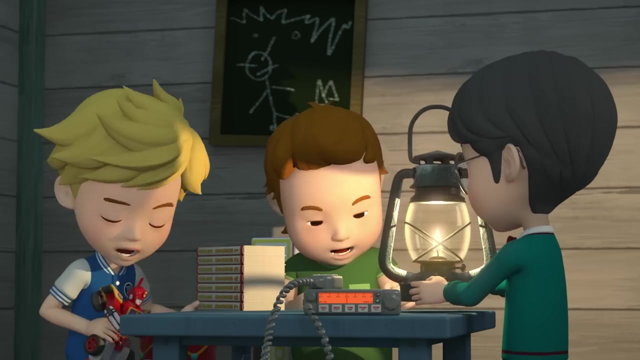 One last thing: Huh, finished, Ta-da, all seven episodes of the newest super dragon series. Hmm, That's cool, But haha, it's only the best. latest ninfrando, Oh, oh, Beware my super dragon fist. Huh, Wow, What's that, Charles? It's called an oil lamp that looks super old and stuff, Yeah. 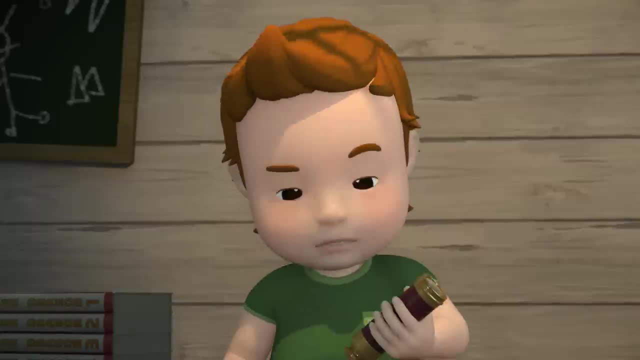 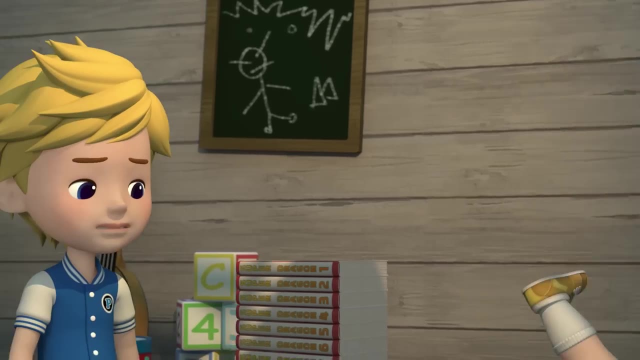 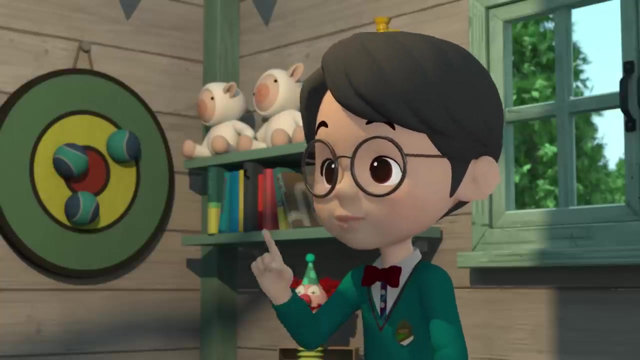 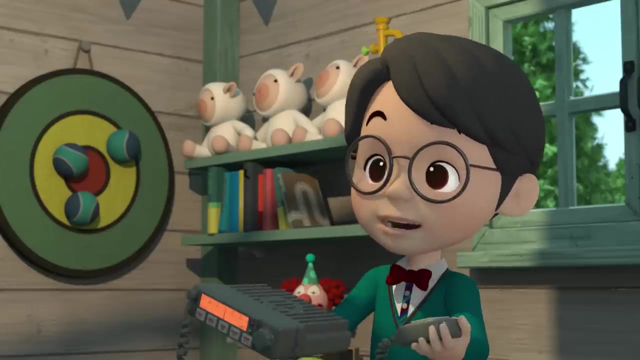 My grandpa used it a long time ago. What's this thing? a telescope? Wow, Wait. what's this? my personal favorite- a ham radio. Yeah, it's great. people use them to communicate all over. You can talk to other people with ham radios all around the world and one day I really hope to hear aliens, aliens. 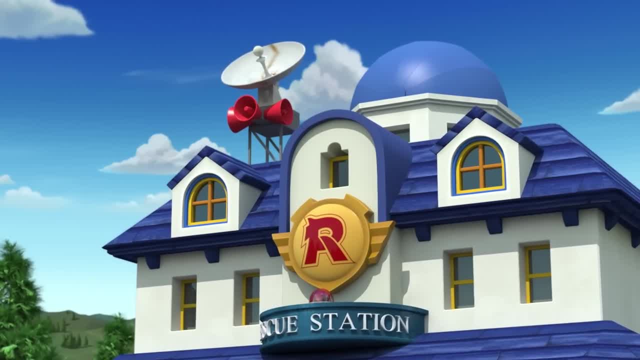 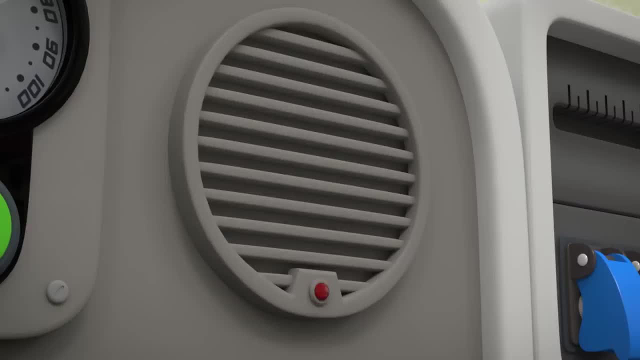 Let's try it out. Hello, aliens, do you hear me? Aliens, this is for the rescue squad. Oh man, It's just the rescue squad. Hey, is that Charles, I hear? sure is, we made a secret clubhouse at Peters place. 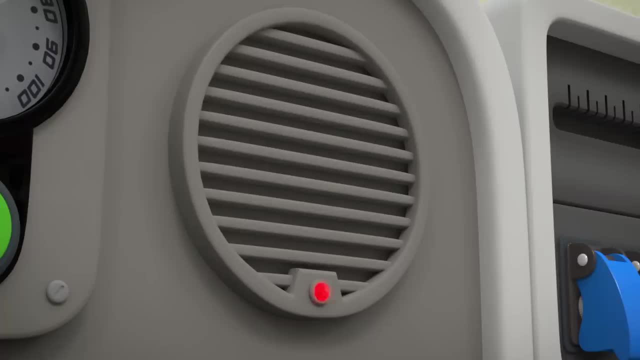 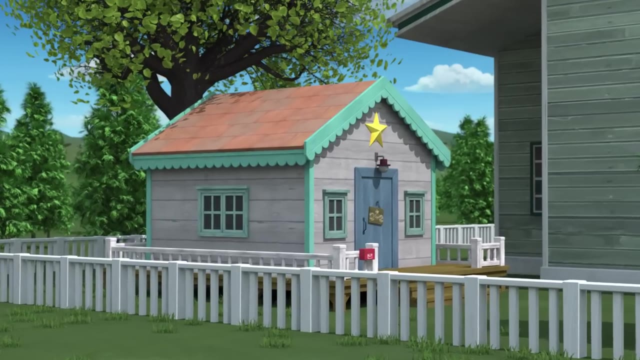 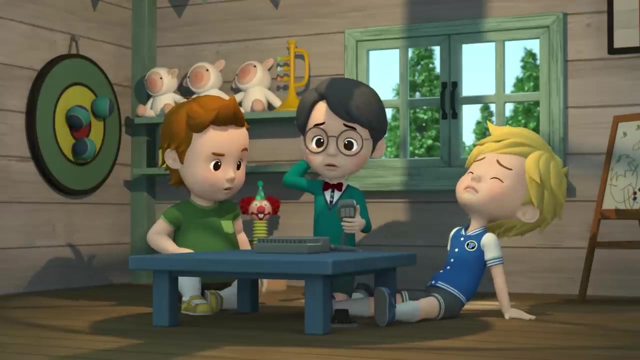 Wow, Clubhouse. Yeah, you guys should come over and say: hi, Sounds good. We can't turn down an invitation like that. Of course, Aliens, do you copy? Hello, Do you copy? Oh man, it's not working. Huh, aliens, that was just me needing food. I'm hungry too. 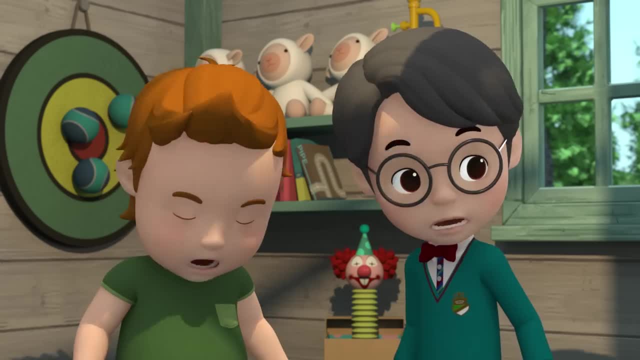 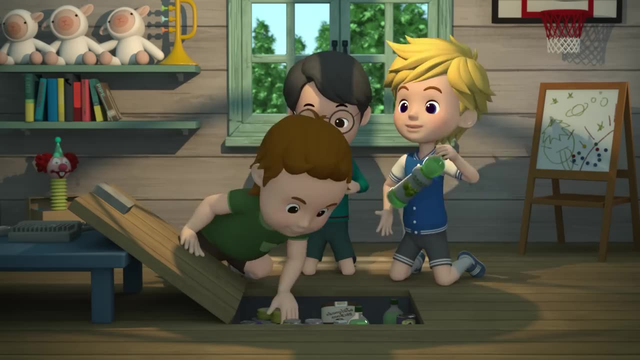 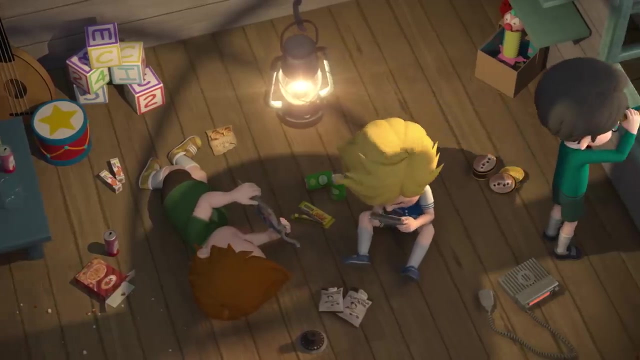 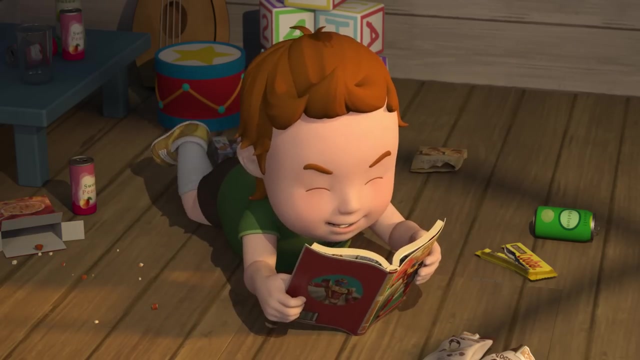 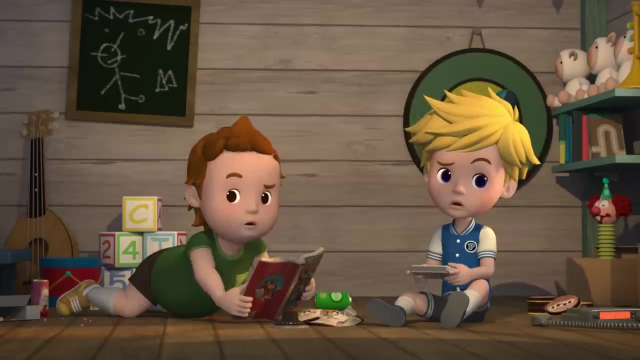 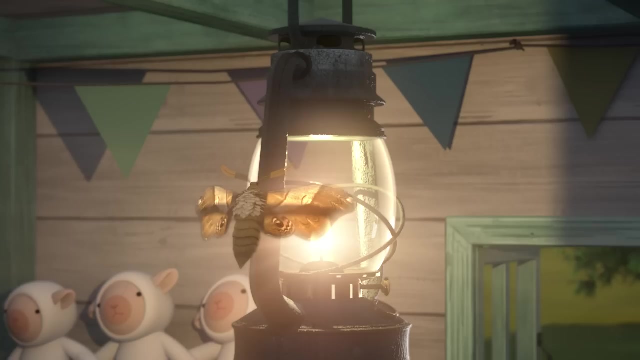 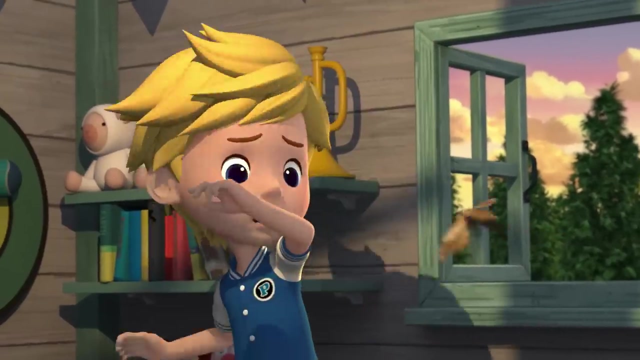 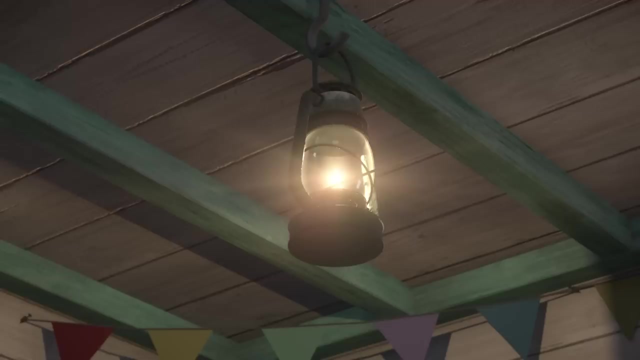 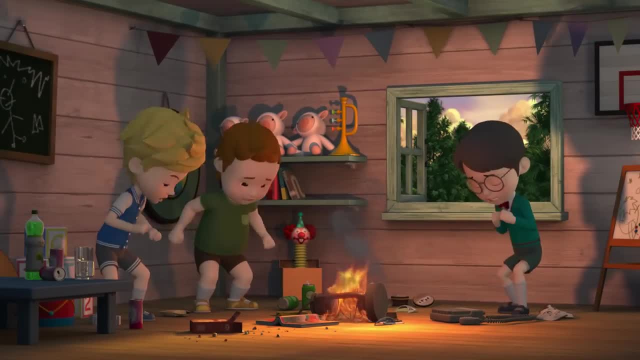 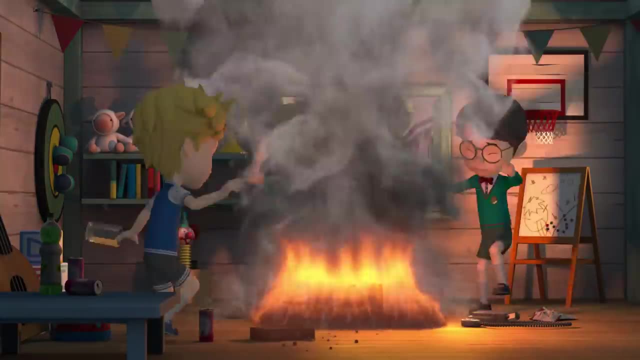 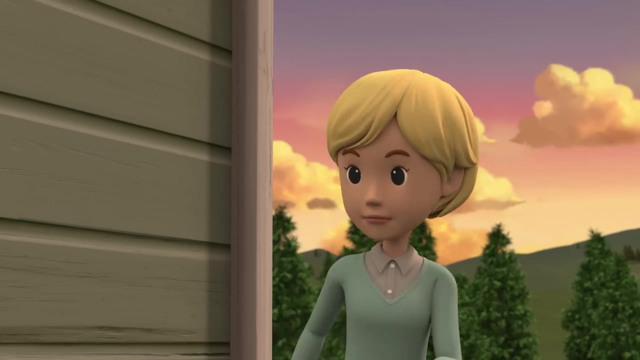 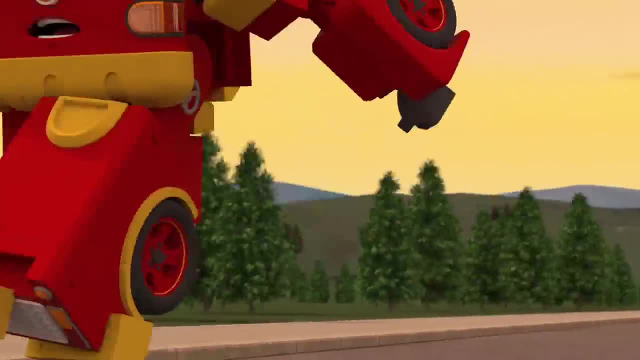 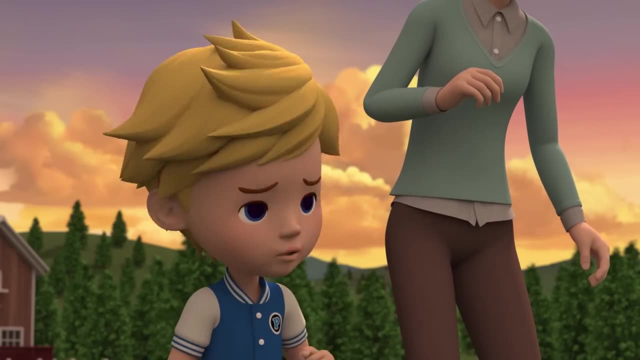 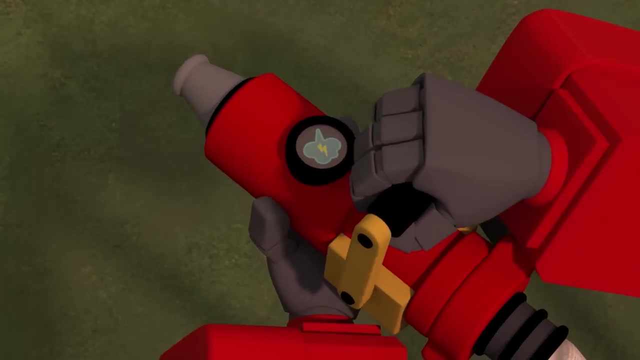 Oh, Ah, Ah, I'm here. What happened, Roy? I tried to put water on the gas lamp, but the fire just got bigger. Is that so I see? Don't worry, Hmph, Hmph, Hmph. 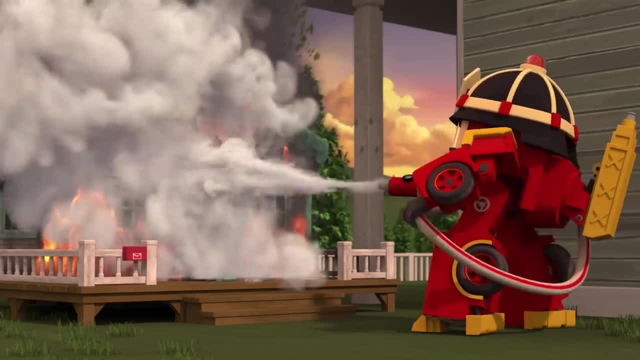 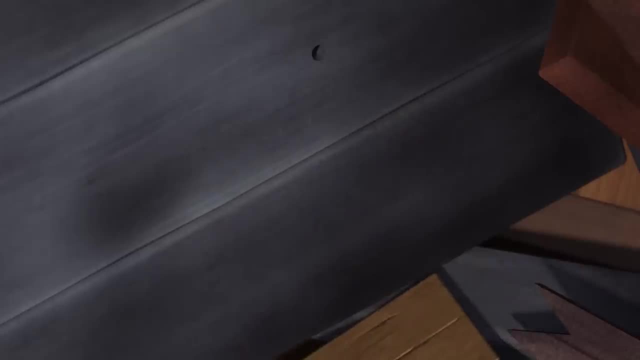 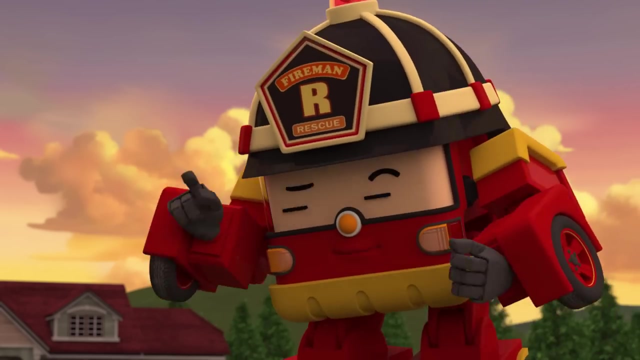 Ah, Ah, Ah, Ah, Ah, Ah Ah. It's great that you're all safe. Listen, if a fire starts from oil, you should never pour water on it. Why Fire from oil can't be put out with water? 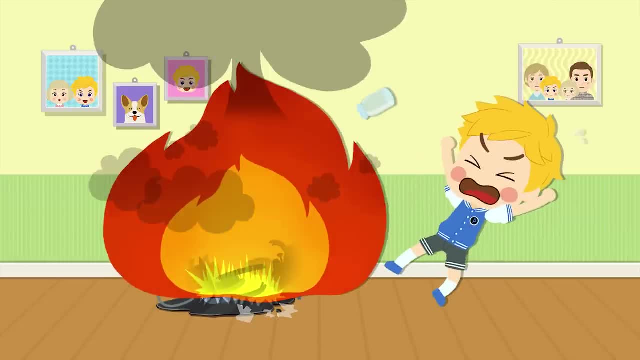 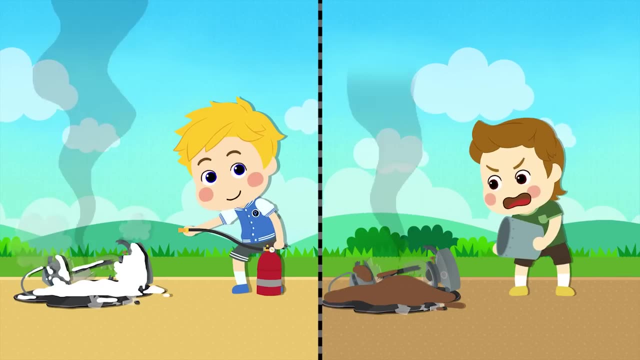 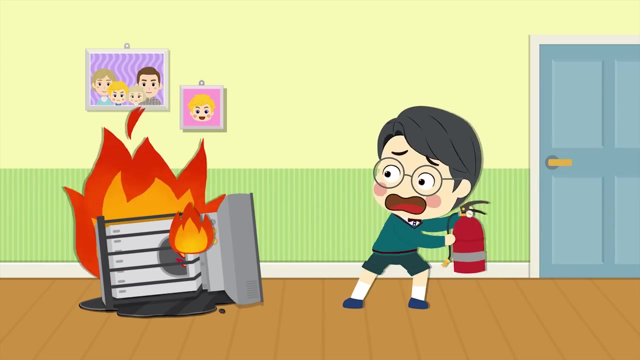 Putting water on burning oil can spread the oil and make it even more dangerous. Instead for grease fires, use a fire extinguisher or sand to put them out safely. These type of fires usually start when we're cooking or using indoor heaters, so always keep an eye out. 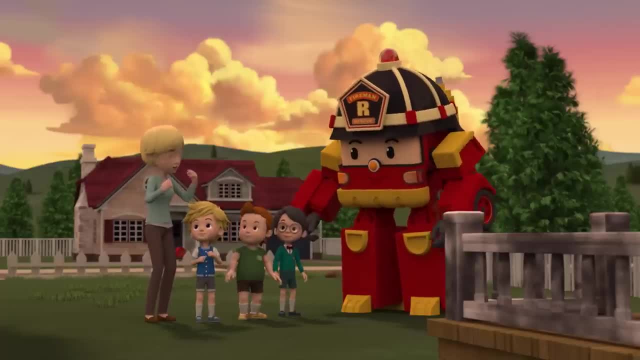 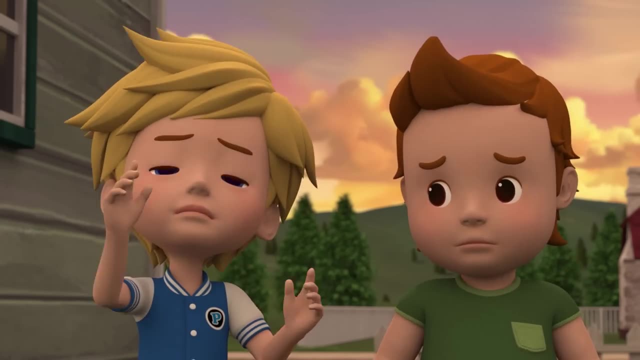 I understand. I'll be careful too. Thank you, Roy. Thanks Roy, We'll be careful. Aw, We put so much work into that clubhouse. I lost my porn-in-friend-o, My ham radio too, Huh. 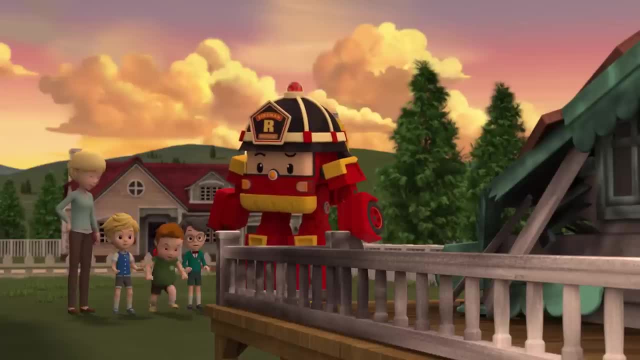 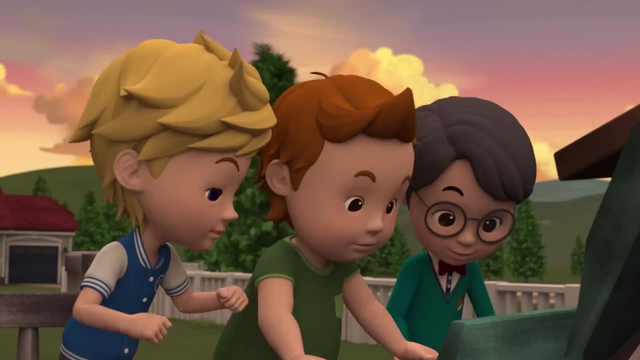 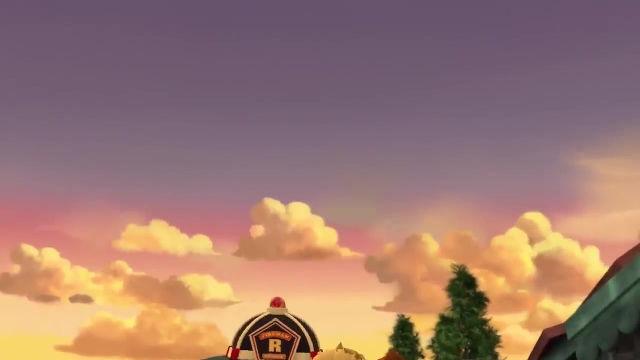 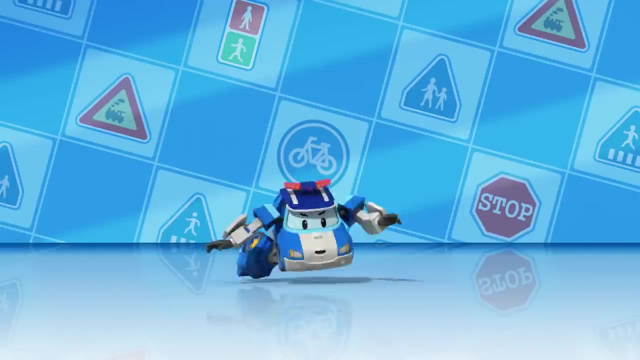 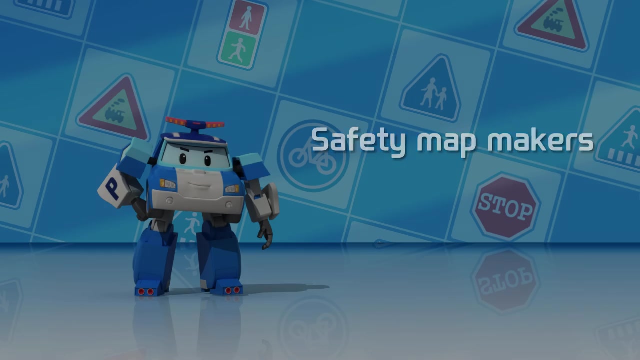 Whoa, Could it? No way, Ah, Oh, Wow, That's definitely aliens. We've totally made contact, All right, Ha ha ha, Ha ha ha. Okay, you know the assignment. Each of us is going to make a traffic. 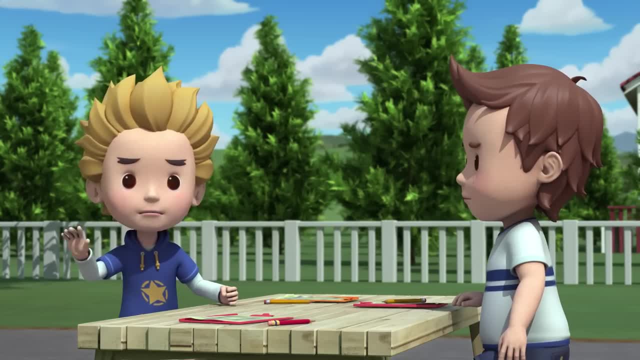 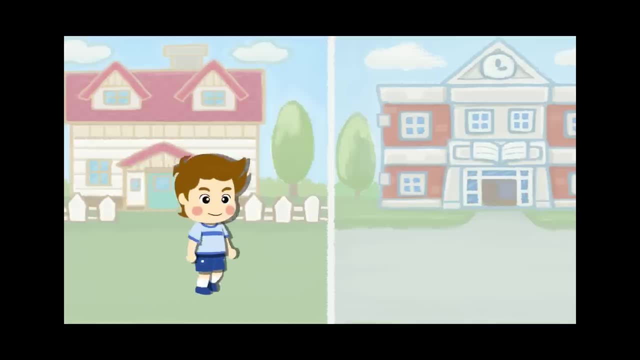 safety map of our town. What I'm not doing. that It's too hard. Kevin's right. How do we even make a safety map? It isn't hard at all. On your way to school, keep track of how many times. 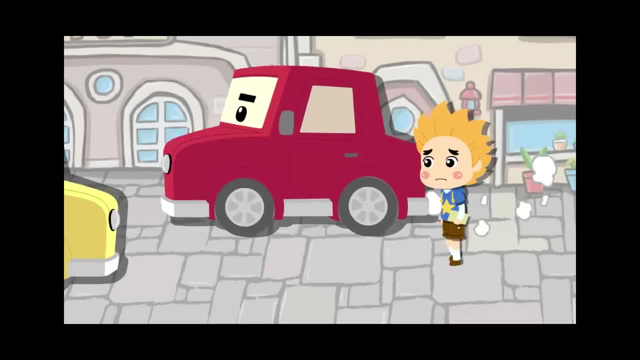 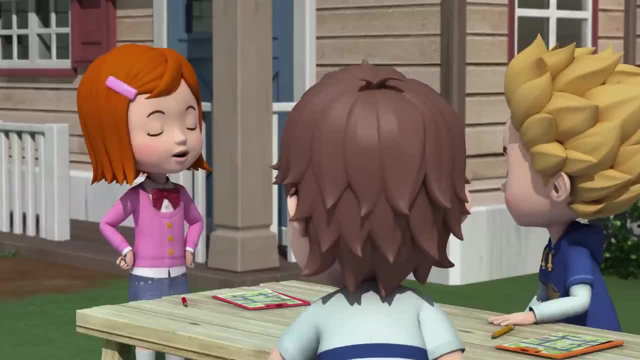 you cross streets whether there's a traffic signal, and if the roads are safe or dangerous, Then mark it on your maps. It's easy. No, it's not. Well, what if I told you this homework assignment gets you five prize? 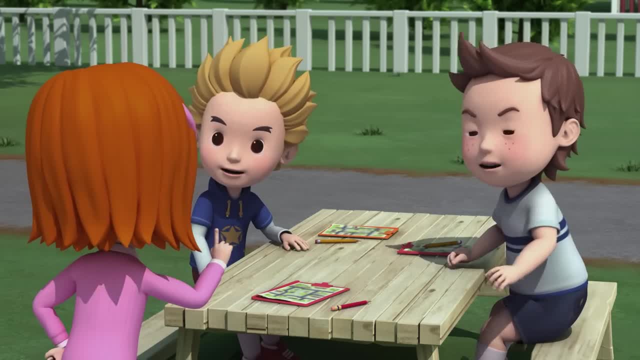 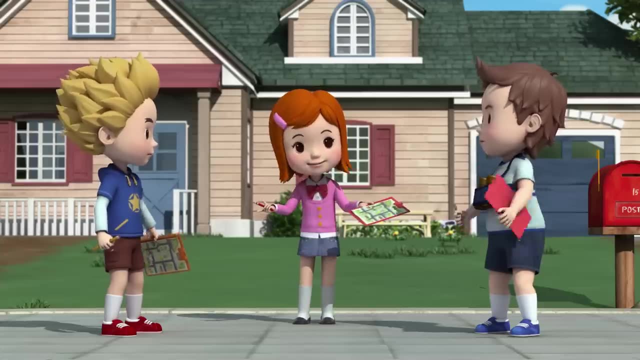 stickers if you do it right. Whoa, Really Yes, so we're going to do it, Okay. Okay, So we'll all go back home then meet up later at school, Right, Doug, Let's see who gets done first. 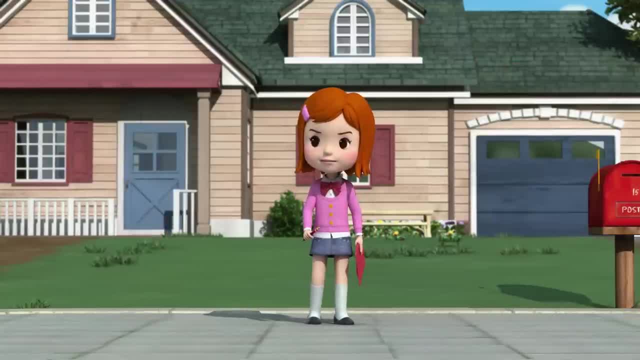 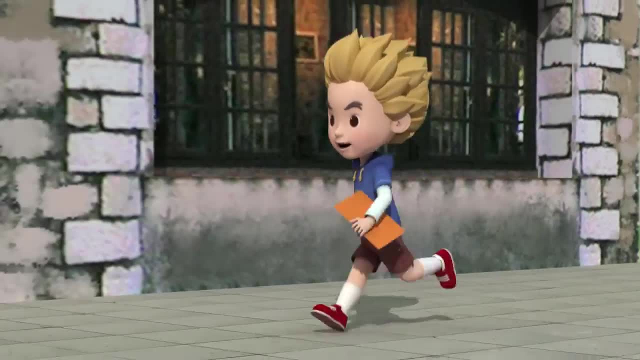 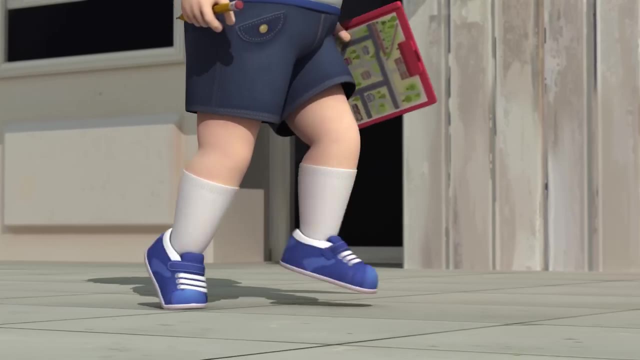 Me. Hey guys, What's up with boys? Ha ha, I'm going to win. There's a traffic light and the crosswalk's short, so I'm marking this as safe. Ah, This way is safe, Ha ha. 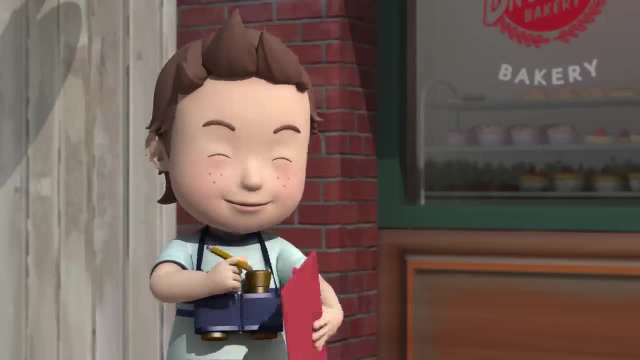 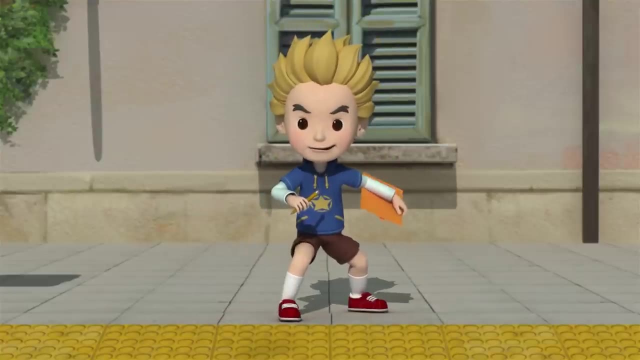 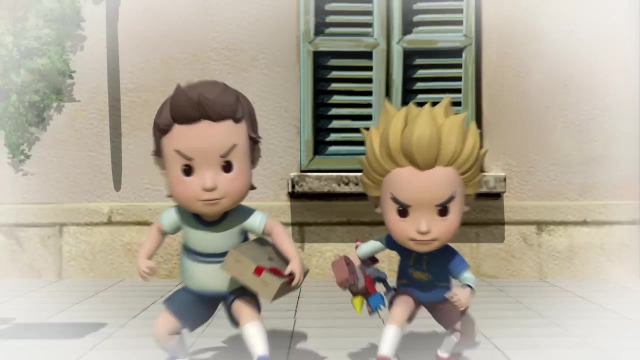 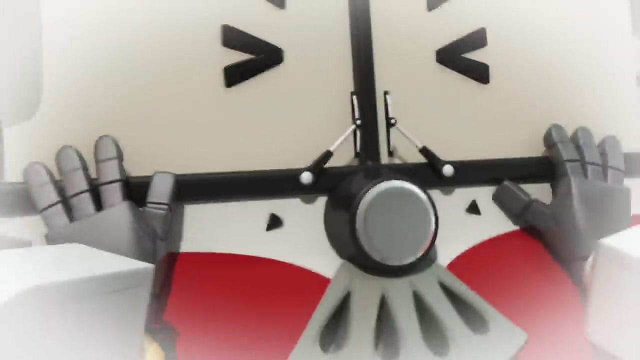 As long as I have money to go into the bakery and buy something to eat. Ha ha Ah. Come on, light Change. Huh, Hey, Green light Go Yay, Ah, What, What Easy. 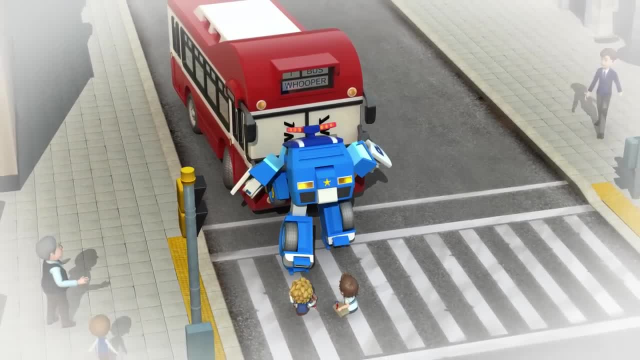 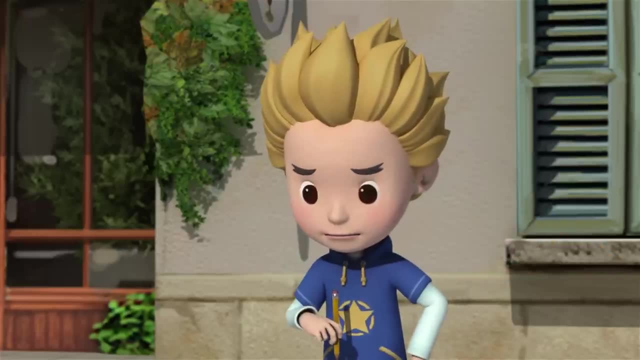 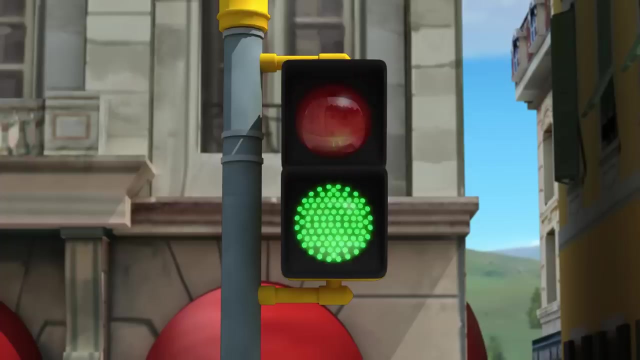 Pull away. Ah Yeah, I remember Holy. Ah, That was another close one. Well, I'll mark this one as a little dangerous, even though it has a traffic light. Whenever I cross, I put my hand up and make sure the cars see me. 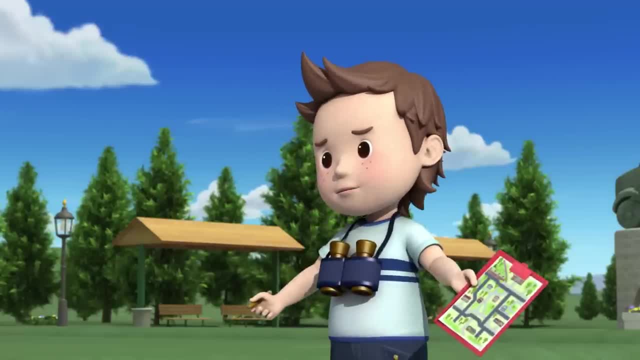 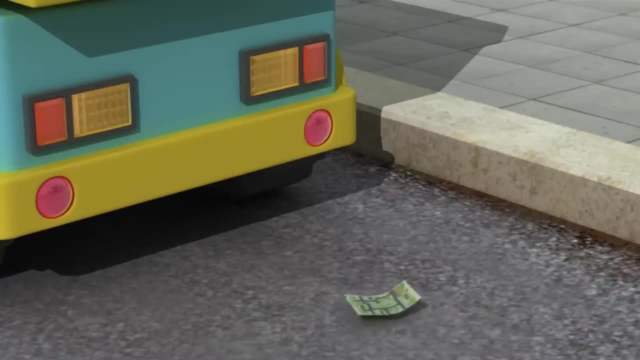 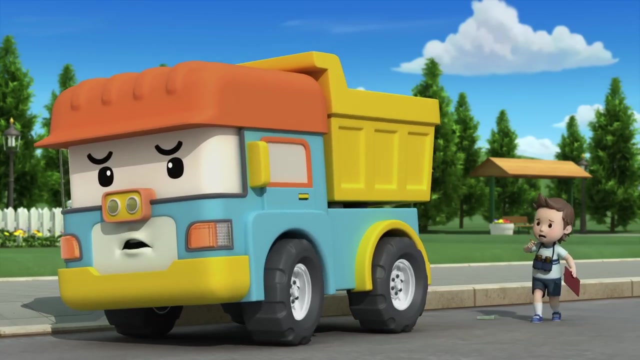 What? They're still not finished fixing the park. Wow, Where can we play soccer? We're supposed to be here today, Ah Ah, Ah, Oh, Doug, Bad spot. Never stand behind a truck. It's a very dangerous blind spot. 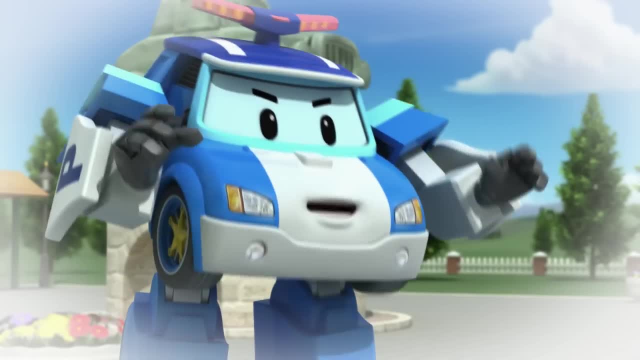 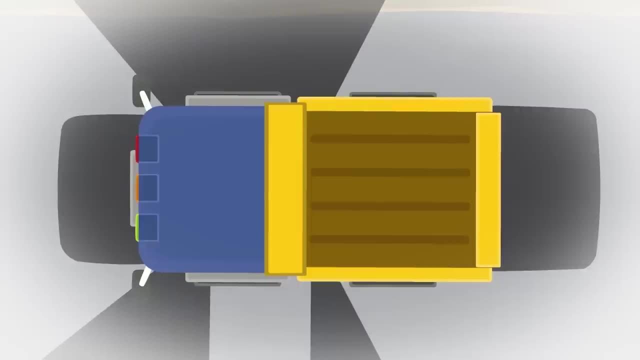 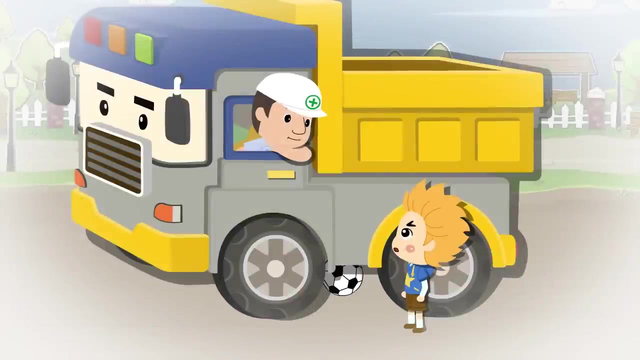 Blind spot. Never play around cars or trucks or underneath them, because they have blind spots. There are certain spots around cars, trucks and buses that drivers can't see, called blind spots. The bigger the vehicle is, the bigger the blind spots are. 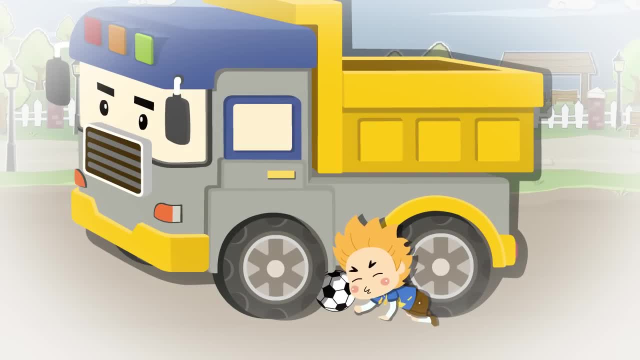 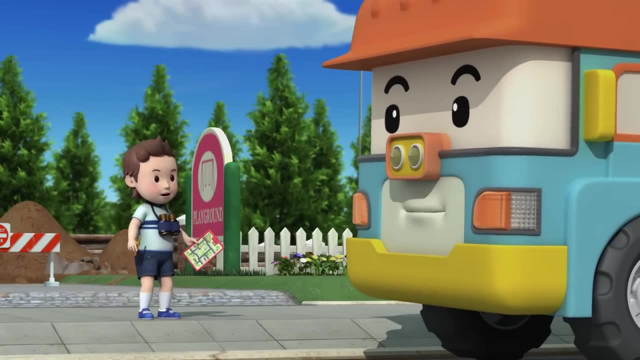 If children like you walk or play in these blind spots? the drivers can't see you. What would happen if a truck moved with you in its blind spot? That's right, Hey Dump, when will you be finished here? Mr Builder says it's going to take. 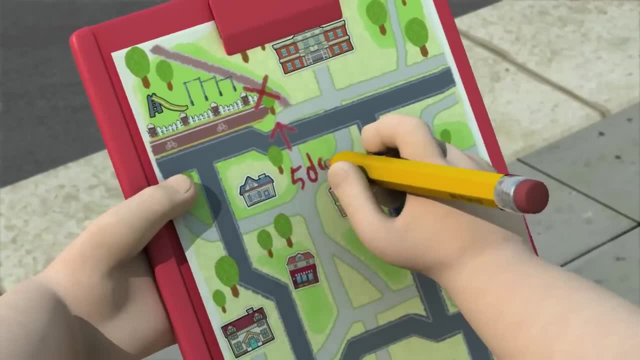 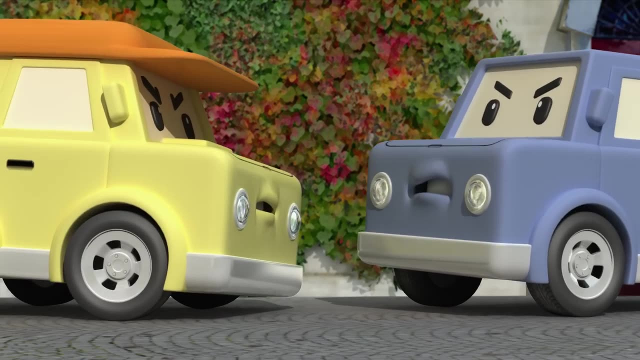 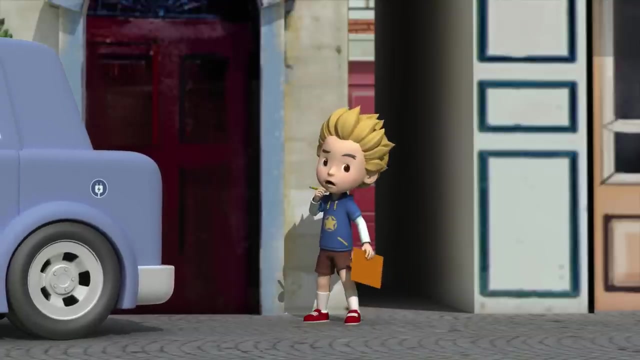 at least five more days. Five days, I see Bye-bye. Thank you, You're welcome, Doug. I was here first. You back up. I have the right of way. Oh really, What's wrong? This happened once. 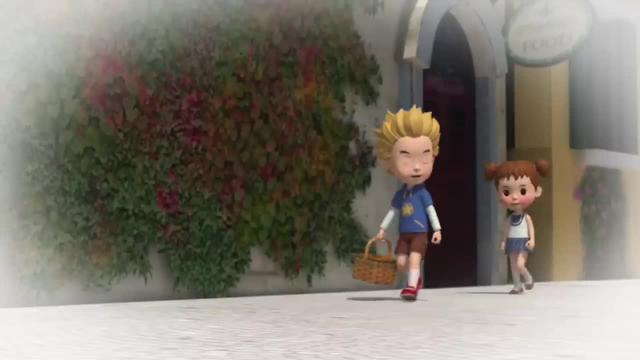 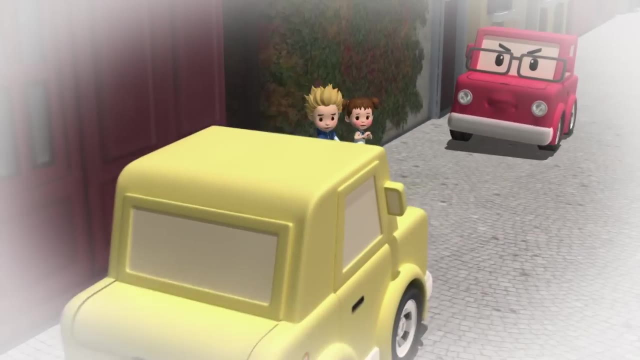 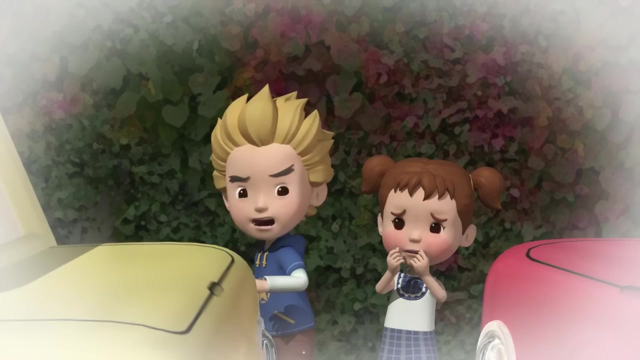 Heaven, Where are you going? This is the shortcut to Mrs Wura's. Whoa, This street is weird. Why do the cars come so close? Okay, pal back up. I came in first. What are you talking about? I was here first. 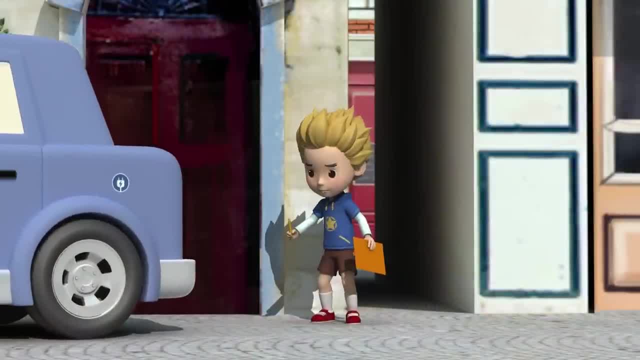 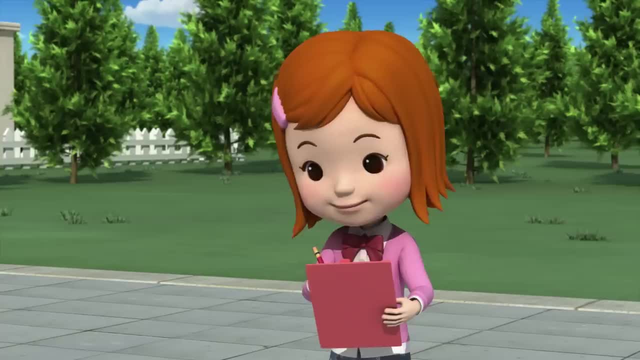 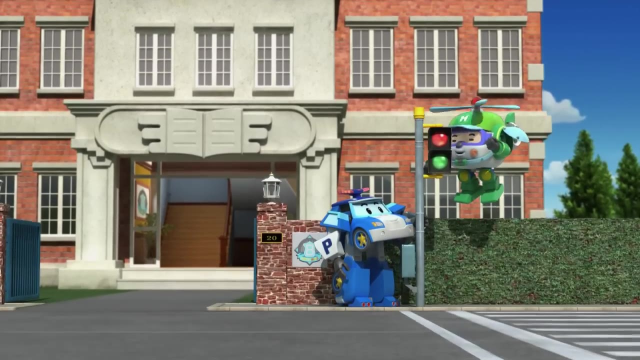 You back up. Mrs Curry, I'm putting down to take the long way because it's safer, Right, Kids should be extra careful here because there isn't a traffic signal. Fixed it, Polly Hooray, I won, Doug. 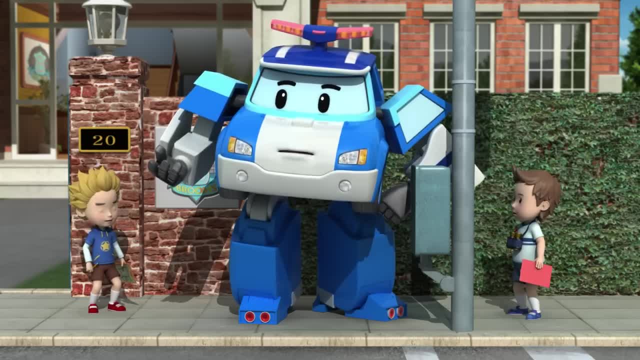 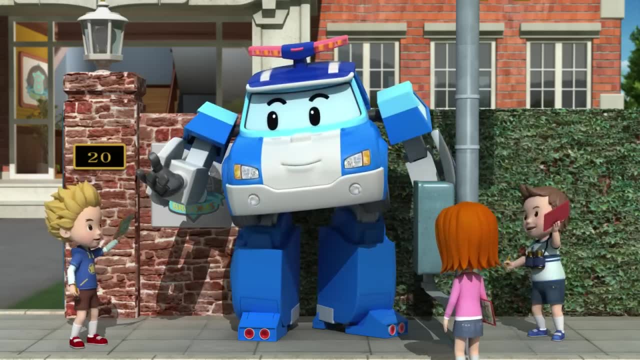 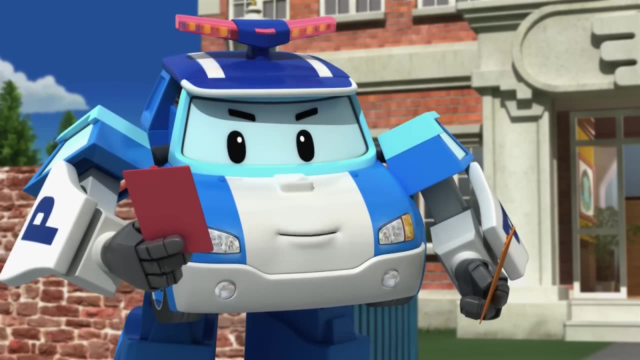 Not by much. What are you doing here, boys? There's no school today. I can explain. We all had some homework, Homework, Yeah Well, you all did a great job of showing safe and dangerous ways to get around town. 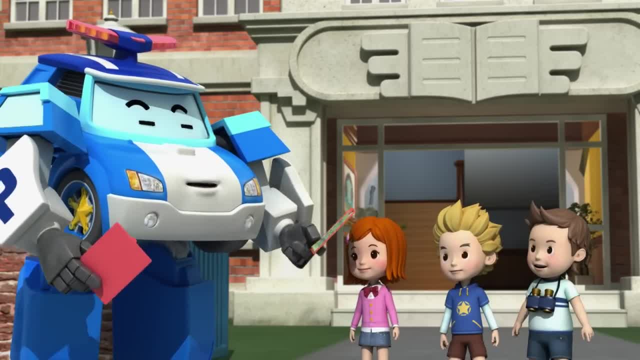 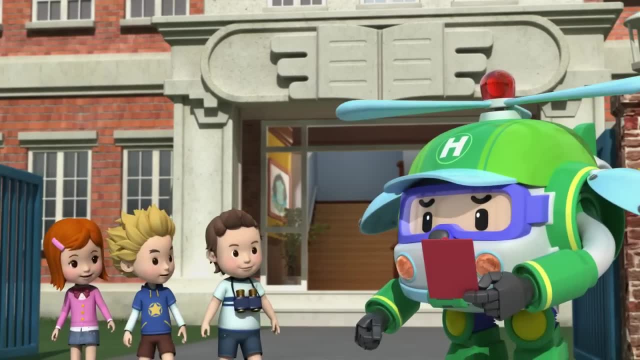 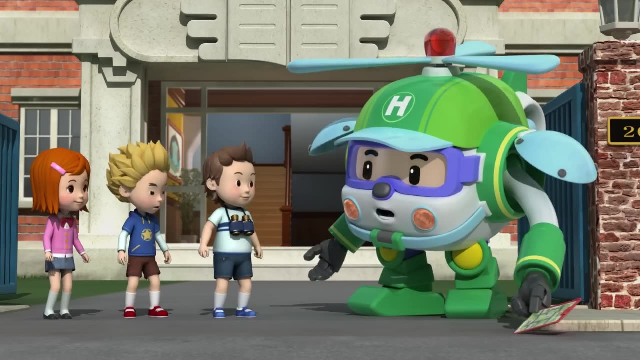 If we had a few more mapmakers like you, I might not have very much to do anymore. Thanks, Polly, Say Doug, Yes, Does the symbol around the OK mean the street's extra safe? That symbol stands for a muffin. 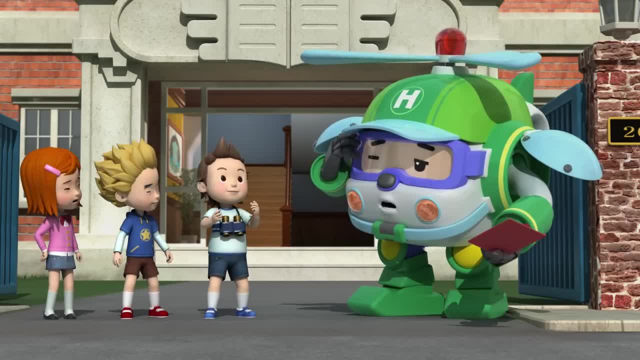 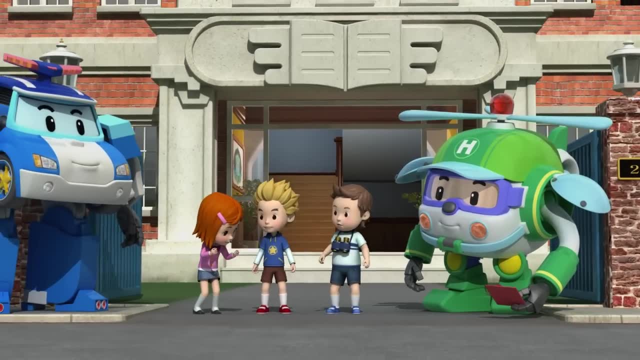 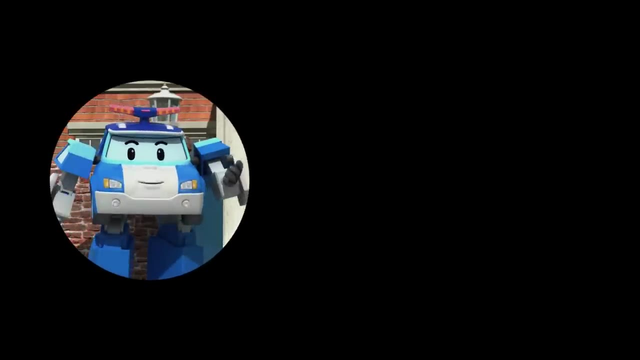 Why a muffin? There are bakeries on that street. Any street with a bakery on it's way too dangerous a place for you. Why All you'll be thinking of are muffins instead of the traffic. You're right, I have an idea. 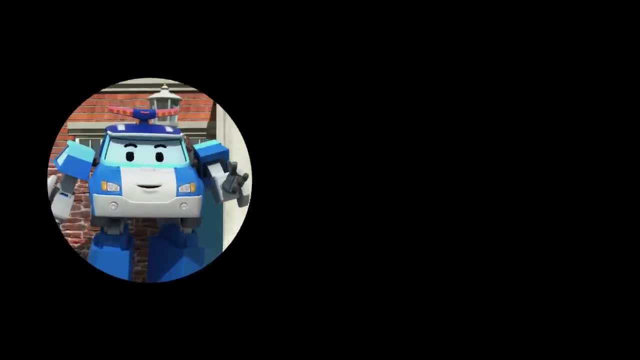 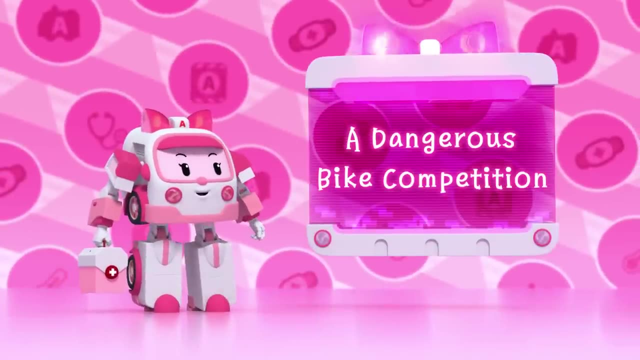 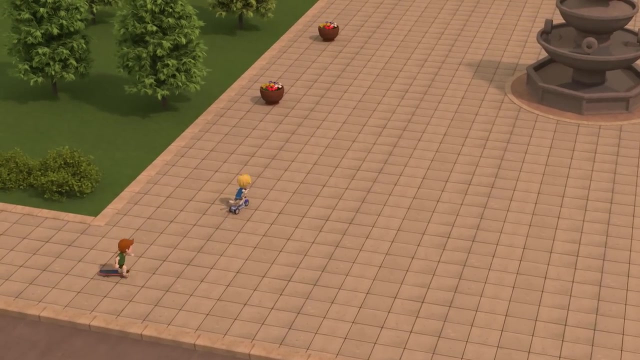 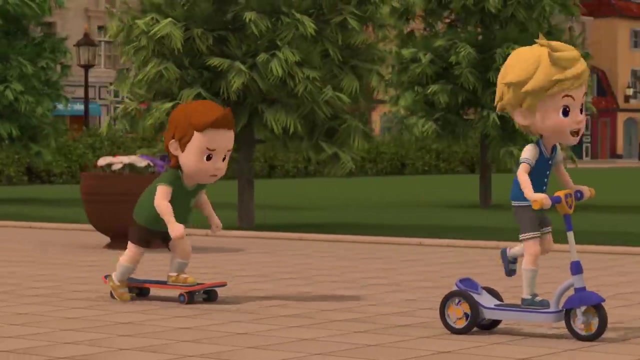 Why don't you and your family make a traffic safety map of your neighborhood too? Sure, Let's do it. Oh my God, I'm gonna be so mad. Those are great. I'm gonna be so mad. I'm gonna be so mad. 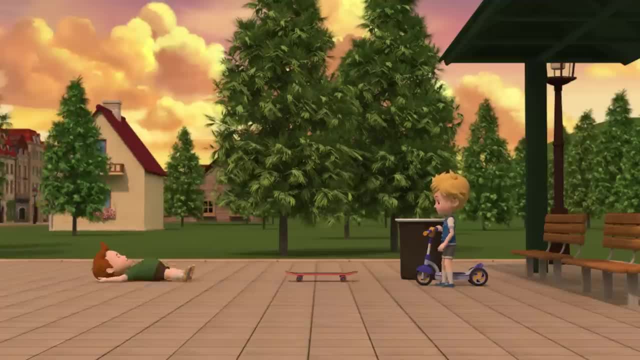 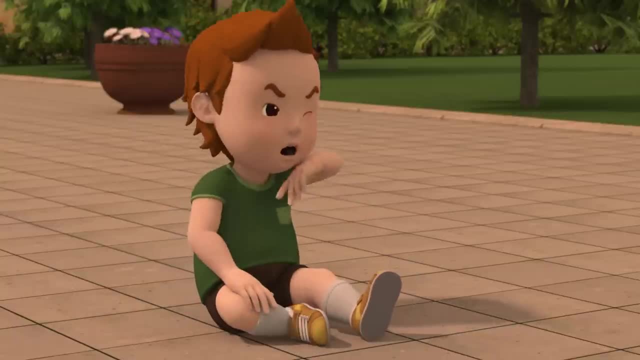 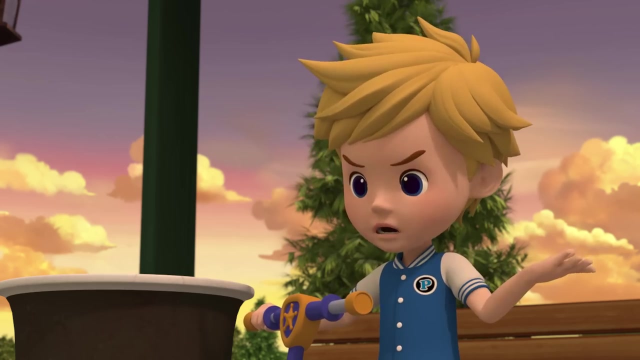 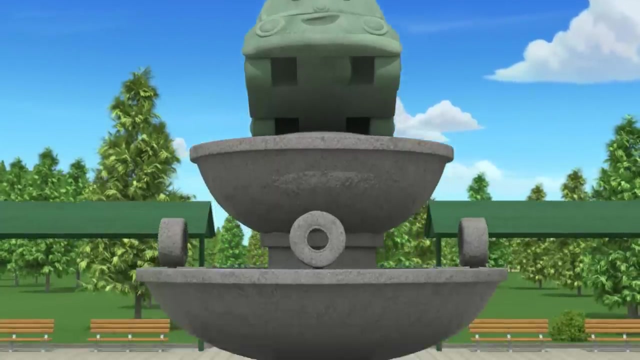 Oh yeah, Good job, Turbo. Well, Johnny, looks like I win. I'm feeling a little tired so I went easy on you. all right, But next time, huh, same time tomorrow- rematch. prepare for my victory. why is Johnny so late? 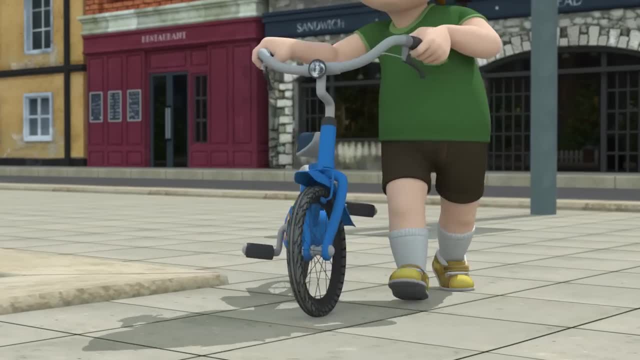 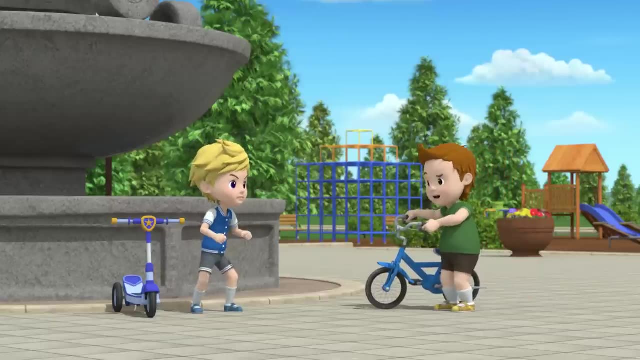 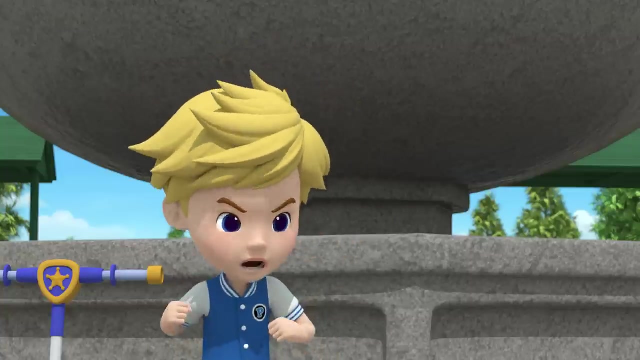 Peter, what's going on? think you can beat me if you're on a bike. we'll see. unless you're afraid to race me on this, that is huh afraid to race you. I'll beat you on that and prove that I'm the best once and for all. all right, what are we? 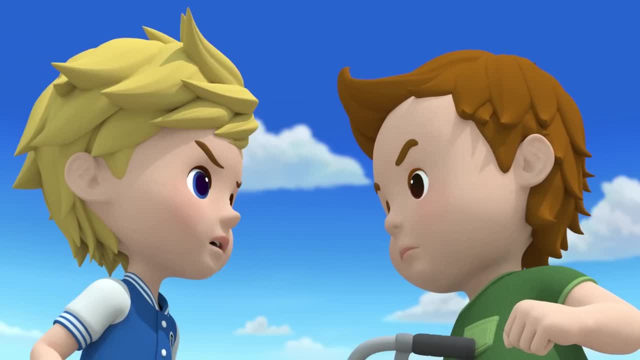 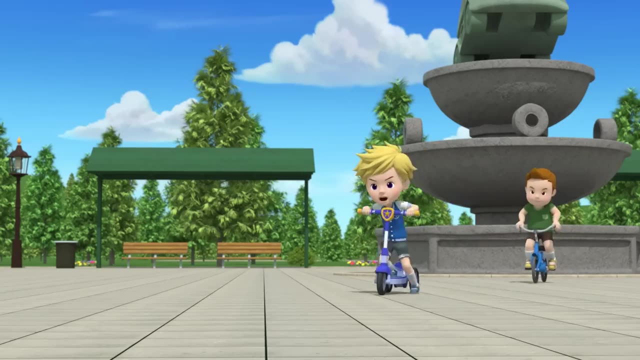 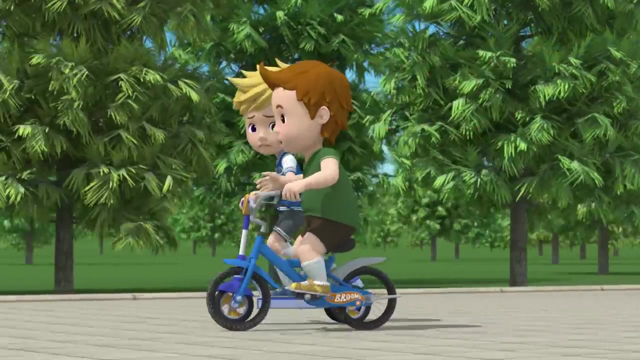 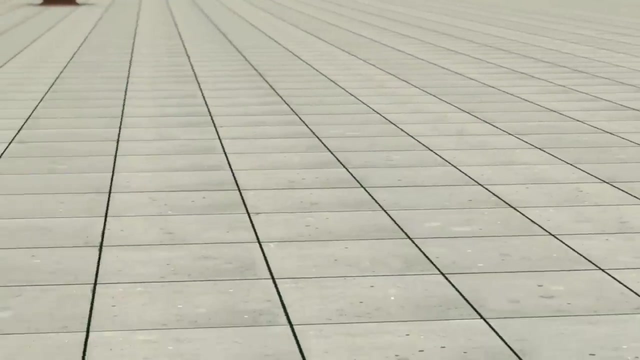 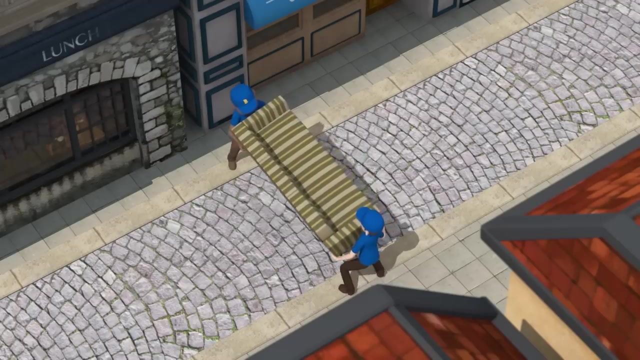 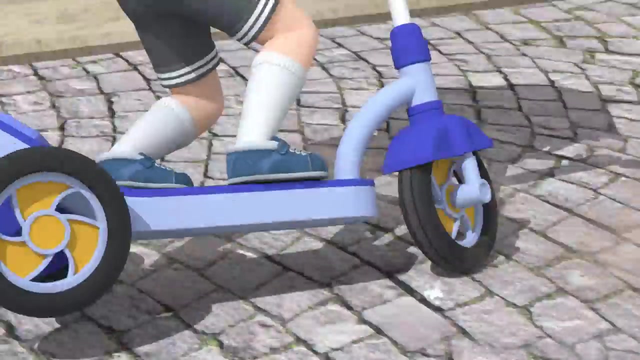 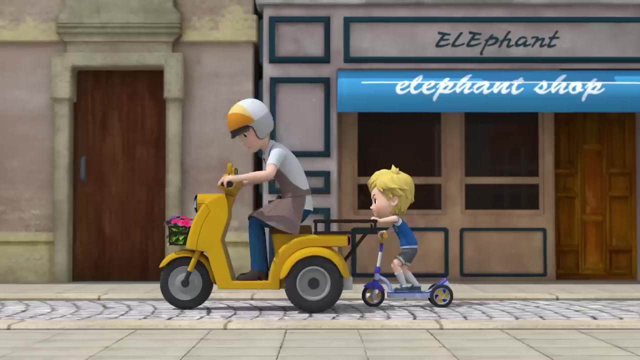 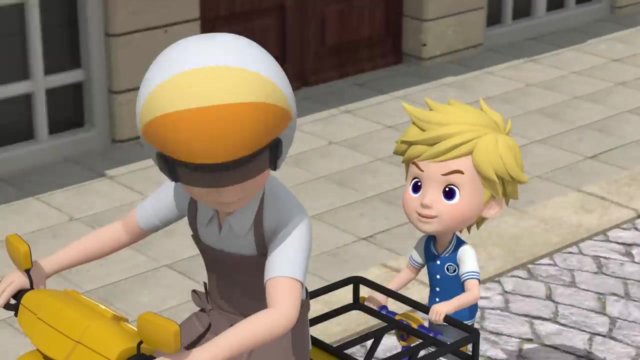 waiting for, let's race. great, then, whoever gets to City Hall first, the winner. you're on one two. how's it going? see you at the finish line. slowpoke, call me slowpoke, you'll be sorry. what are you doing, kid? hi, there, huh, there's Johnny. thanks, see you later. 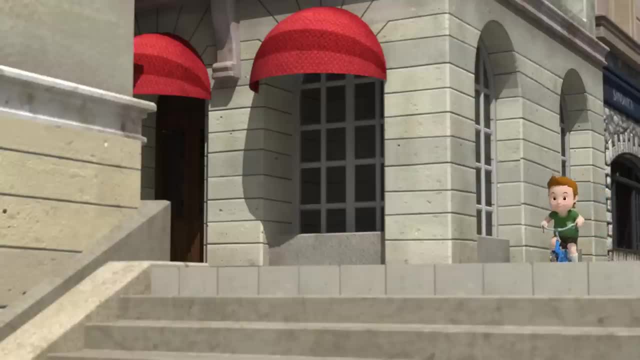 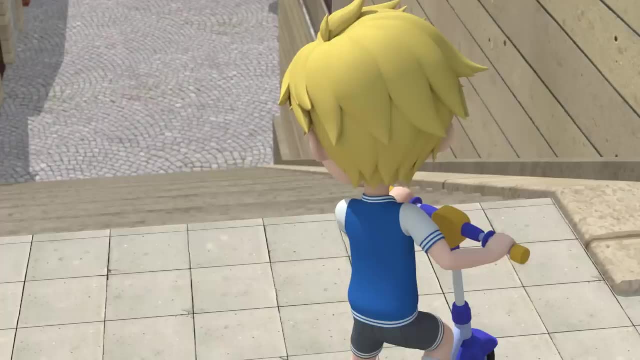 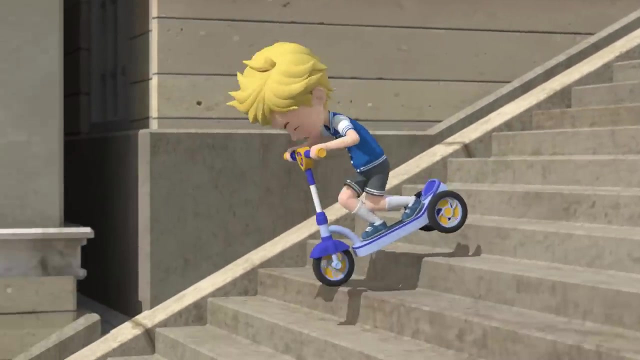 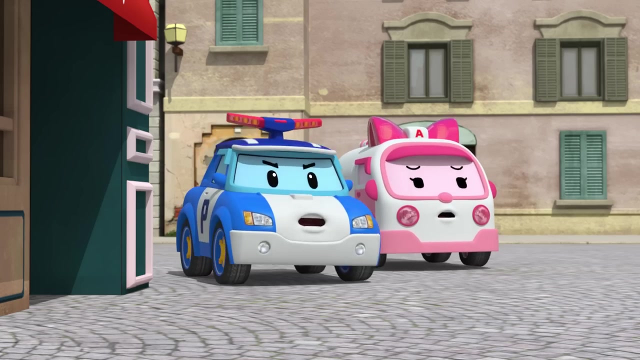 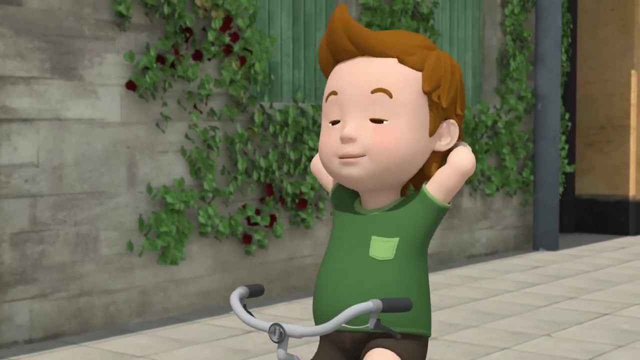 goodbye. I'm pretty sure this way is a shortcut. should I go for it, he might be in trouble. Peter won't be bragging after today. there's no way he can outrun my bike. Ha-ha-ha, Who's the slowpoke now? 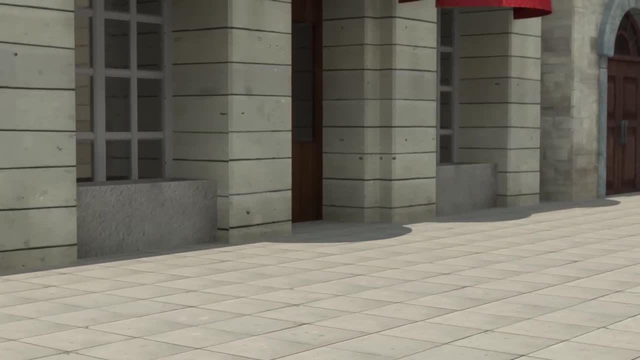 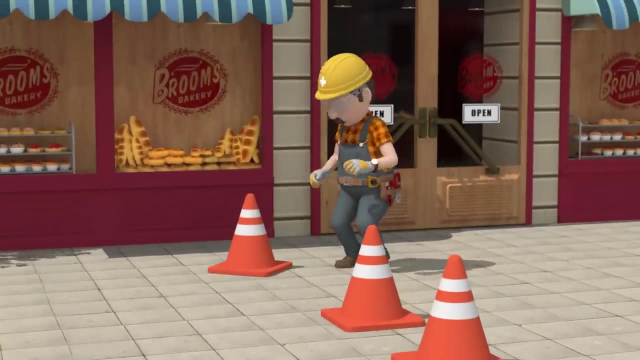 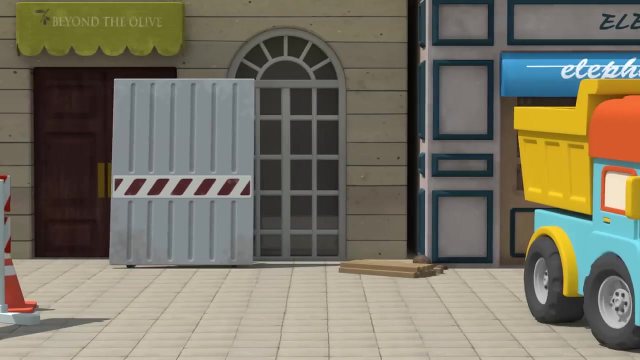 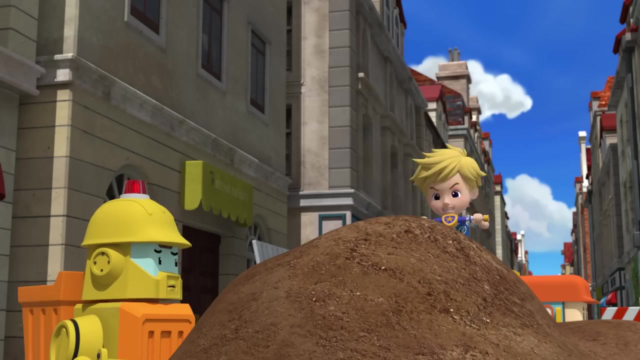 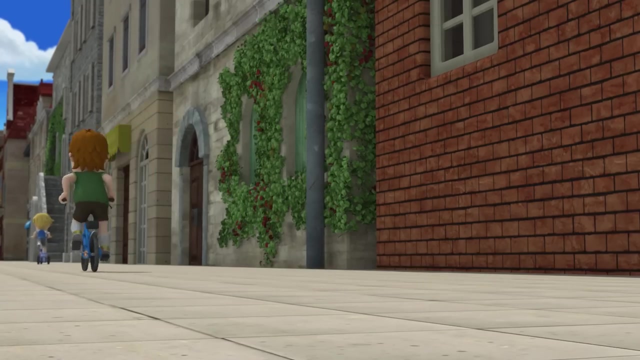 Huh, Oh, no way Out of the way. Oh, my goodness, You two-wheeled menace Coming through. mister, You, darn kids, Let me by Me too. Hey, that's dangerous. Yah, Hey, you guys. 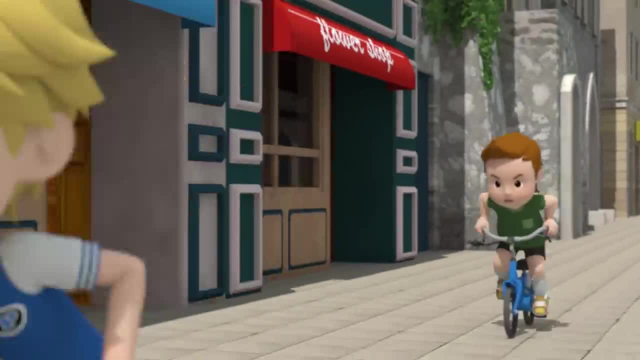 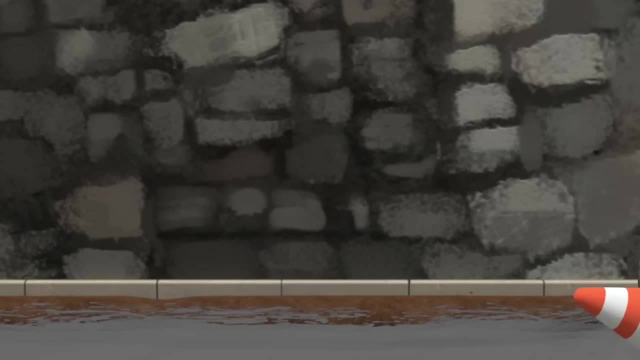 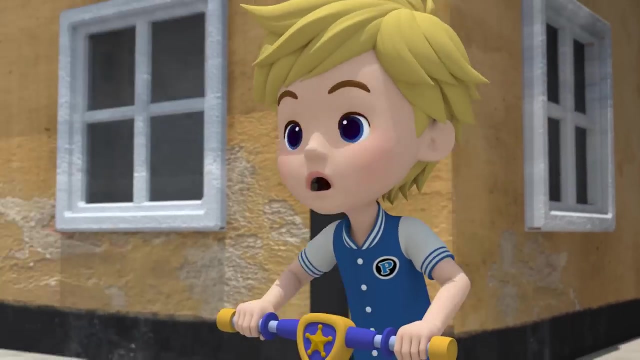 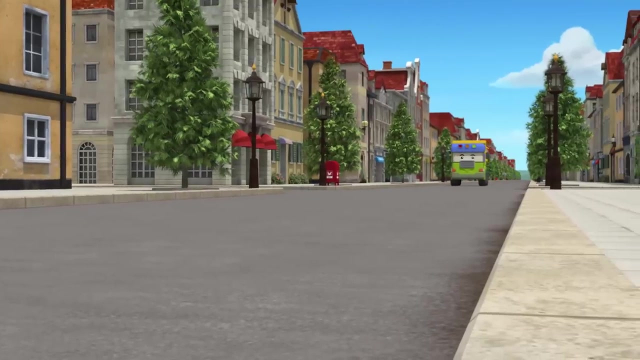 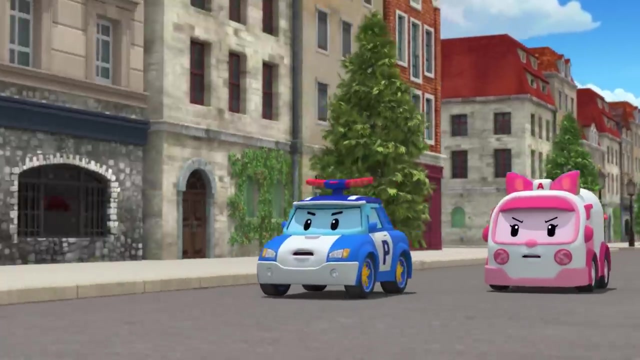 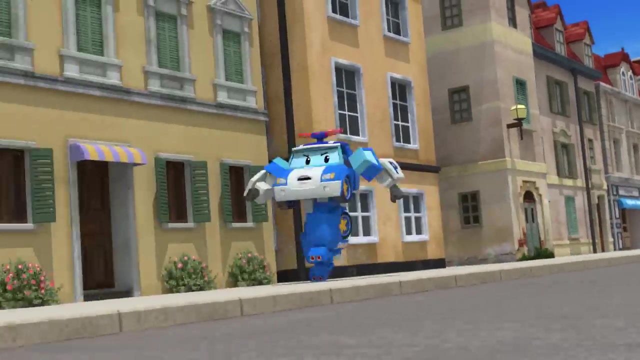 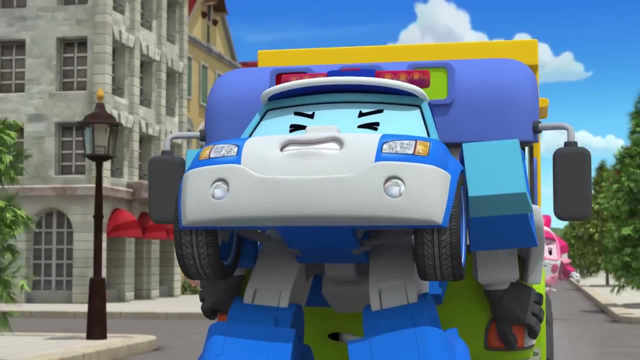 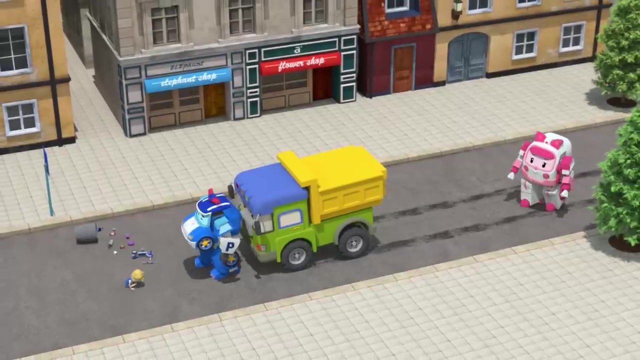 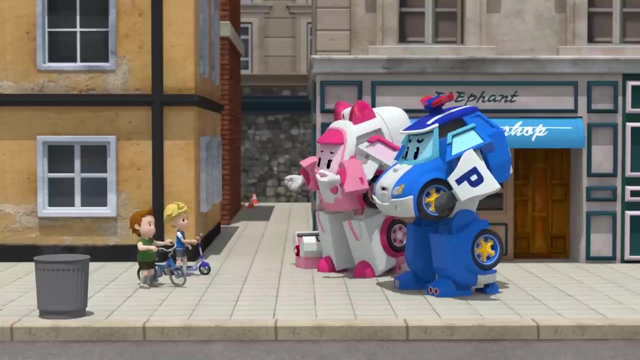 I'm coming, Peter, Johnny, faster, faster. Hey, what is this? I win again. Huh, It's a kid. Watch out, Ah, Yah, Yah, Ah, Oh Ow, What a close call. Riding is dangerous without protective gear. 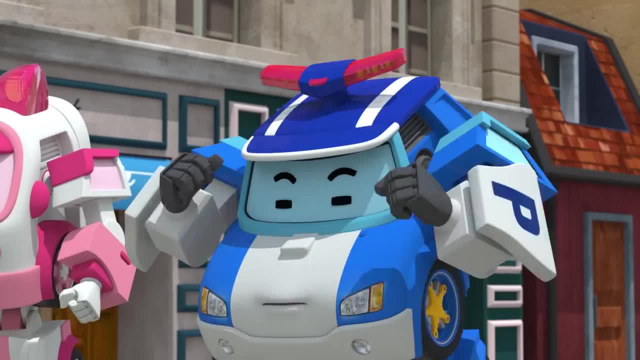 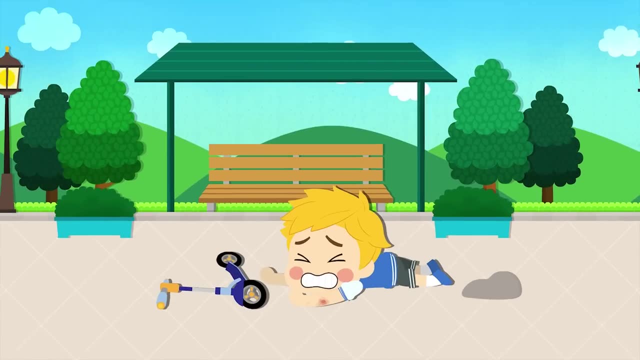 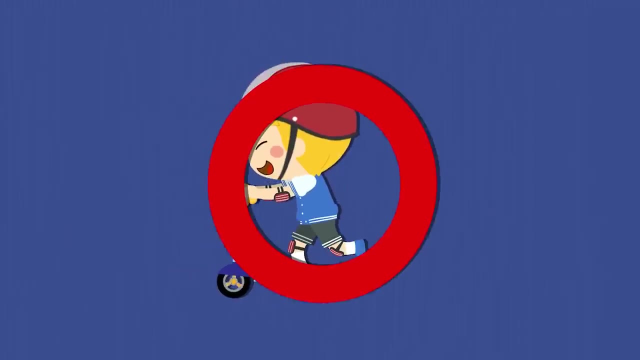 Peter, Johnny, when you're riding vehicles like a scooter or a bicycle, there are things to remember. If you ride a bike or scooter without wearing protective gear, you could seriously be injured. You must wear safety protective gear properly. Don't ride in construction sites, driveways or crowded sidewalks. 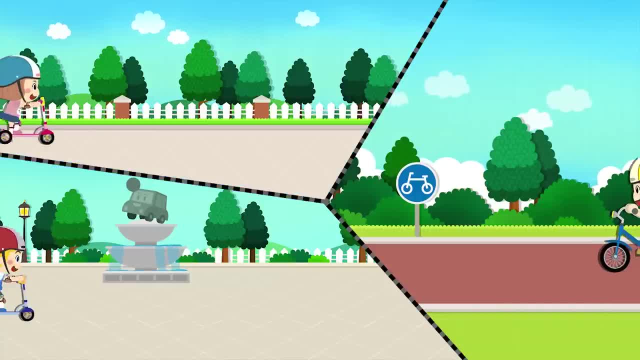 You should only ride in safety protective gear. You should only ride in safety protective gear. You must not ride in safe places like private roads, plazas and parks. You must not ride in safe places like private roads, plazas and parks. 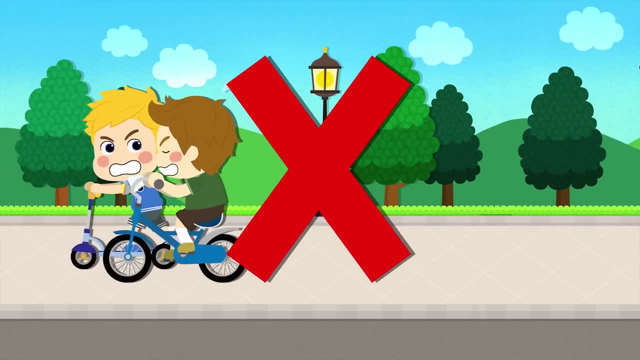 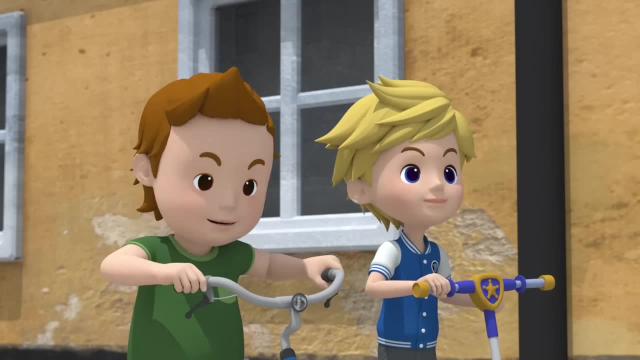 And it's dangerous to do tricks or compete while you ride. Riding is great fun, but let's do it safely. Got it, Mm-hmm, We get it, Poli. Hey you guys. You speed freaks made a mess of our construction site. 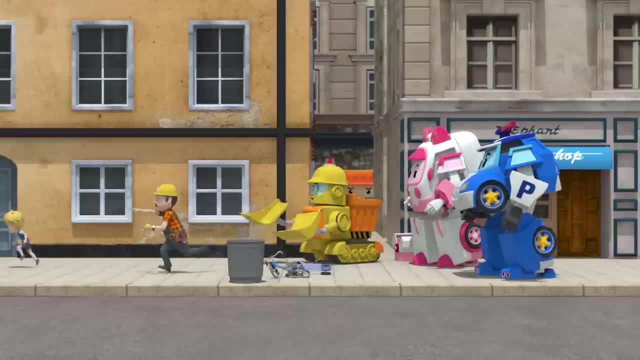 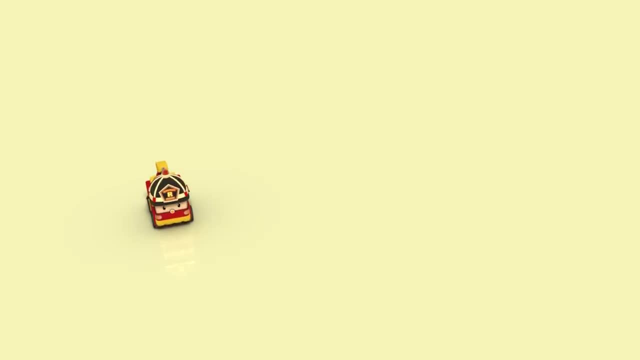 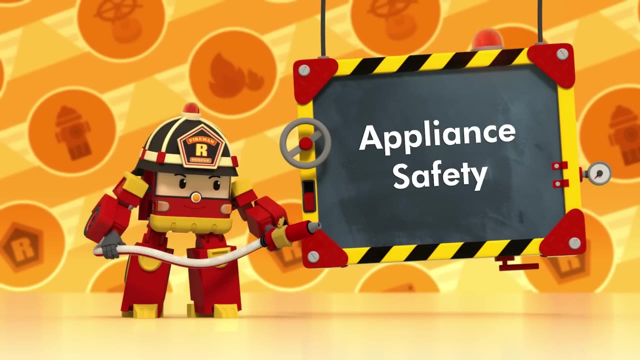 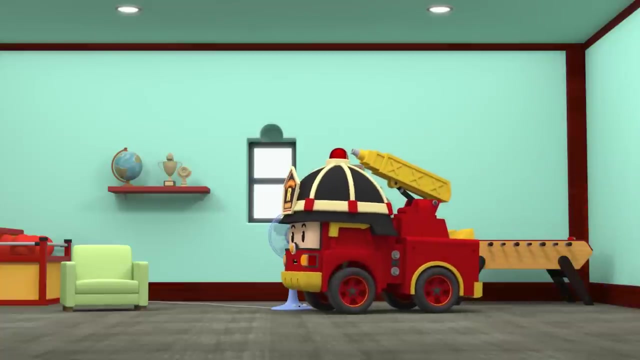 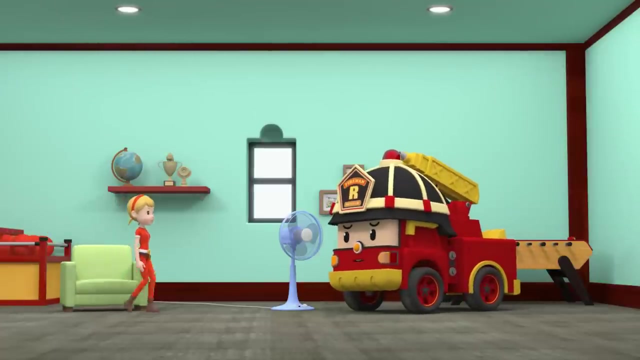 Ugh, Come on, run away, Come back here, You kids. I'm sorry It won't happen again. Gin Gin, She left this running with nobody here. Oh, I'm sweating. Oh, hi, Roy Gin, you left this fan on and it could have overheated and caused a bad fire. 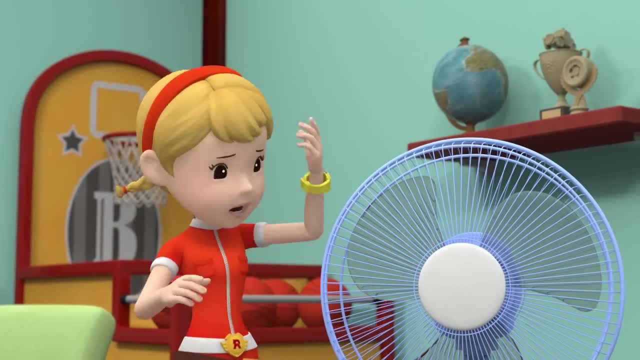 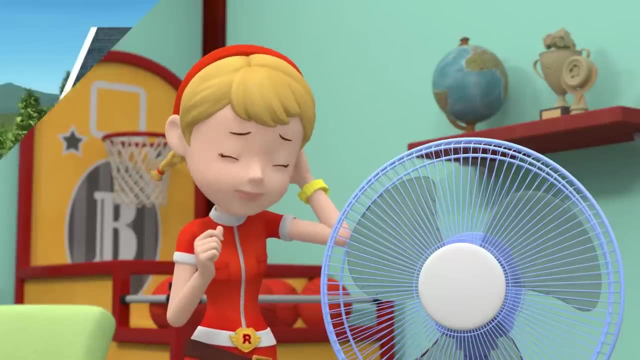 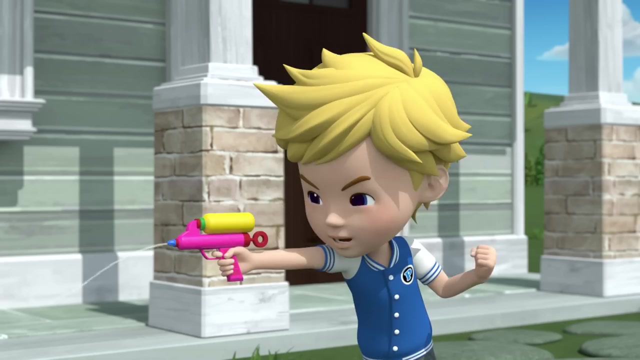 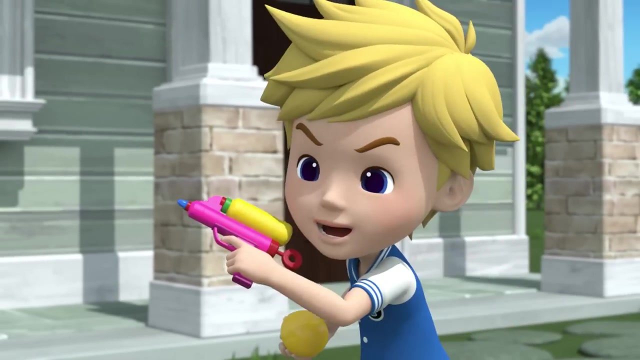 It's all right. I barely left it on for that long. Ow, it's hot, Are you all right? It started to overheat. You have to turn it off. Okay, Roy, Take that All right. Never saw that coming, did you? 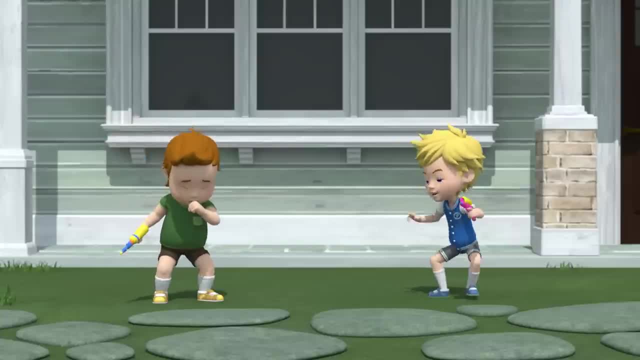 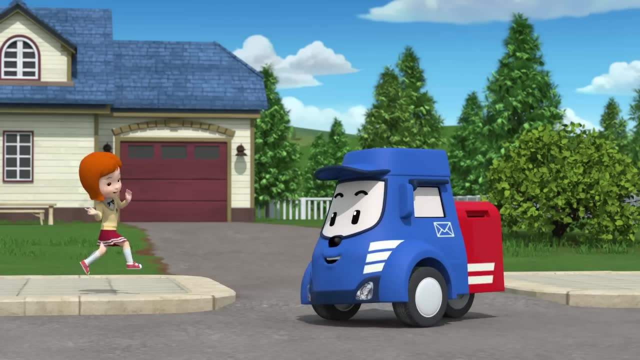 No water balloons allowed. I got you all wet. Stop right there. Oh hi Posty, Hello Cindy, You waiting for this. Oh it's here at last. I knew you were waiting for this book, so I came right here. 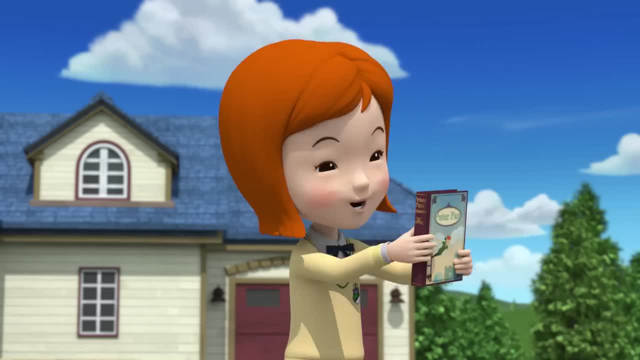 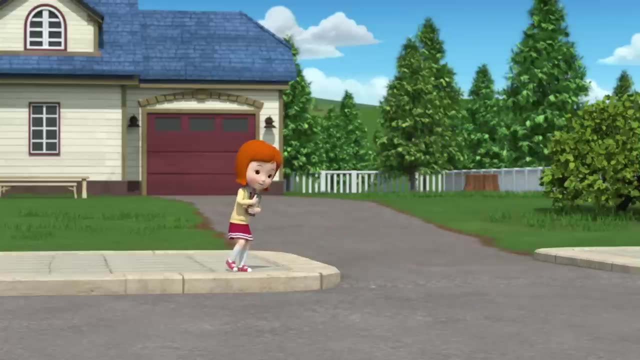 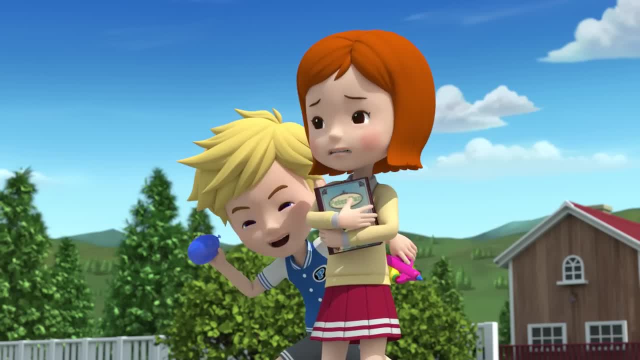 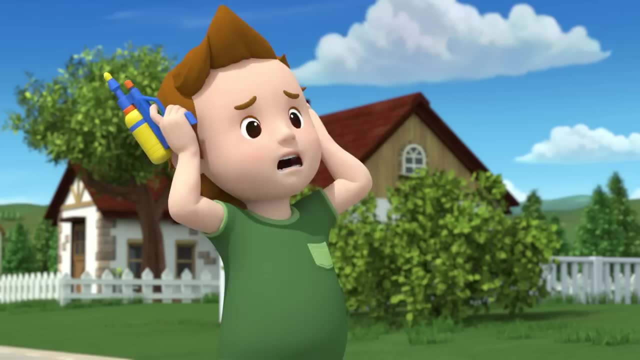 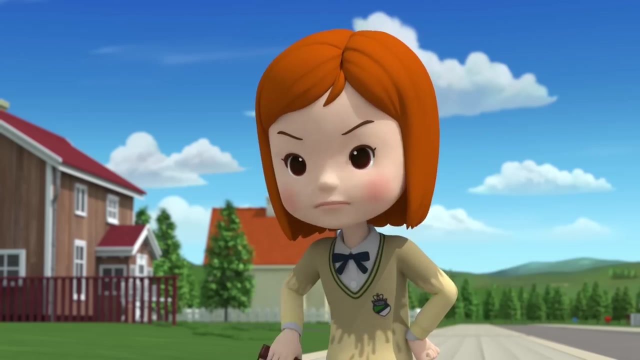 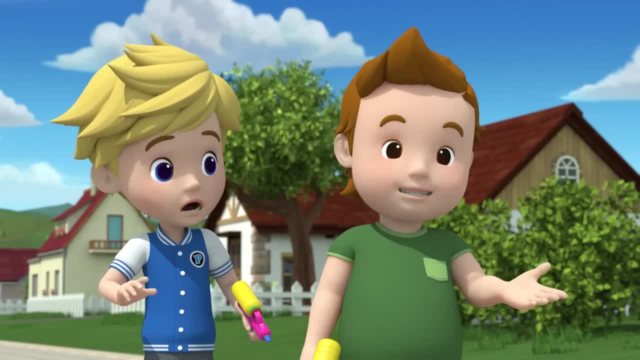 Huh, Peter, You just got my brand-new book all wet. I um, I'm really sorry about that. I know We can take it and get it all dried off. You'd do that? Yeah, Of course we would. 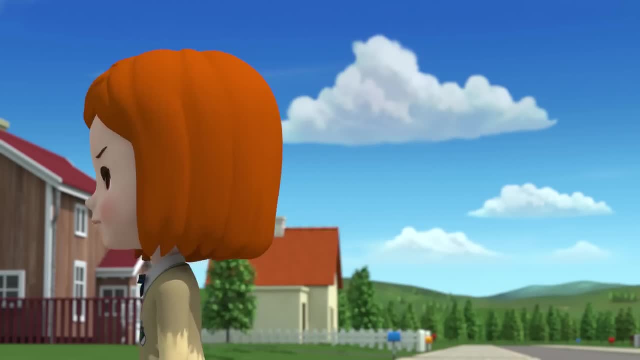 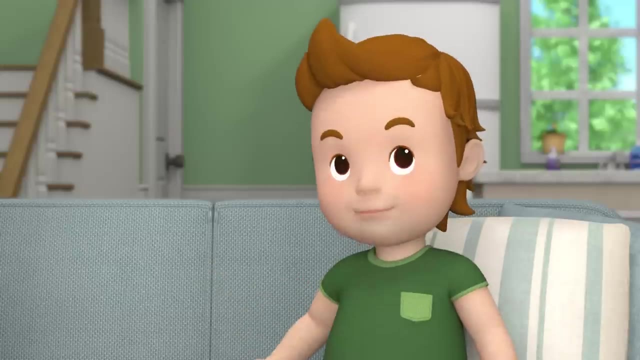 Uh-huh, That's right. We'll make sure it's as good as new again. Give it here. You better fix it. Hmm, Hee-hee, How are we supposed to dry this book? Who knows? Um, maybe the washing machine? 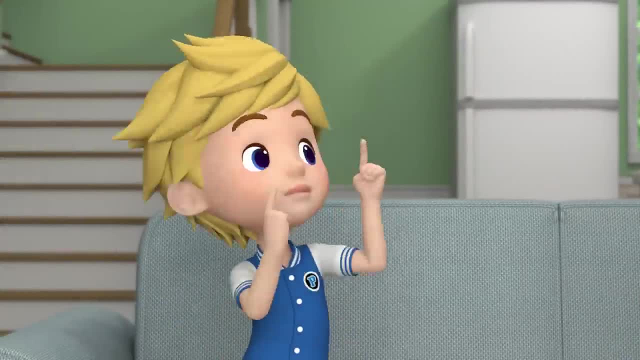 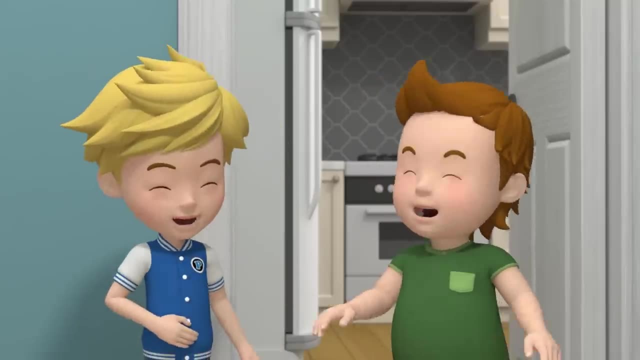 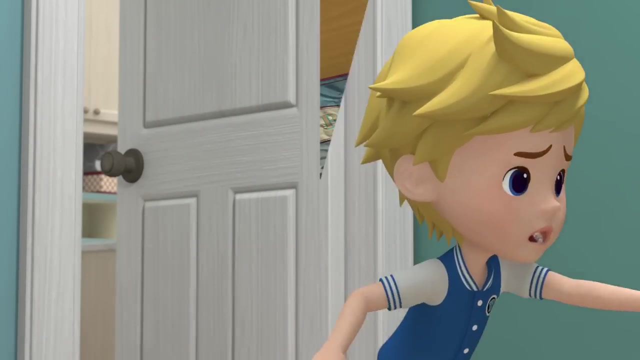 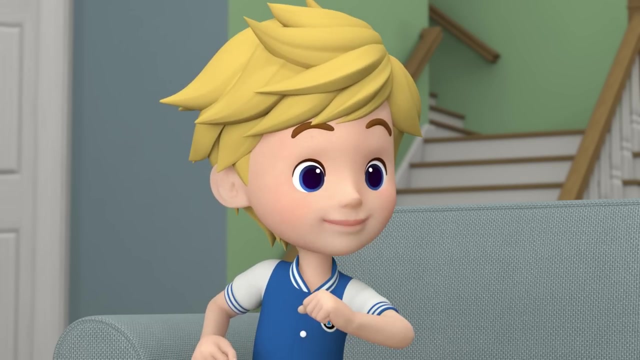 How The spin cycle. Johnny, let me think That's it. Let's do it. Turn it off, Turn it off. Well, that was a fail. Maybe the toaster might work. It's so hot, it'll dry it up. 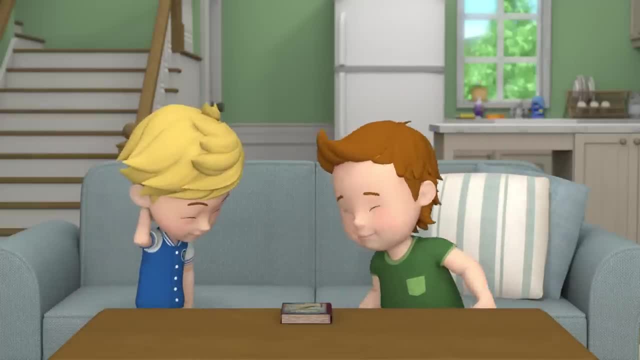 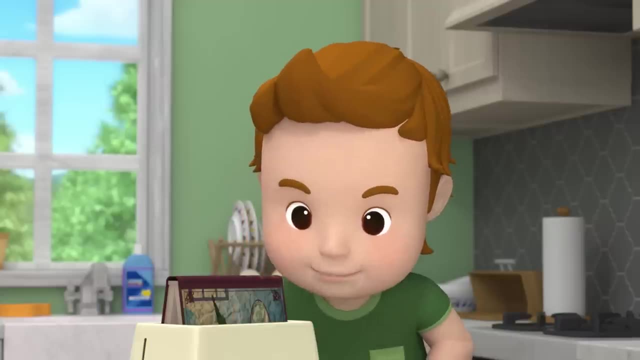 You're right, Peter. you're the smartest kid I know. I am, aren't I? Hoo-hoo, Doesn't that smell great? All I want in this world right now is toast. Oh, Peter, Look, It's on fire. 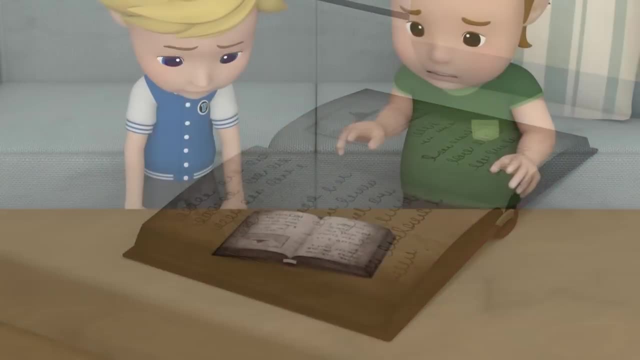 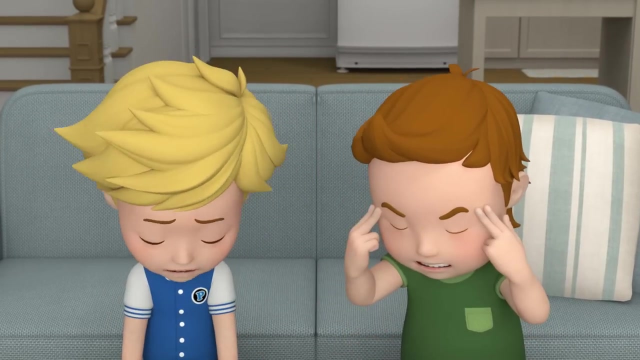 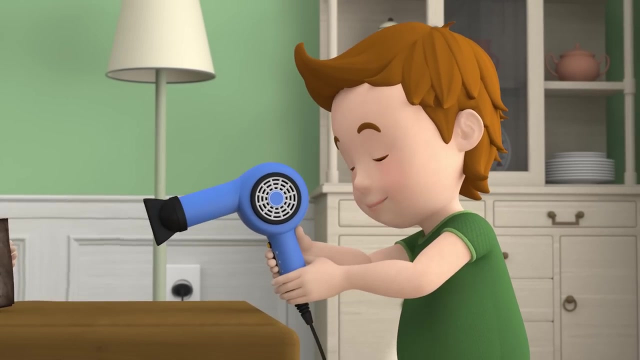 Ah, Water, Huh, Huh. So what should we do? Cindy's gonna be here soon to pick it up. I got it: The warm air will dry up this book in no time. Yeah, Why didn't I think of it first? 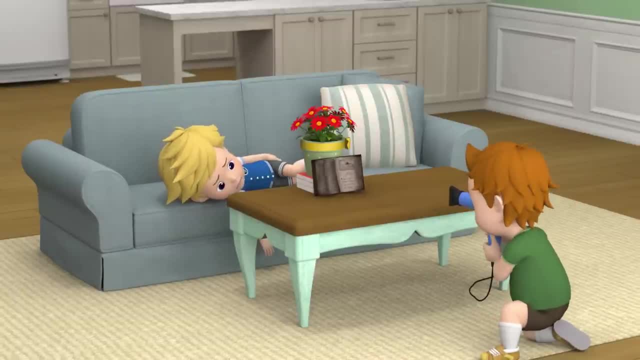 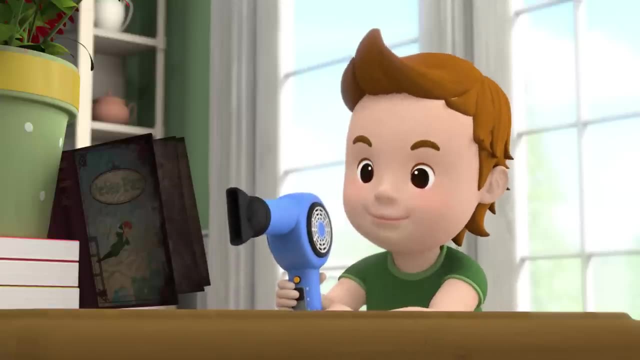 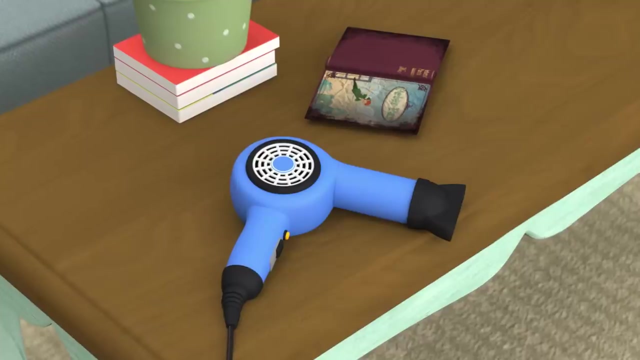 Johnny, is it done? I wanna go home. I think we're almost there. Huh, What happened? Oh, all right, Come to papa. Ah, Ah, No wait, Peter, that's my ice cream cone. 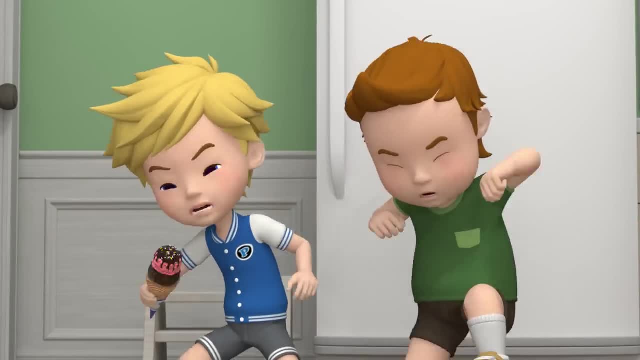 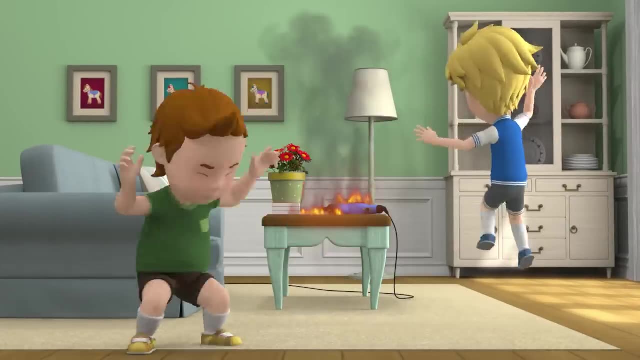 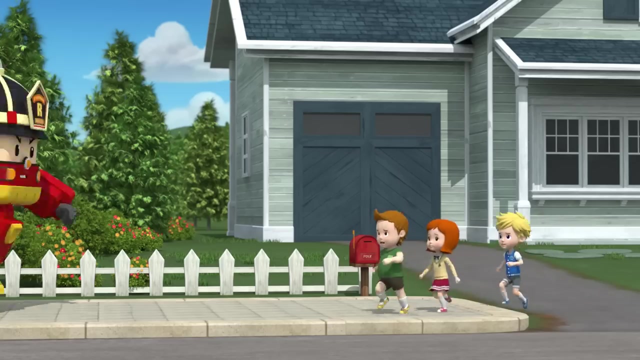 Wait, why can't I have some? Ah Huh, Ah, You're in. Ah, Ah, Fire, Fire, Fire, Fire, Fire. Huh, Is that smoke at Johnny's house? Hey kids, are you all right? 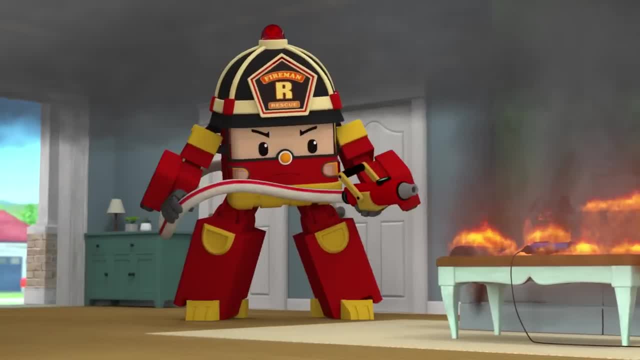 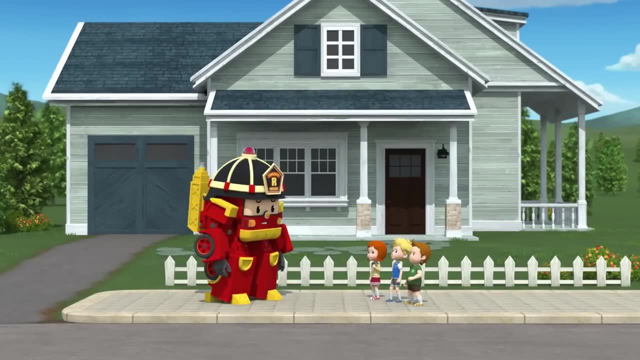 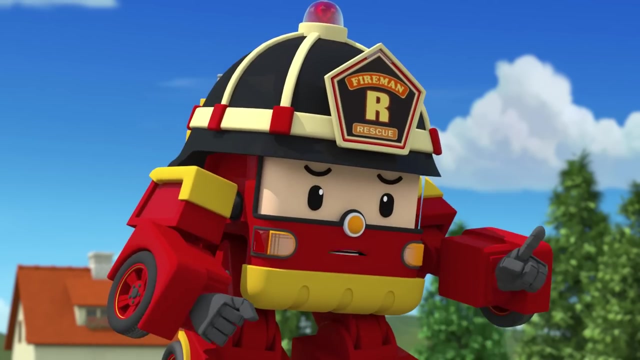 Just stay right there. Huh, Is everybody okay? We're okay now. all thanks to you, Roy. You guys, you can't leave an appliance on and unattended. Small home appliances can overheat and cause a fire, So even if you're just leaving the room, 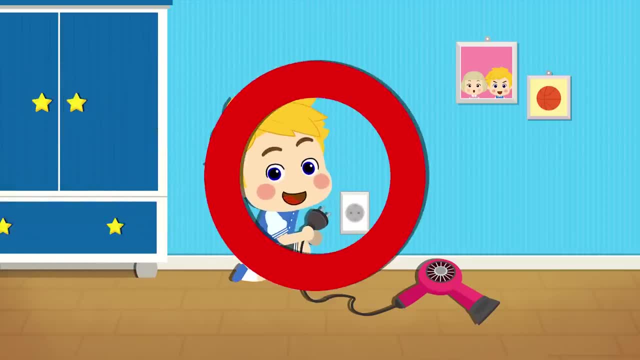 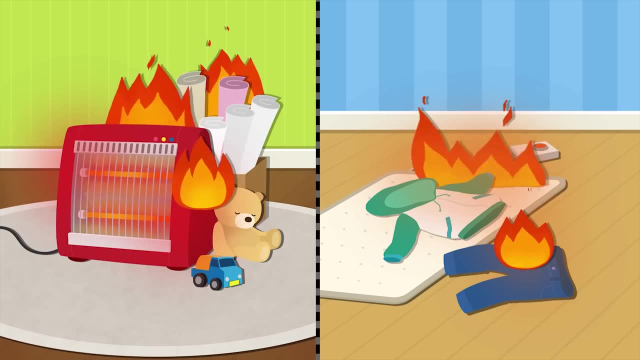 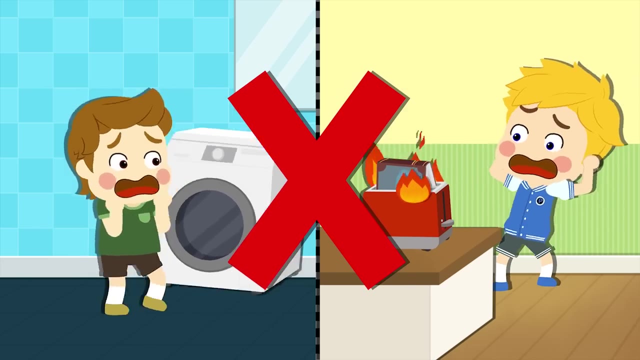 make sure that they're off. Also, be sure not to leave flammable items near electric heaters or blankets. And last, only use appliances for their intended purpose. Ah, Ah, Ah. Okay, we get it now. Hold on Whatever happened to my book. 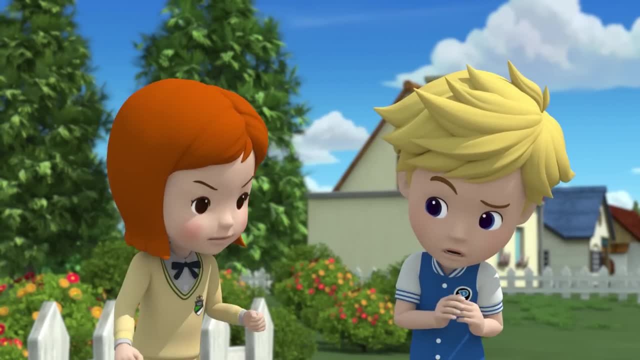 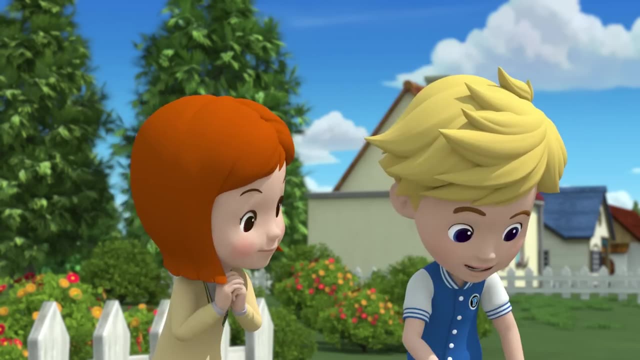 You better hope it wasn't damaged in the fire. Come on, Cindy, You can always trust me, I'm not going to lie to you. Trust me to take care of things. Ah, It's fixed. It's not wet. Here you go. 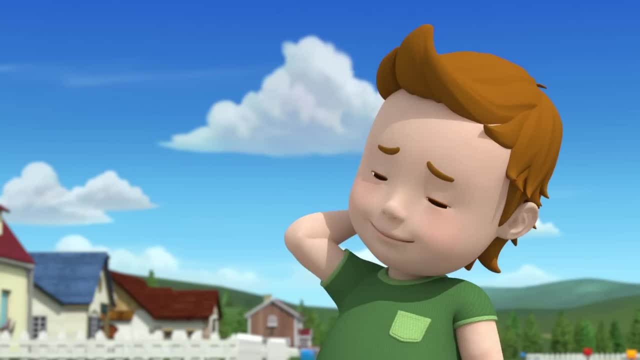 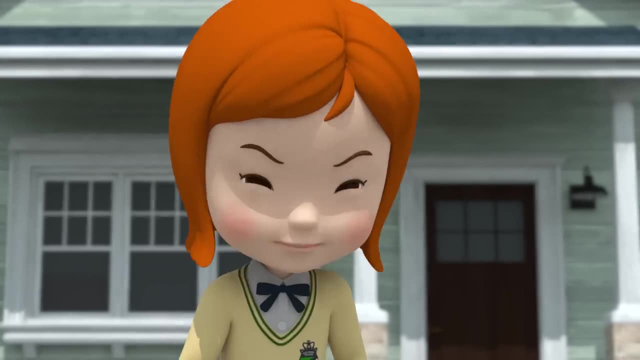 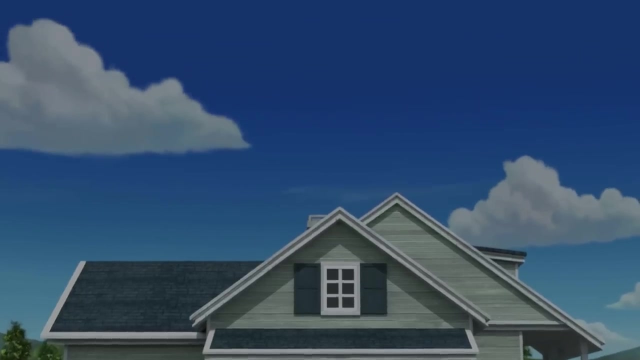 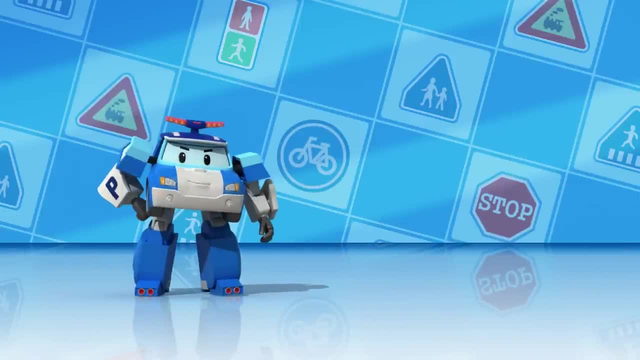 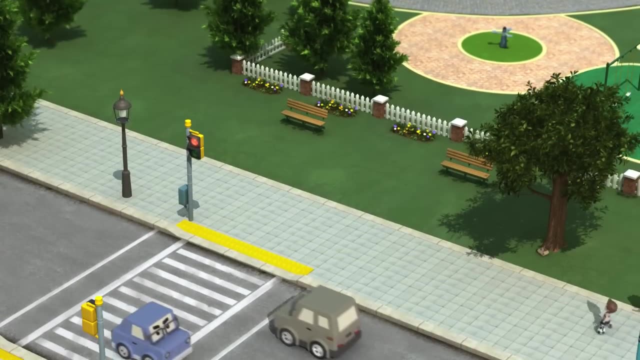 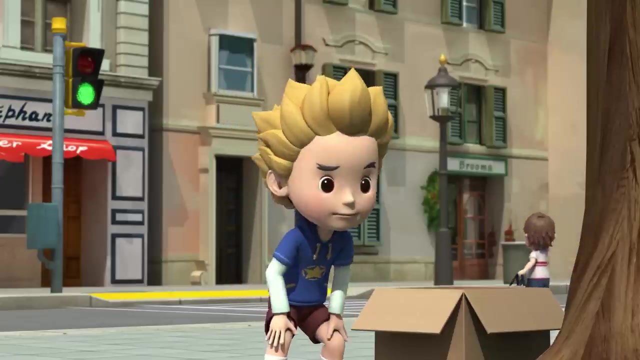 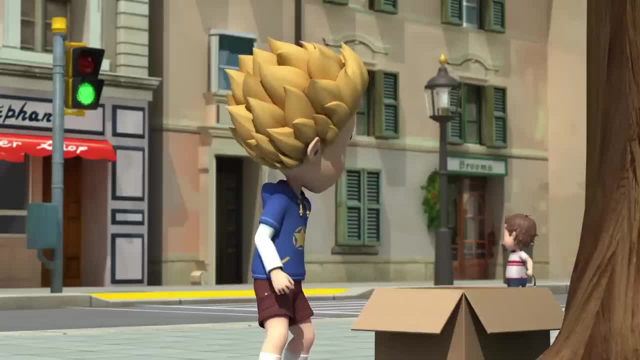 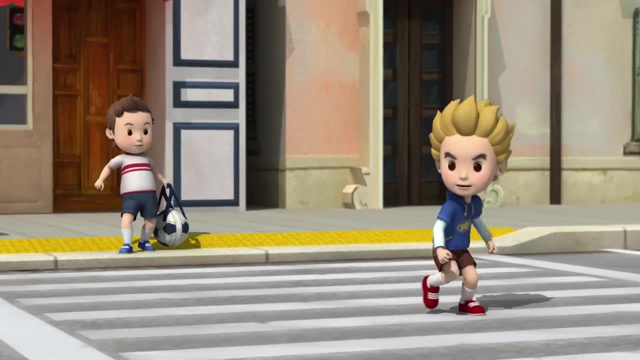 Ah, Ah, Oh, it's reallyils me. I'll go get these 300 bills for a new home And encourage them to sleep soundly. Why don't you stand up for TV for a minute? Okay, loves it, Enjoy. 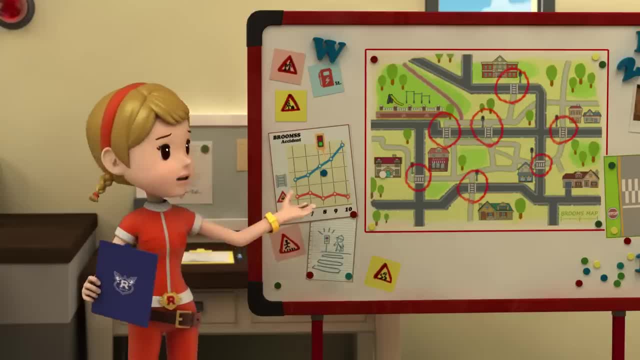 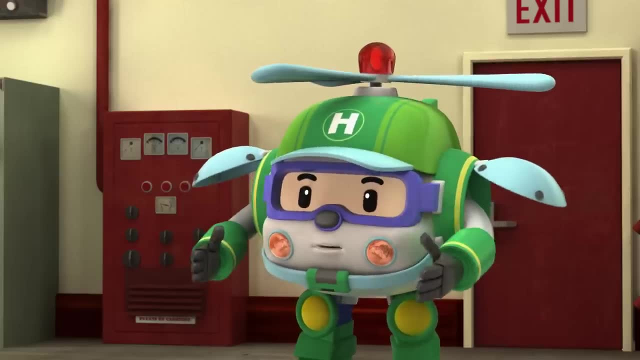 Time to switch up TV, Chicken. There's a growing number of accidents recently with children at crosswalks. What do you think we should do? I'll go and double check that all the green lights are working properly. Good, Amber, let's go together. 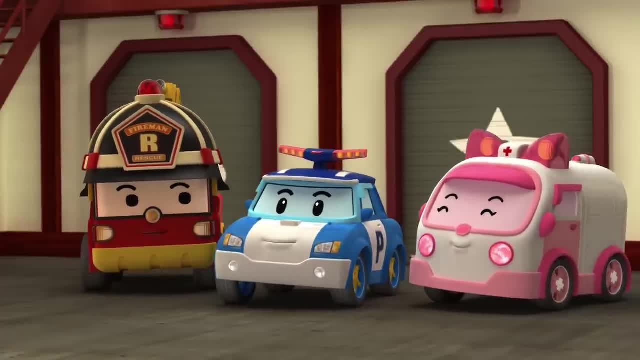 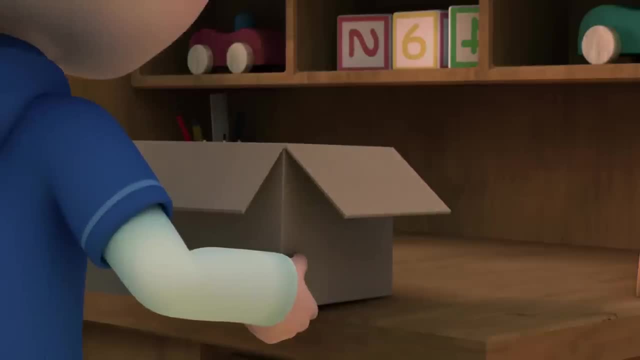 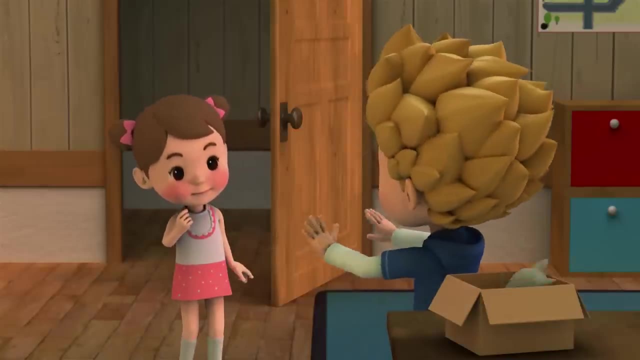 We'll go out to the crosswalks and guide the children as they cross the street Soft Like a ninja. There, Kevin Mommy says: come to supper There. All right, What's that? It's nothing, A cat. It's so cute. 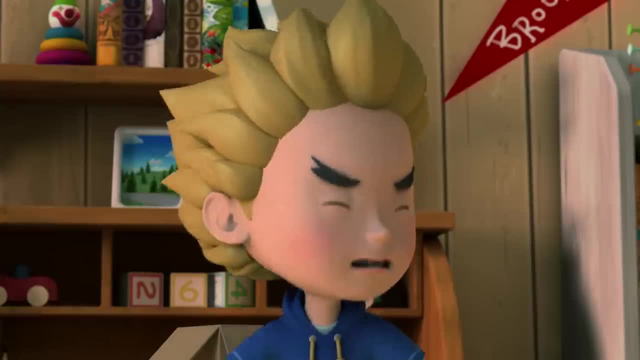 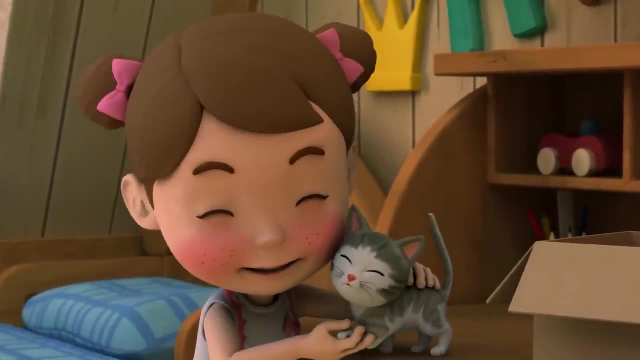 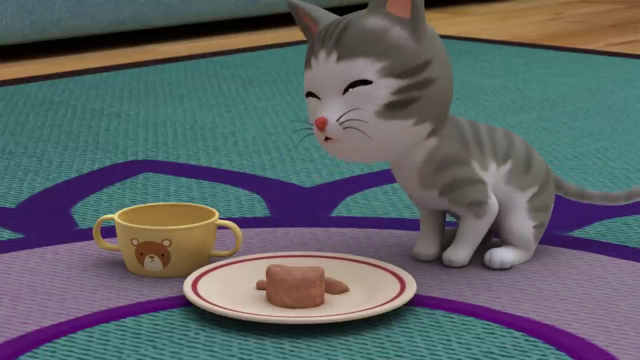 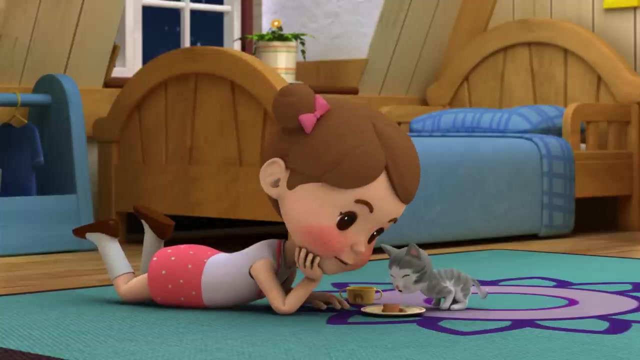 Shhh, Mom cannot find out. Kevin, Suzy, Okay, we're coming. Suzy Precious, Thanks for dinner. Thanks, Mommy, Go on and eat. Elizabeth- Elizabeth is not her name. Hey, Elizabeth, Aren't you adorable? 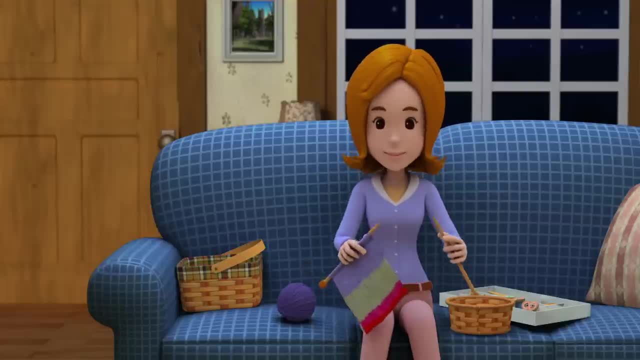 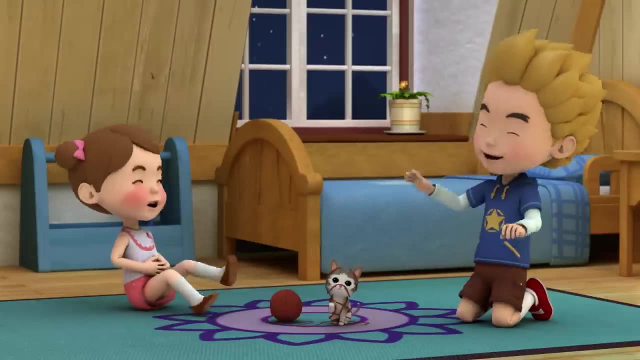 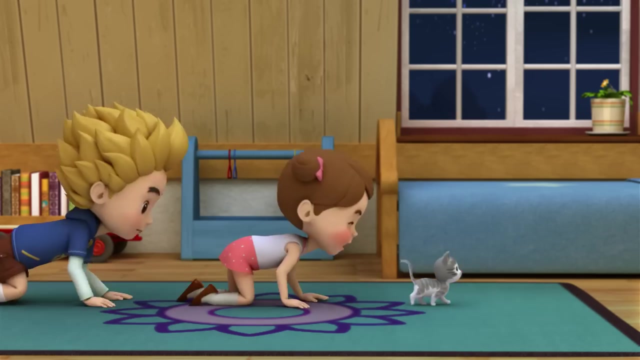 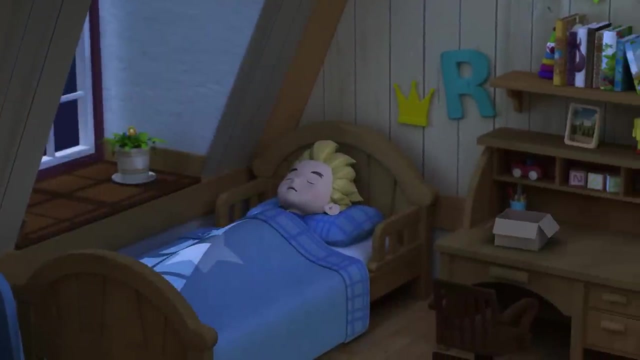 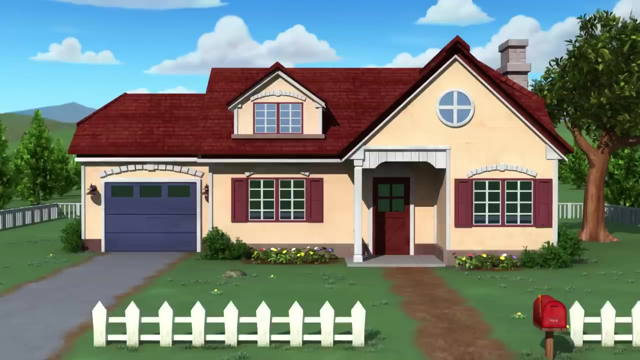 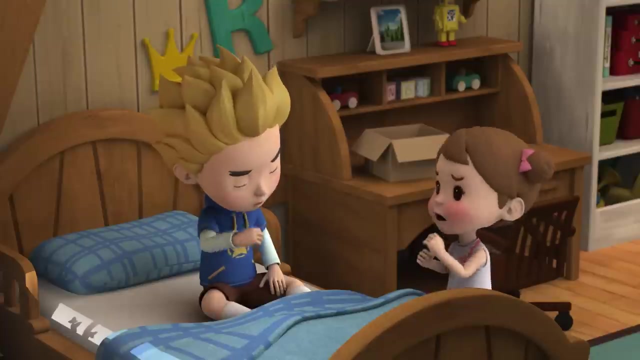 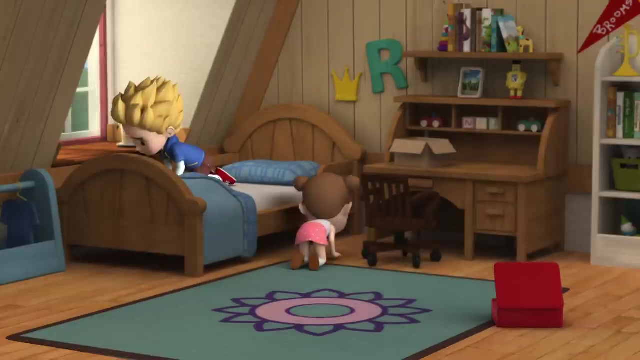 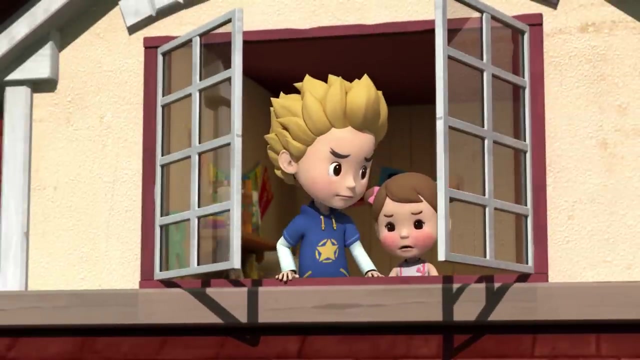 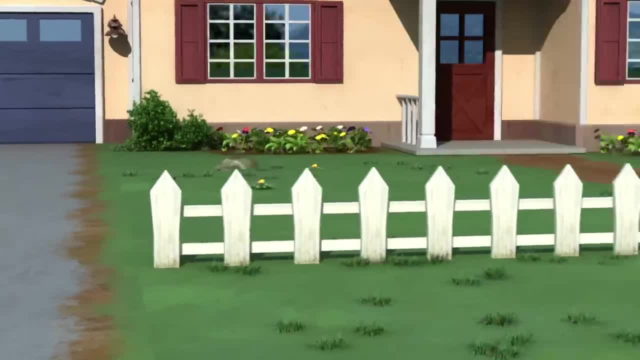 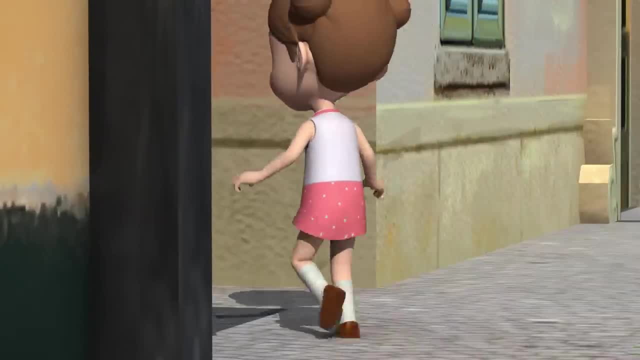 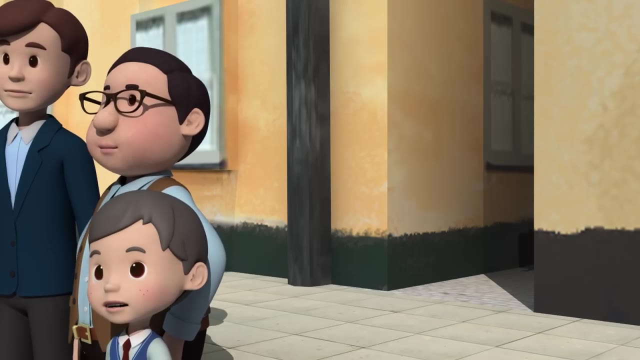 Huh, Come back. Hey, Susie, wait Elizabeth. Huh, Wait for me, Amber, let's see how things look at the 7th Street crosswalk. Sure, Huh, Okay, let's go, Susie. 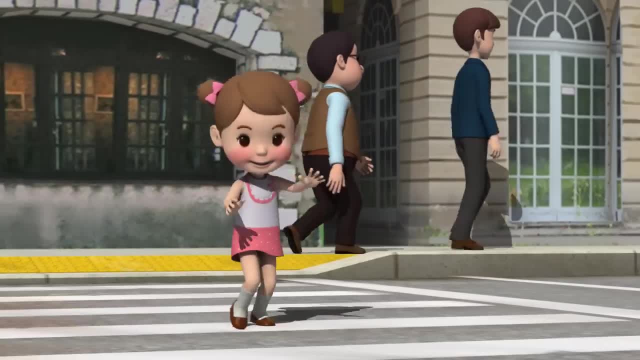 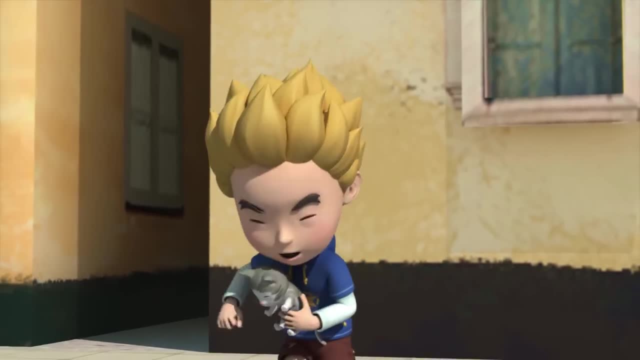 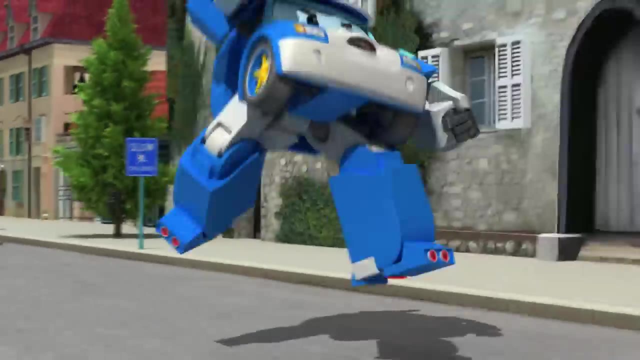 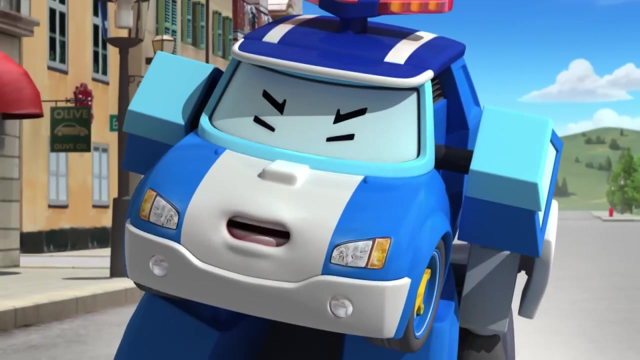 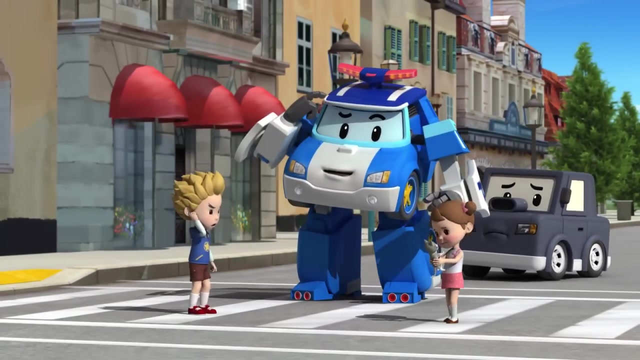 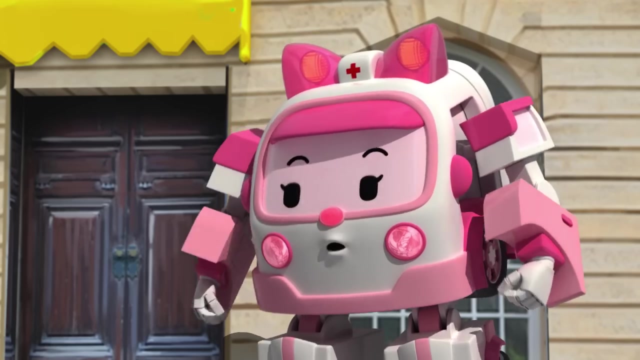 Huh, I found her, Elizabeth, Out of my way. No, Susie, Look out, Look out, Watch out. No, Elizabeth, That was dangerous. Susie, Thanks for saving us. Polly Susie, you have to learn that it's very, very dangerous to turn back when you're crossing the road. 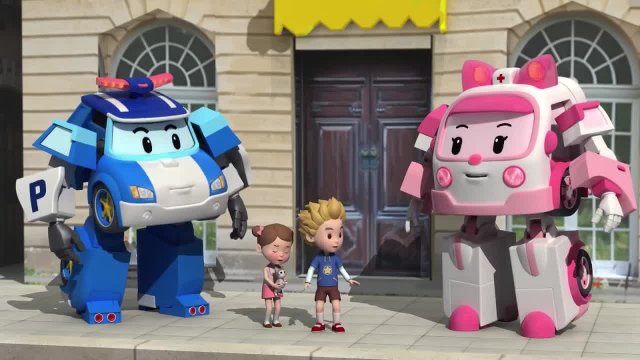 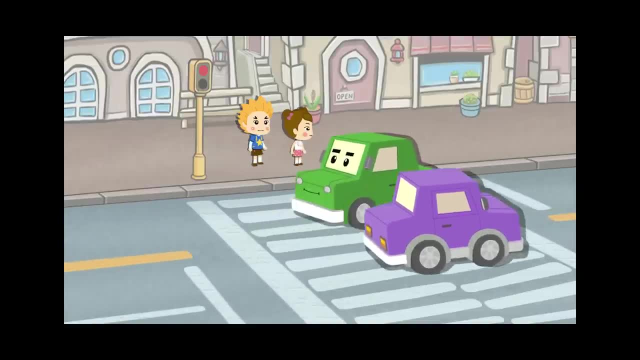 I didn't know. Okay, both of you pay attention and I will teach you the proper way of getting across a road safely. Are you both listening? Uh-huh, Uh-huh. You need to be very careful because there are a lot of cars driving on the road. 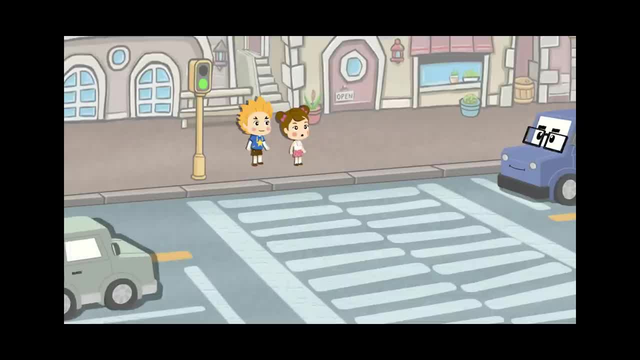 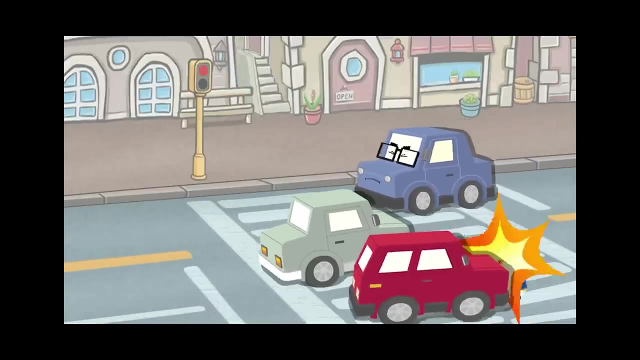 You must make sure all the cars are at a complete stop, even after the light says it's okay for you to walk. Once you cross the road you must not turn around, because cars might not see you coming back. When you have to go back, go all the way to the other side and wait for the next light. 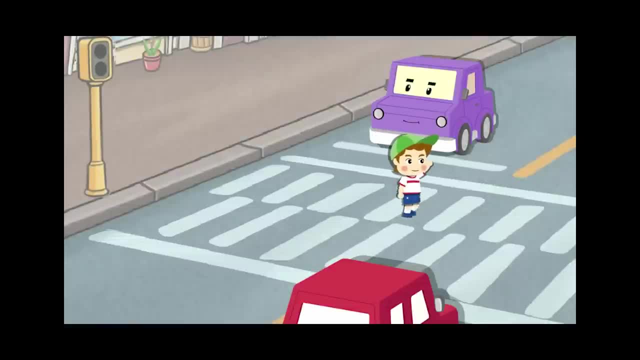 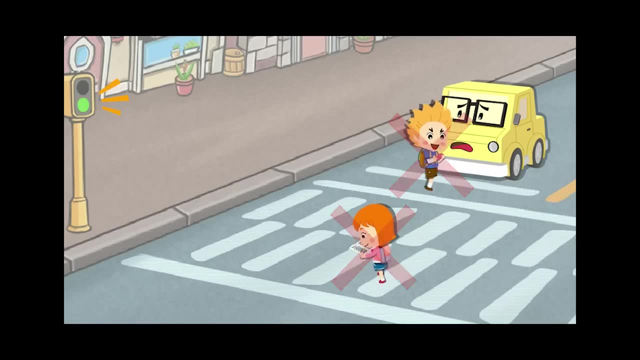 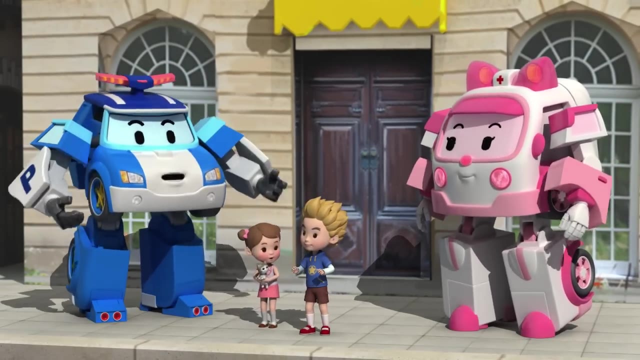 And while you're crossing the road, you should not pick things up from the ground, play games, read books or look anywhere but the street. Okay, And if the don't walk light is flashing, then it's a good idea to wait for the next light. 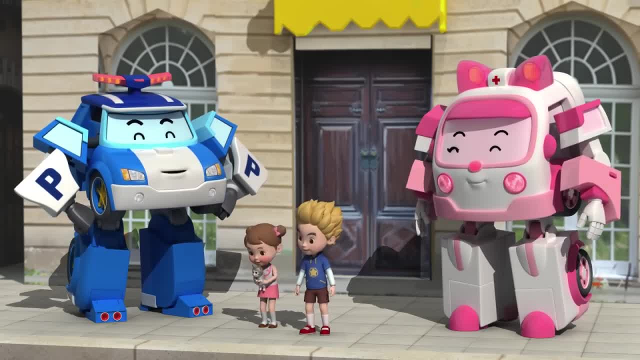 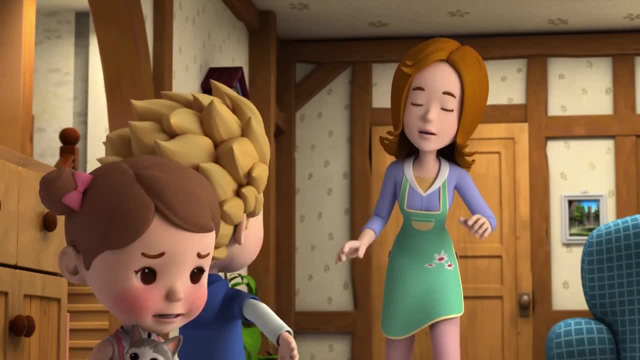 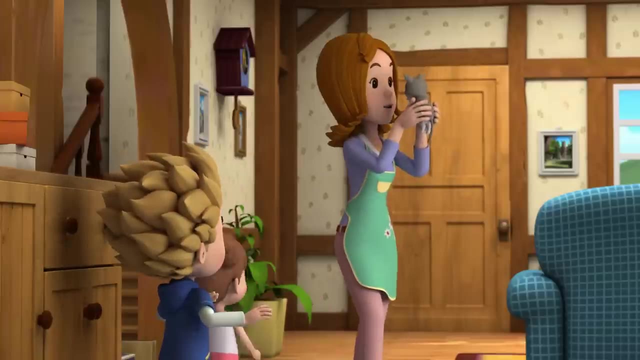 Okay, Polly, Okay, Polly, Quiet, Okay, where have the two of you been? Huh, What is that, Susie? Oh my goodness, It's a kitty. Oh, I'm gonna call you Mittens. Her name's Elizabeth. 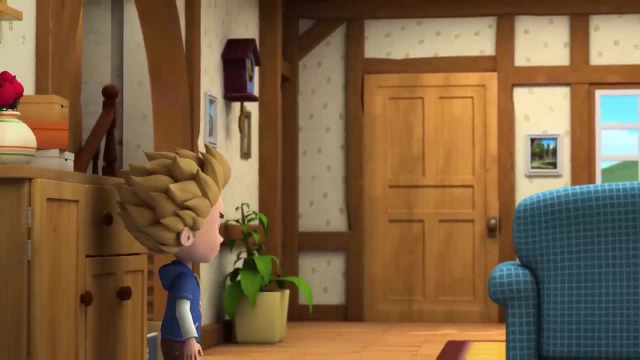 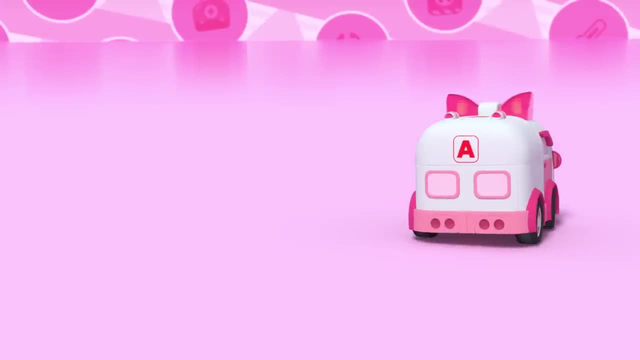 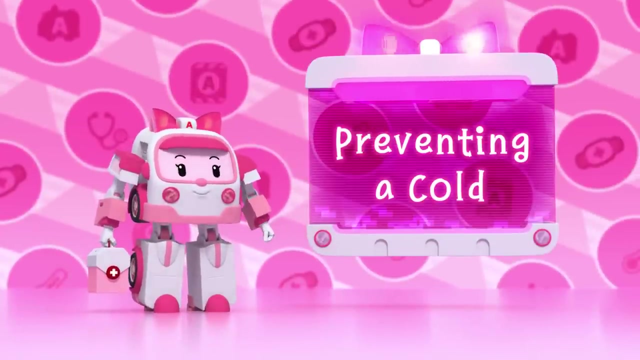 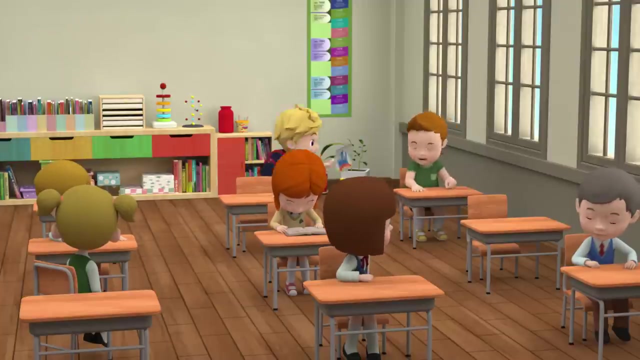 I like mittens. You can't change your name. Preventing a Cold. Johnny, look at this. What is it? Uh, where's Charles? He's out today because he has a cold. That's too bad. I'm going to Broomsland this weekend and I can't wait. 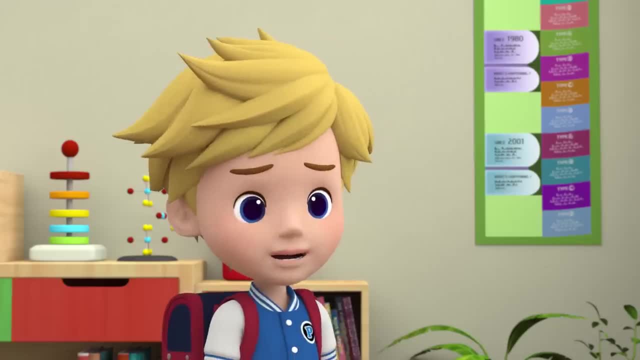 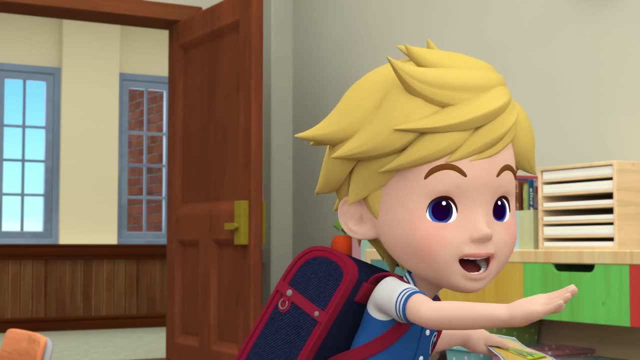 Broomsland. Yep, I'm going on the roller coaster and the bumper cars. Whoa Sounds great. Watch out, Johnny, That's so gross. Sorry, Peter. Ah-choo, Ah-choo, Ah-choo. 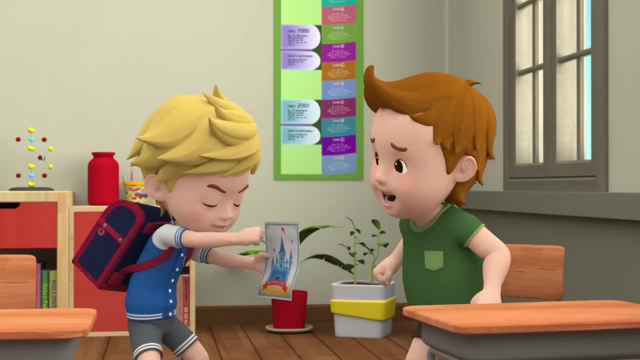 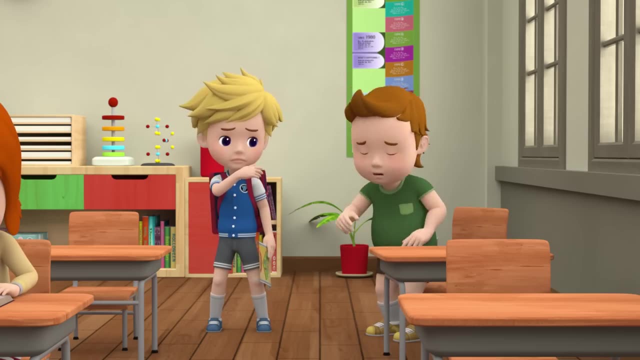 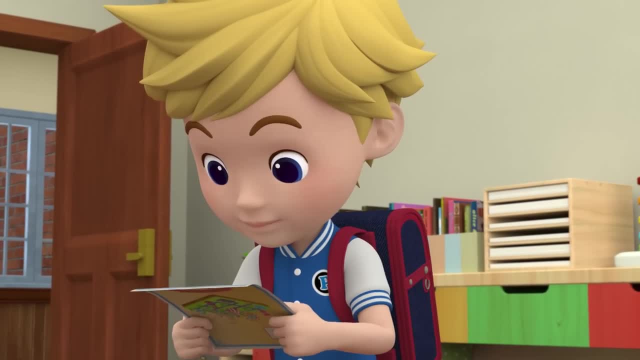 Ah-choo, Ah-choo, Ah-choo. Wait for this. What's up, Jin? Welcome back everyone. I love the pig mask. That's hilarious, Jin, do you not feel? well, Jin, are you getting a cold? 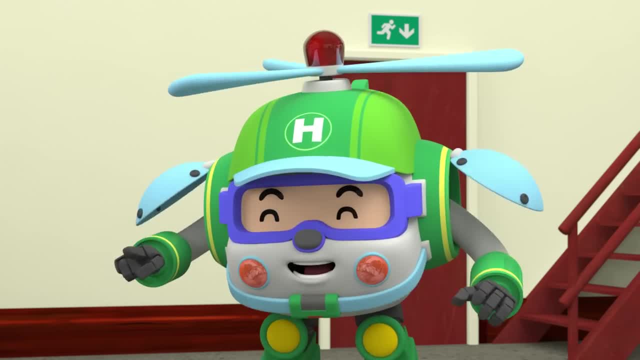 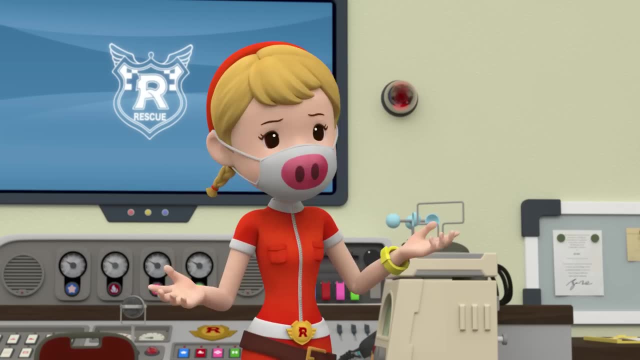 Ugh, There's some kind of bug going around Broomstown. In that case, it's good you're wearing that mask. It helps to cut down on the number of germs that get spread around the room. Oh, I see. 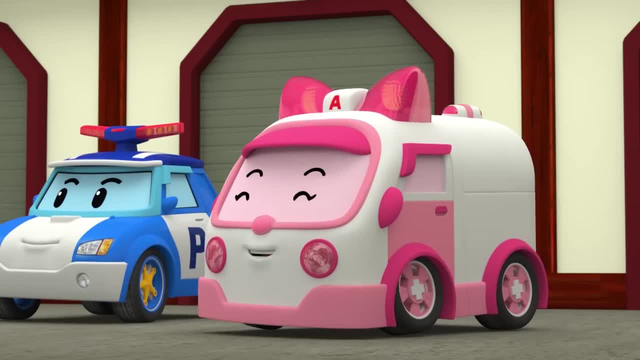 I'm glad you're not feeling well. I'm glad you're not feeling well. I mean, you can't be shivering or anything like that. I still have to go see a doctor. Well, I see, I'm glad you're not feeling well. 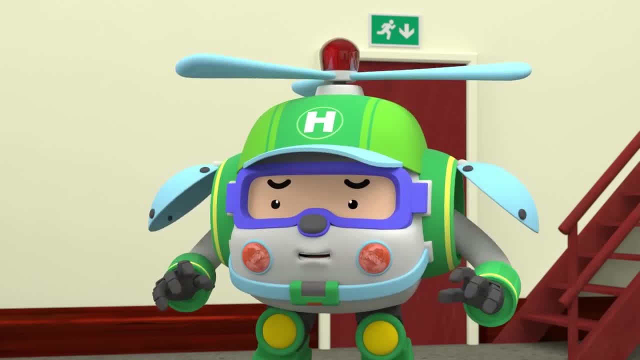 But there's some kind of bug going around the room. with this kind of bug Here, this makes sense. You might have some of the things that get spread around through the air. That makes sense. Good thing, because I've got one for you too. 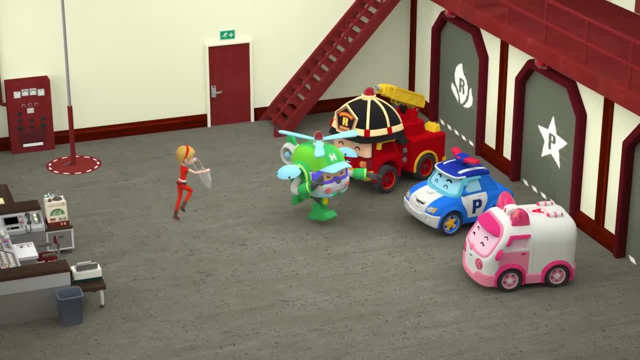 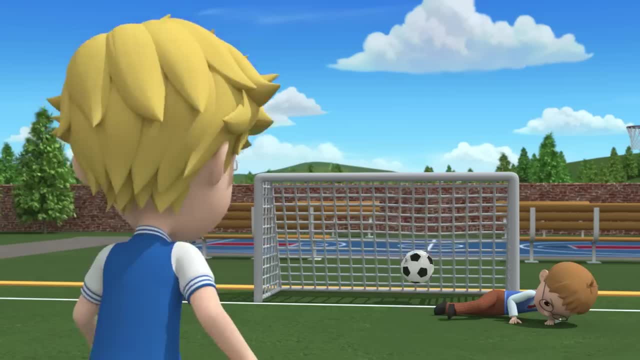 What? No, thanks, I'm feeling fine. Oh, come on, Get it away from me. No, I don't need it. No, Just try it on, Heli, You'll look so cute. Take it, Peter. 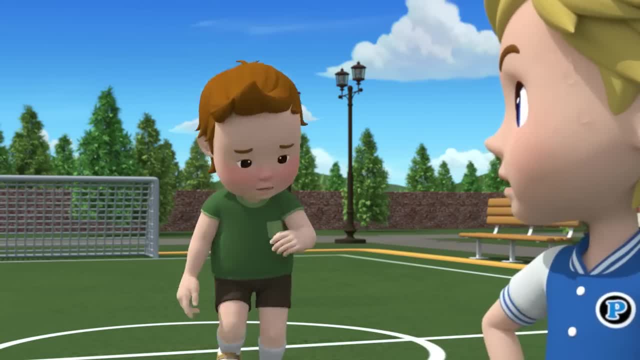 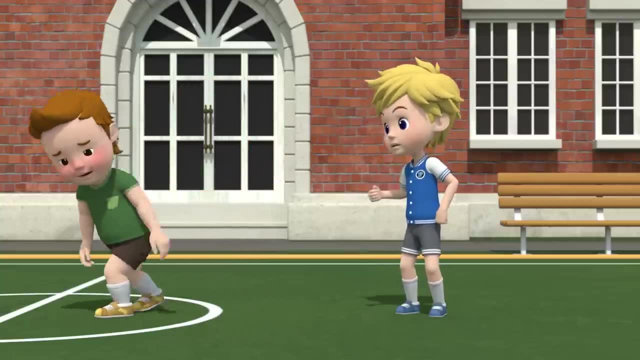 Nice pass Andgoal. Alright, Johnny, I scored. Peter, I think I need to go home and lie down, and lie down. Come on, you're tired already. Yeah huh, See you later, Johnny, you're so out of shape. 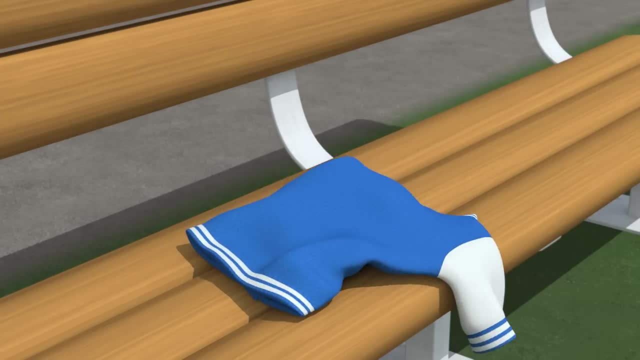 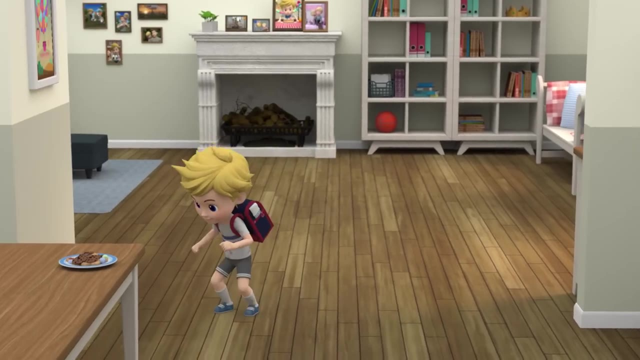 Peter, come on, man. Yeah, all right, Let's get this half started, right, Mom, I'm home. Yes, I see that. Nice work, Mom, These look great. Not so fast. You need to wash these hands first. 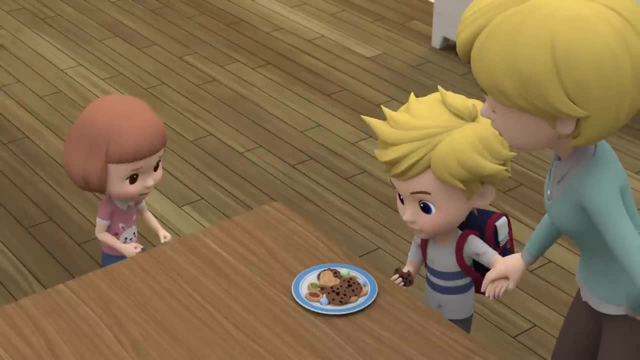 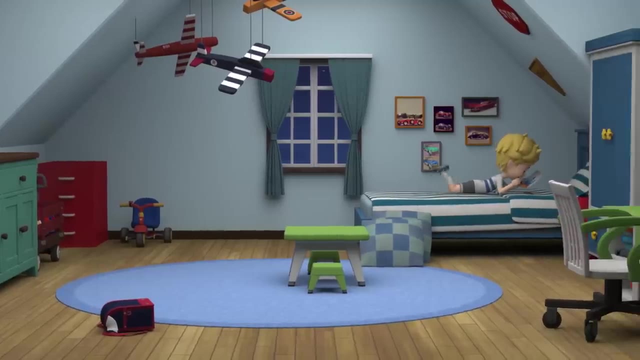 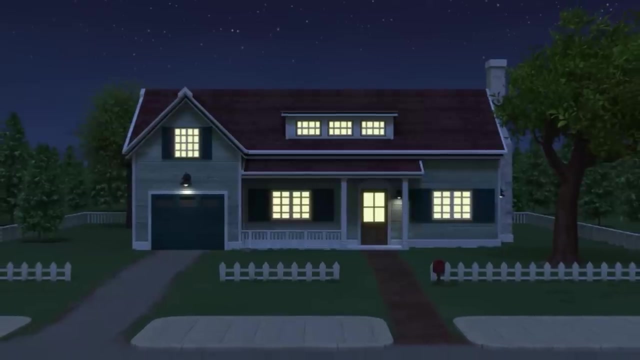 I'll do it later, Peter. Mom and I made those to take to Broom's Land tomorrow. I'll only eat a few. Ha, Peter, We'll do the petting zoo and the fireworks. Ah-choo Tomorrow, can't get here soon enough. 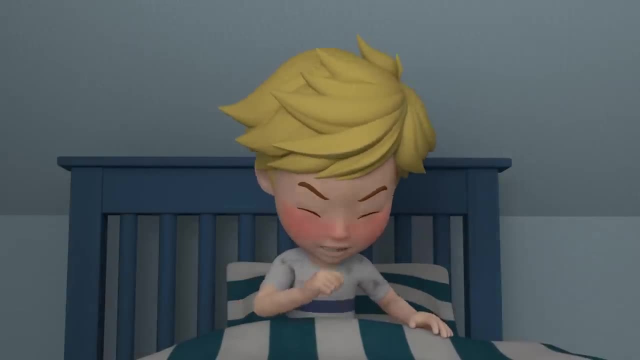 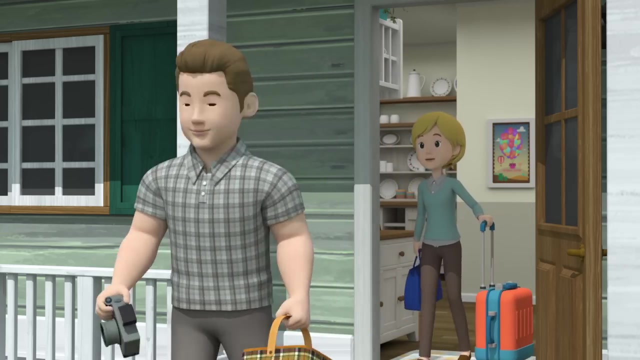 Finally, I can't wait to go. Woo-hoo, I can't believe we finally get to go, And we couldn't have asked for a better day. Robert, you packed everything. I've packed the lunchbox and I've got the camera. 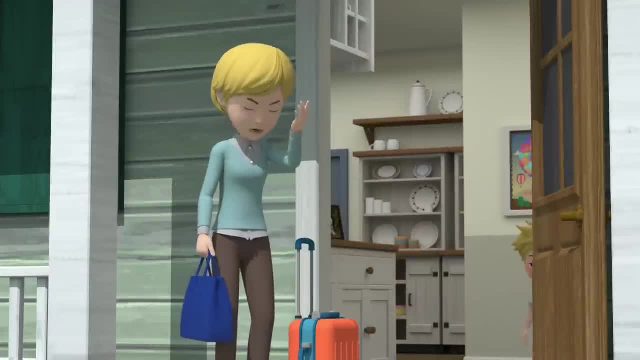 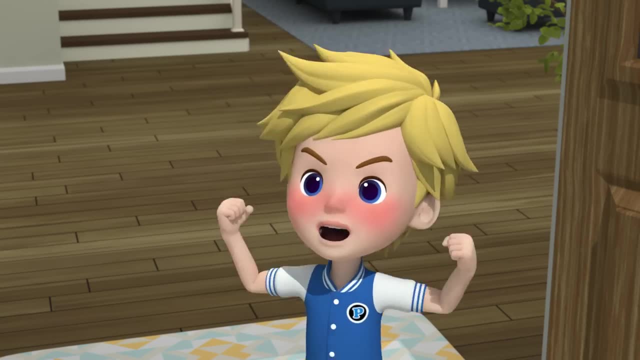 And the mat. Uh-oh, I'll be right back, sweetheart, Every single time. Huh, Peter, do you have a cold? Huh, Uh, no, I'm better than ever, Really, Yeah for sure. 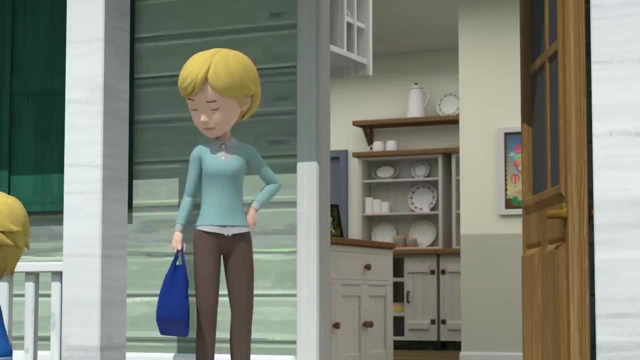 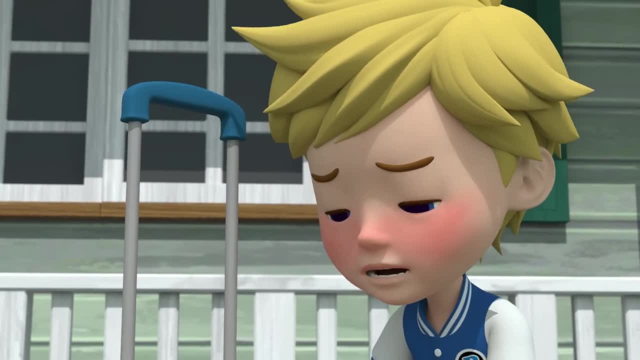 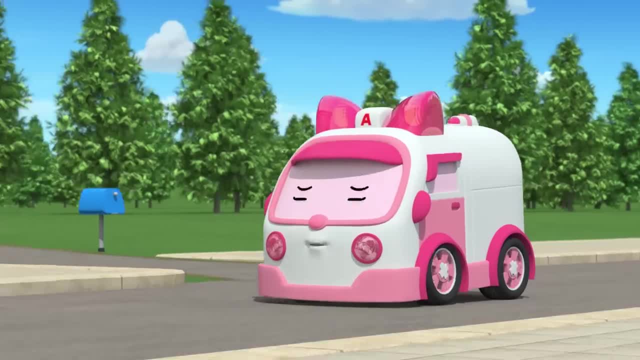 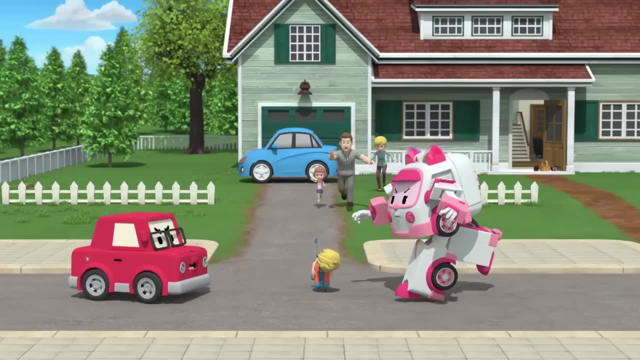 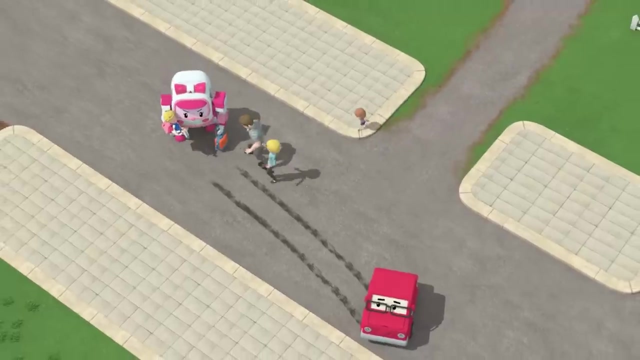 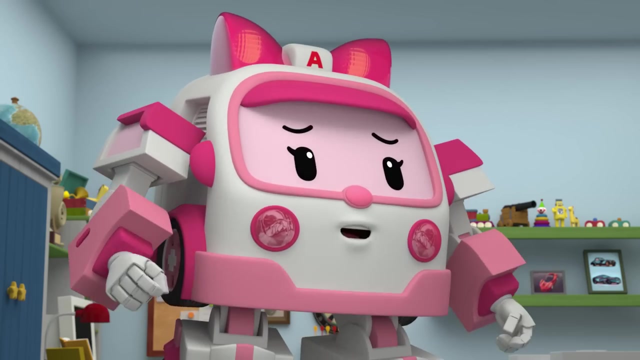 Peter, Huh, Somebody help Peter. Huh Ugh, What's happening? Oh no, Watch out, Ugh Ugh, Peter. Peter, He's got a nasty cold. I gave him some medicine for the fever. 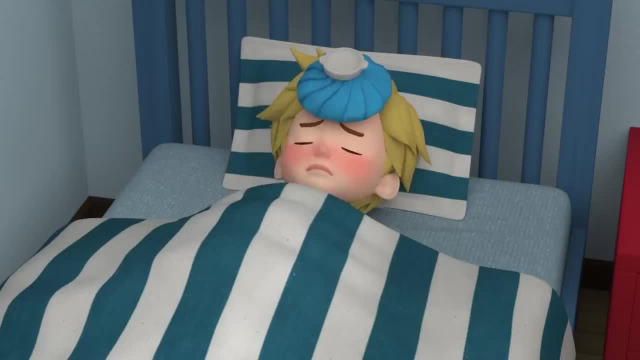 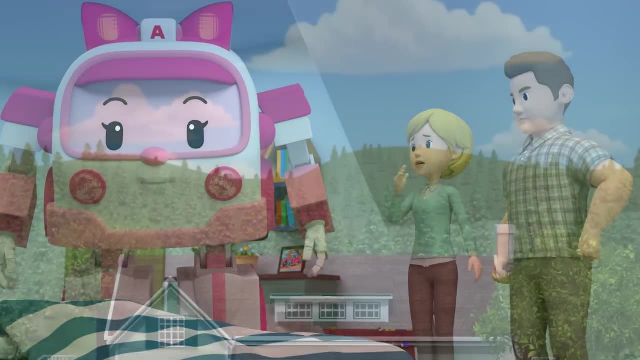 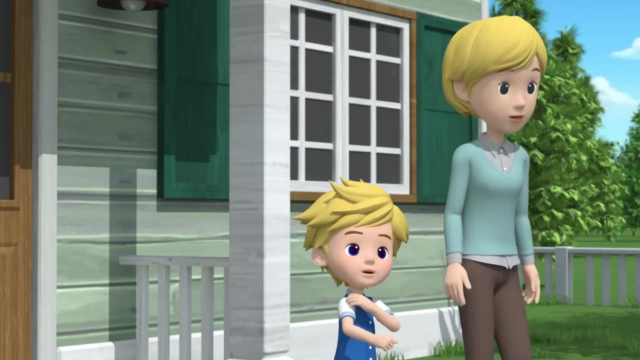 Thank you, Amber. Thank you, Amber. Oh, Broom's land, Broom's land. Just let him rest a few days until he's better. Okay, It feels so good to be outside. Good morning, Hello Peter. 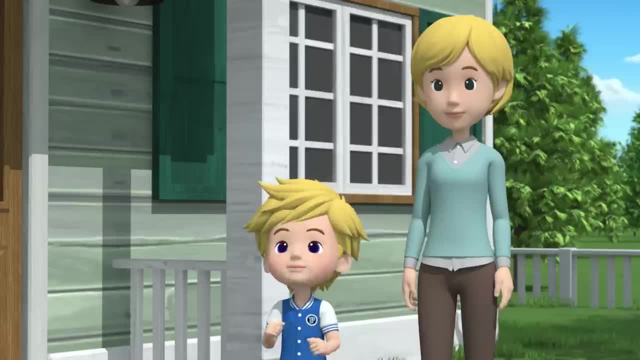 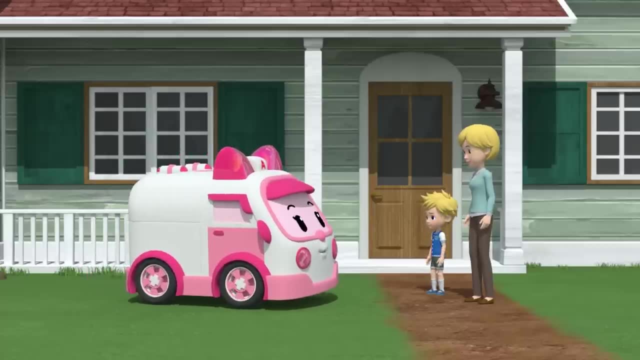 Hello Amber. Hello Amber, So how are you feeling After sleeping? like you said, I feel much better. I don't want to be sick ever again. You can help prevent colds by doing a few simple things, Really. 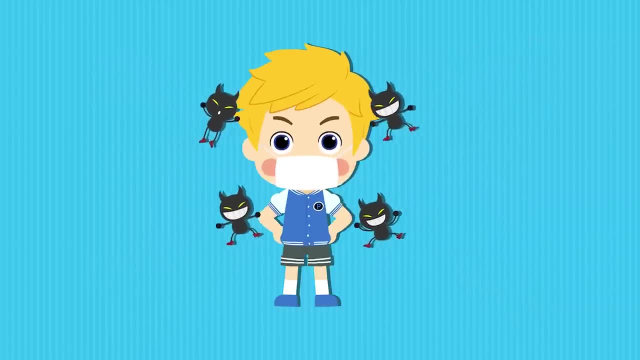 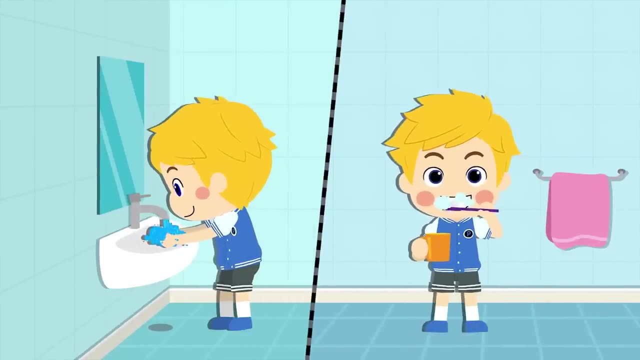 If there's a cold going around, it's a good idea to wear a mask to keep the virus from spreading. Washing your hands often and brushing your teeth will help eliminate any germs you may have come into contact with If you're not dressed for the weather. your immune system can weaken. be sure to wear a mask. Be sure to dress warmly on cold days. If you cough or sneeze into your hands, you'll spread the virus to anything you touch. Cover your mouth with the inside of your elbow or a tissue. 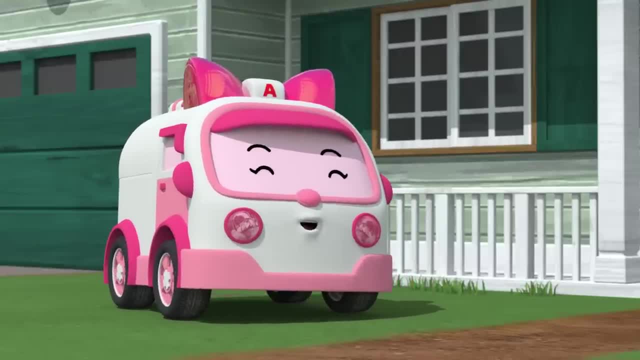 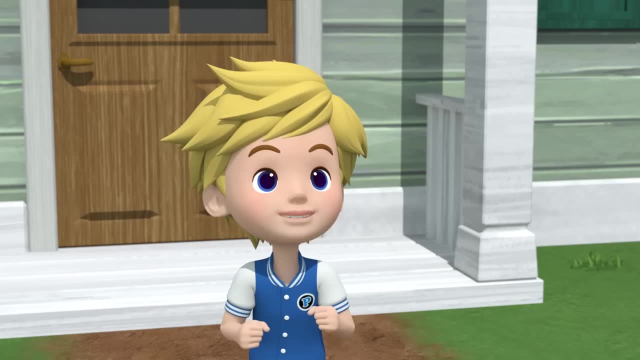 If you do catch a cold, get lots of rest and drink plenty of fluid. Understand, Yes, Amber. Hey Mom, can we go to Broom's land right now? You're sure you're well, Way sure, I'm 100%. 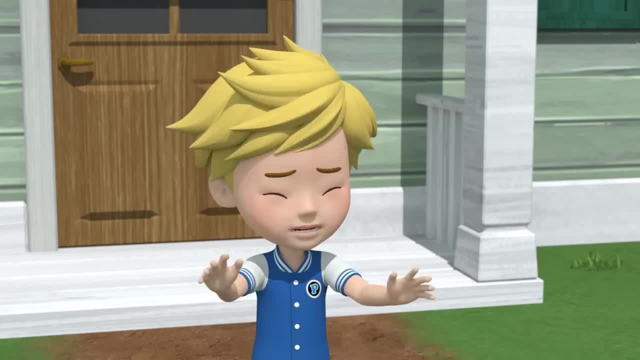 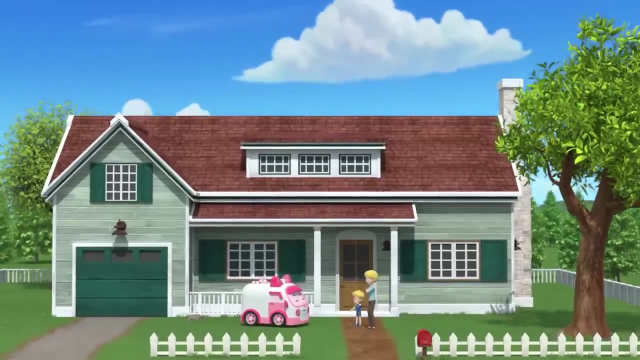 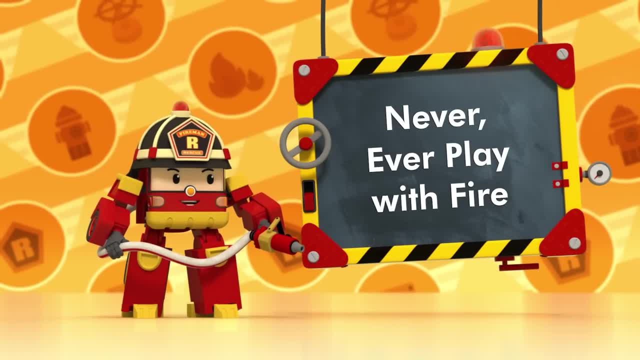 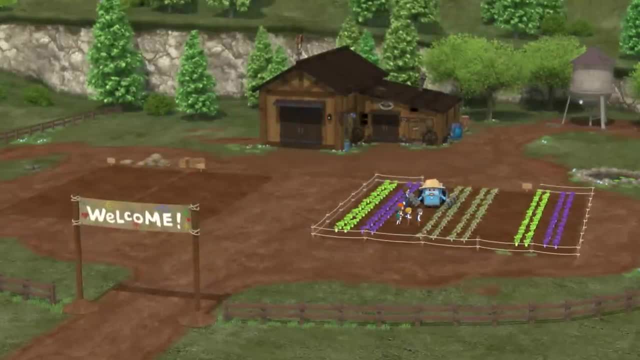 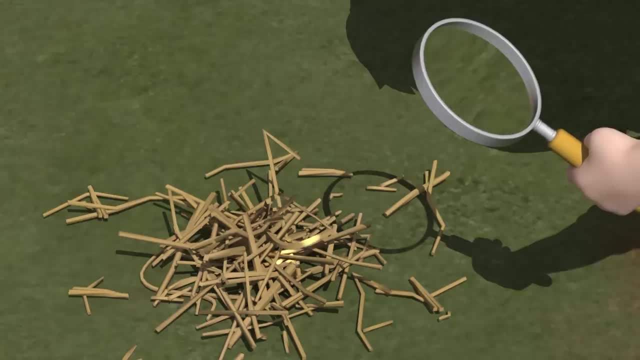 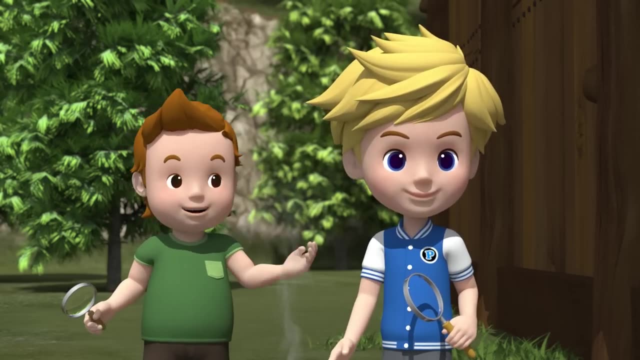 Wow, Huh, Huh, Huh. What are they up to over there? And if I do this, What's going on? You scared me, Charles, come here and check this out. Peter's burning stuff with his magnifying glass. 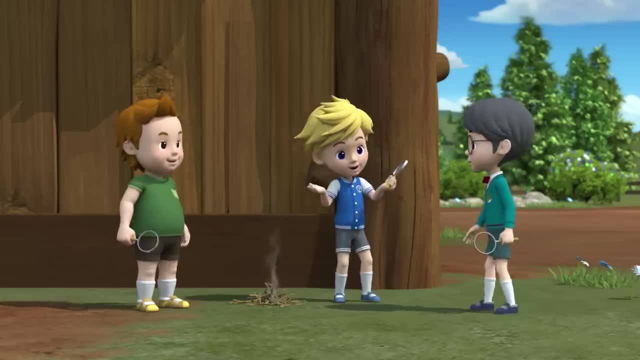 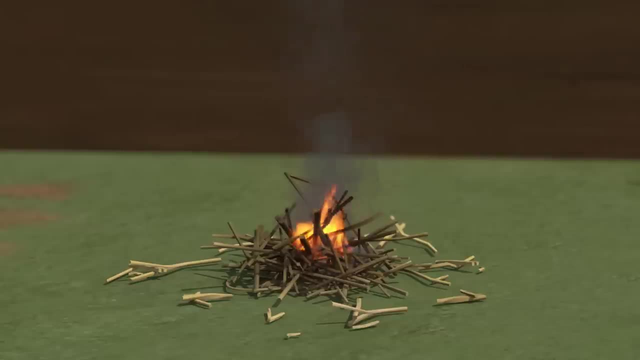 Huh, Peter, you should never play with fire. But it isn't playing. Yeah, It's a science experiment about harnessing the sun's power. Look It worked. Oh, Whoa, Isn't that fire too big? Oh, 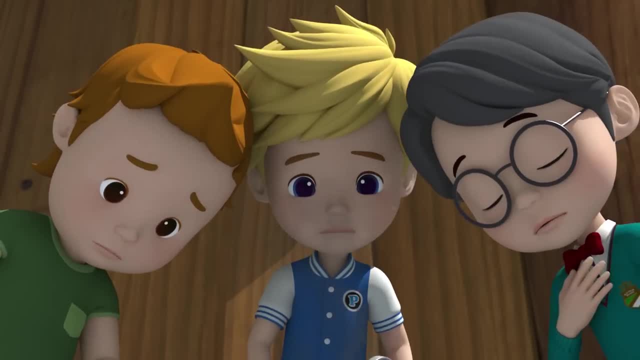 Oh, Oh, Oh, Oh, Oh, Oh, Phew, Phew. OK, students Gather up, Huh, Huh, Huh. Right, Come on. Huh, Huh, Huh Huh. 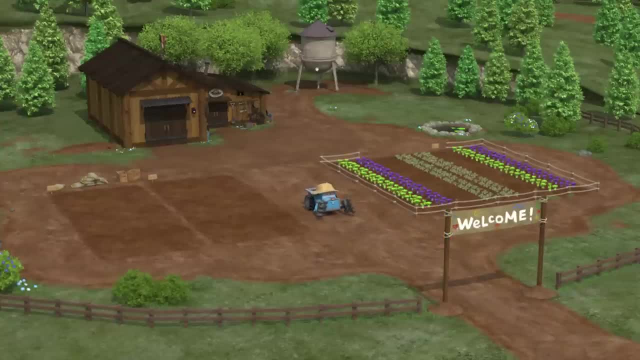 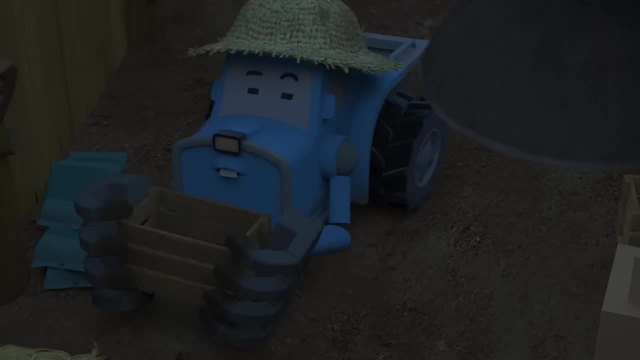 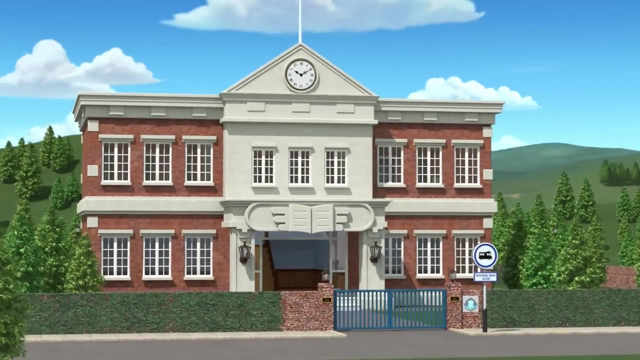 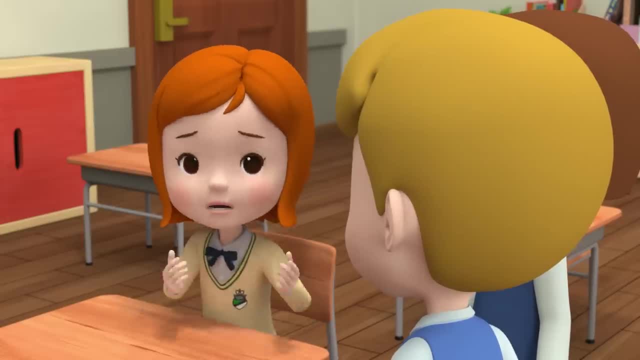 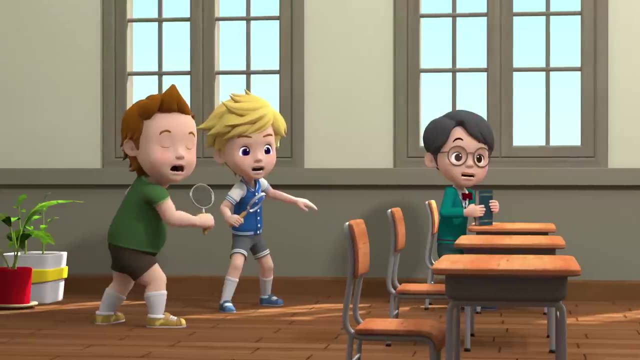 Trachy's house caught on fire For real. Huh Goodness, What happened? Huh, We had to call in the rescue team and everything. It was pretty bad, Oh dear. Is Trachy going to be OK? 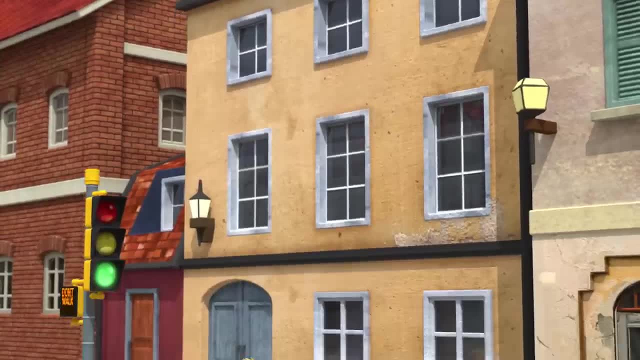 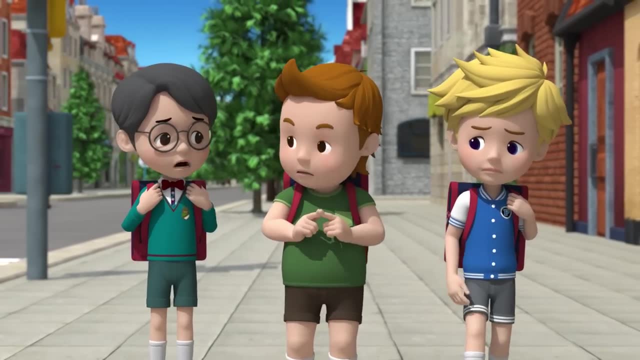 Huh, Huh, Huh Huh. Do you think we caused the fire at Trachy's? It's weird. Our little fire was out for sure. Listen, guys. We need to be honest and tell the teacher about the fire. 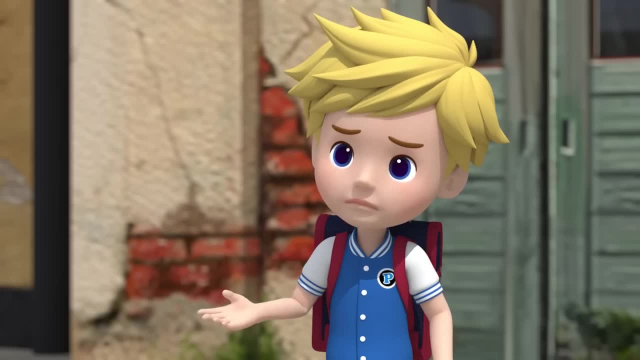 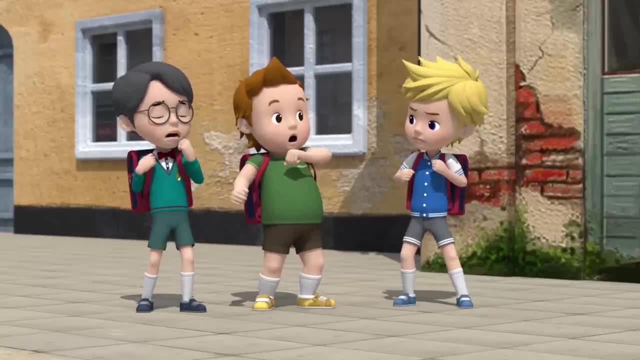 What, What, Charles, are you kidding? If we tell the teacher, then all our families will find out, And then they'll tell the rescue team. Oh, Then we'll end up in jail, or worse. Oh no Huh. 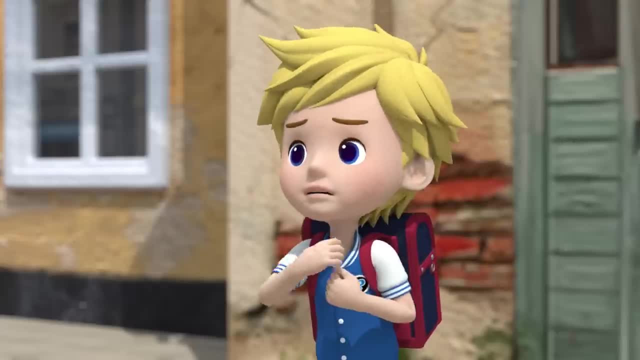 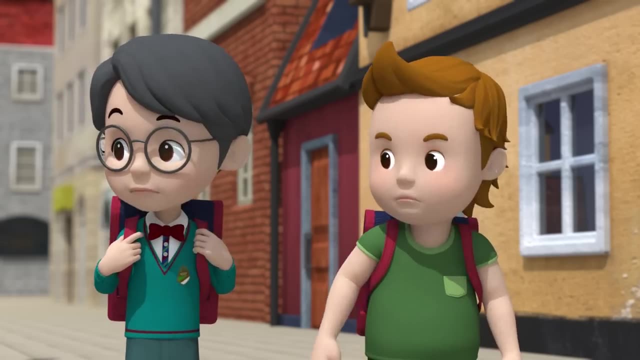 Jail. I can't go to prison. So the whole thing about what we did at Trachy's will be our secret and we'll never tell. Um, but, Kleene, did you hear? Huh, There was a bad fire out at Trachy's place. 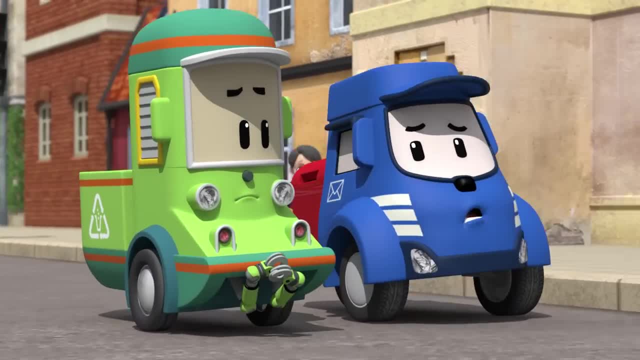 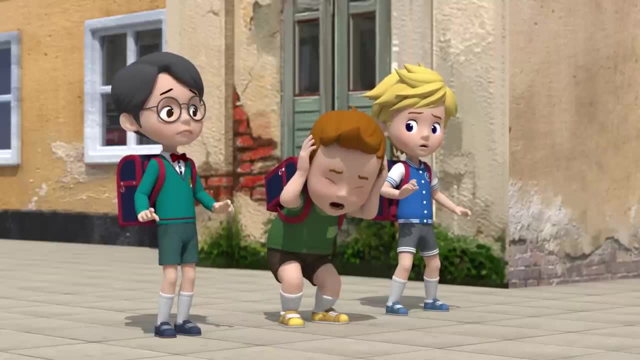 And Trachy got hurt Really. And was he hurt bad? Well, he's lying in bed wrapped in bandages. Huh, I'm sorry, but I have to confess what we've done, What No way You promised you wouldn't tell, remember? 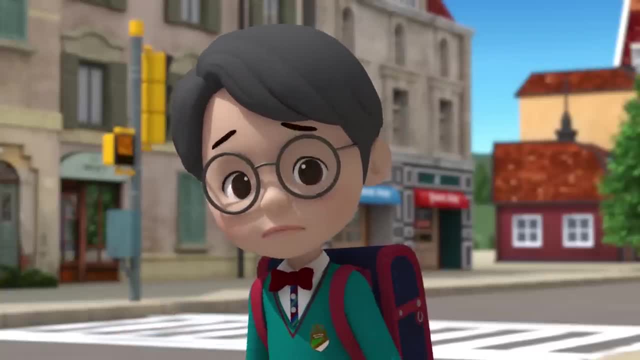 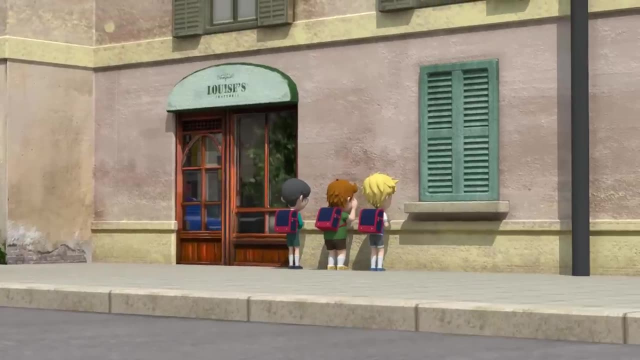 I'm with Johnny Trachy got hurt And it's all because of us. Guys, please don't tell: Huh, Huh, Ugh, Phew, Then it's settled. No one says a word, right? 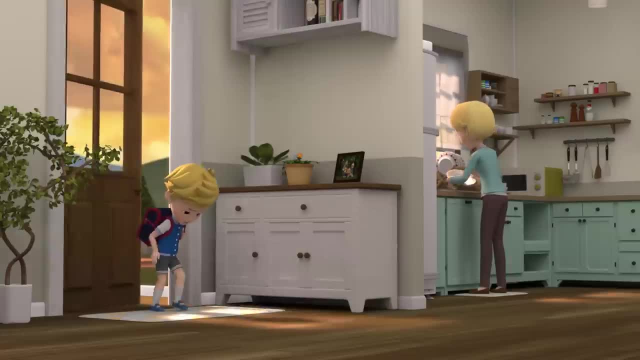 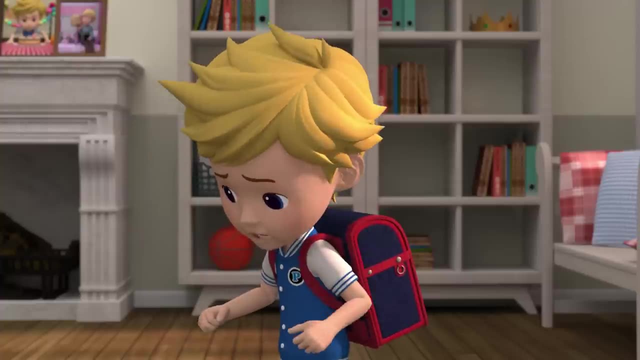 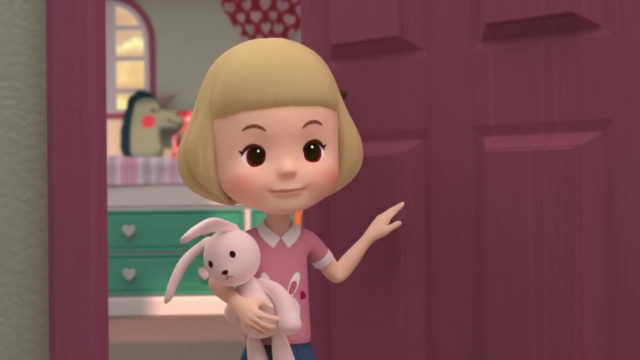 Uh-huh, I'm back. Hi, Peter, Did you hear There was a fire at Trachy's Mom? I'm tired, I'm going to bed. I wonder what's bothering him. Huh, Uh, Peter, you dropped this on the floor. 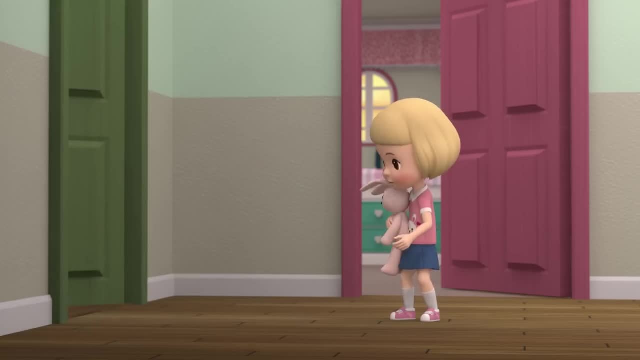 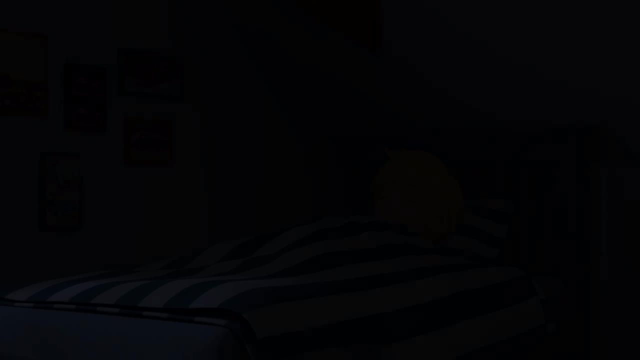 Huh, Ah, Give it here. Ugh, Huh, Hmm, Hmm, Huh, Huh, Oh, Peter, Huh, I'm so disappointed that you caused the fire, Cindy, I didn't. You set Trachy's house on fire. 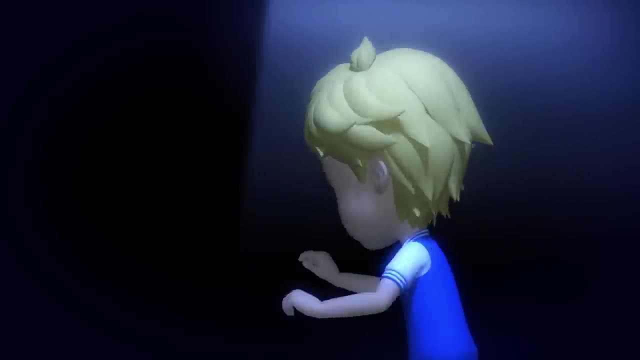 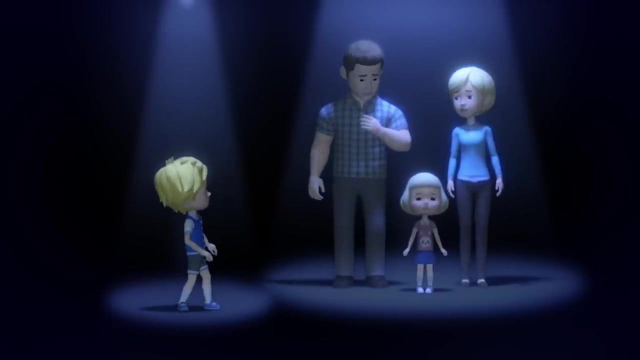 Huh, Huh, No, No. I never knew our son was lying in bed wrapped in bandages. What, No, No, No, No. I never knew our son was like that. Dad, Oh, Mom, It isn't true. 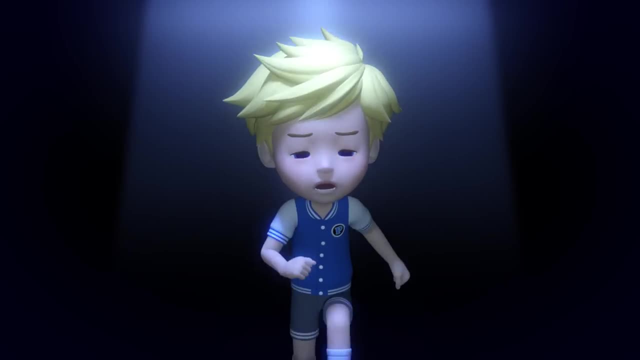 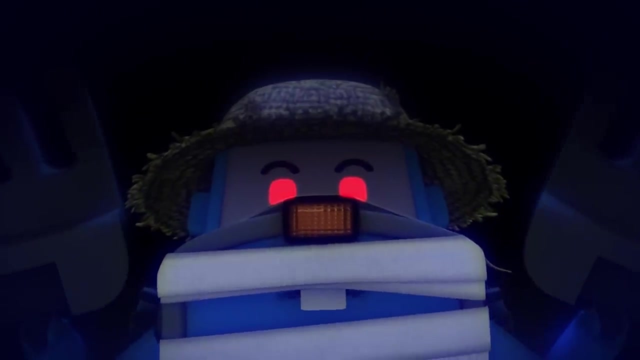 Peter. Huh, Johnny Charles, Why are you in there? Oh, Oh, Oh, Oh, Peter, How could you have done this to good old Trachy? Look what you did, Trachy, I'm sorry.